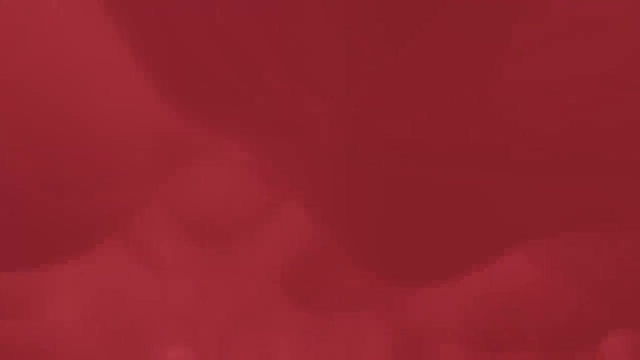 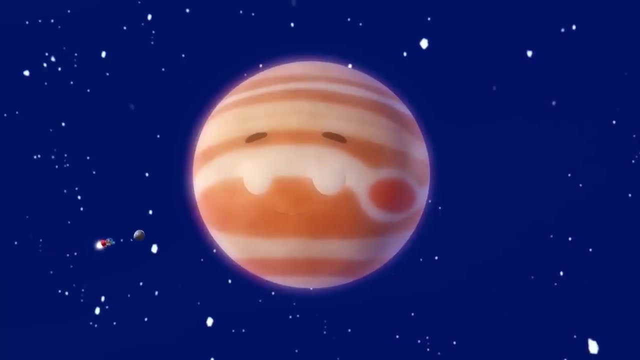 Mars is red because it's covered in rusty soil. Ah-choo, That's a lot of dust. Come on. Next up is the giant Jupiter, bigger than all the planets combined. bigger than all the planets combined. He doesn't scare me, though. 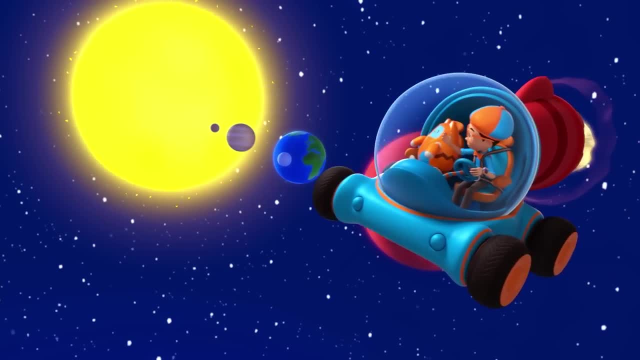 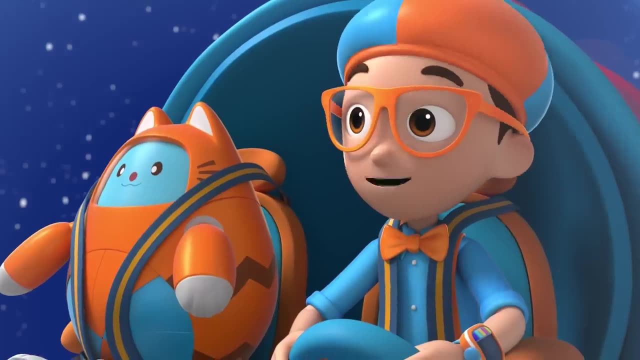 Whoa, We should go. We sure are a long way from the sun now. We sure are a long way from the sun now. Welcome to Saturn and her rings. Welcome to Saturn and her rings. Whoa, They look beautiful. Can we get closer? 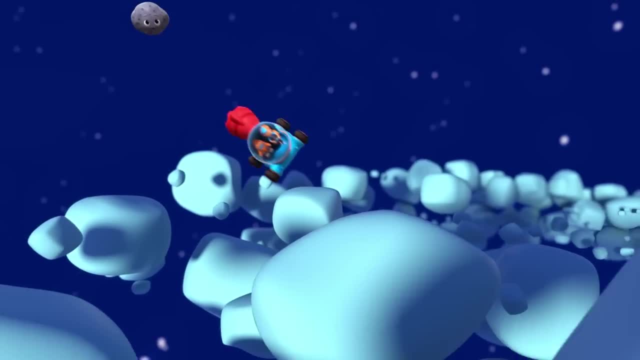 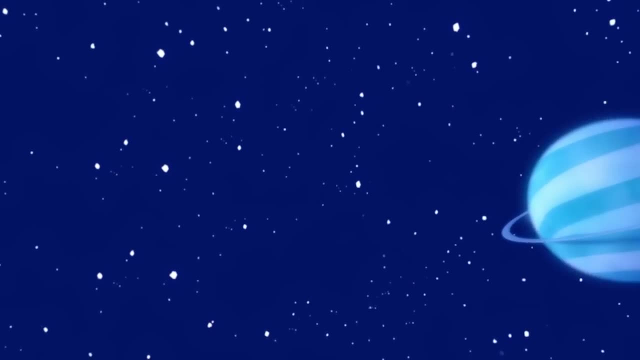 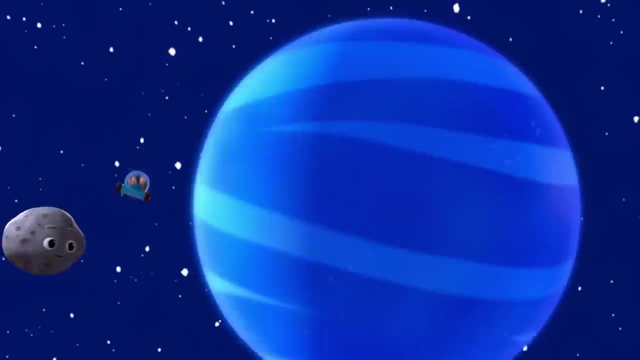 Of course, Whoa, Whoa, Yeah Wee. We haven't finished yet. On your left is Uranus. On your left is Uranus: billions of miles from the sun, pretty cold. billions of miles from the sun, pretty cold. Now let's hear it for the furthest, windiest and coldest planet: Neptune. Whoa, I have the answer to my question: What planets are in our solar system. What planets are in our solar system? Mercury, Venus, Earth, Mars. 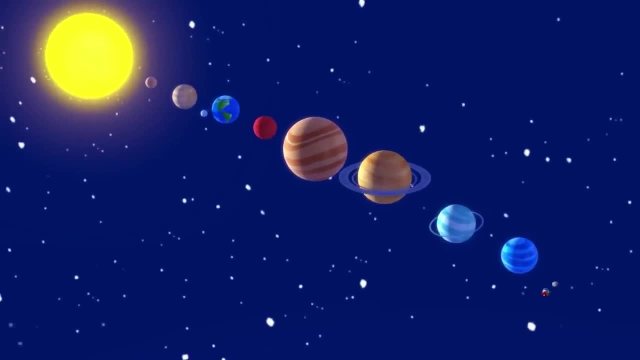 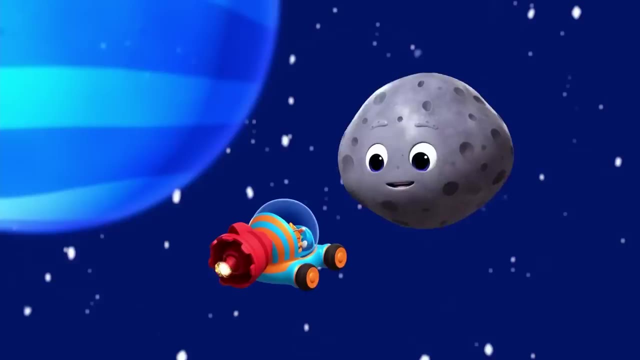 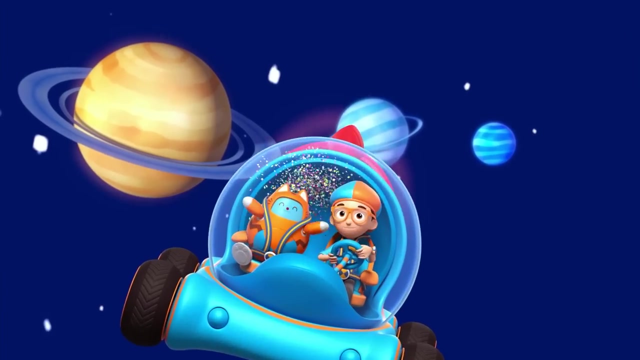 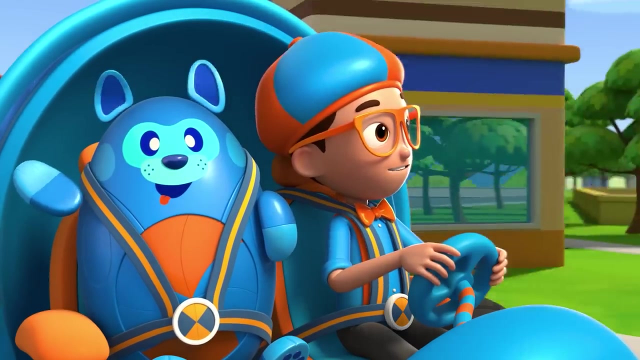 Jupiter, Saturn, Uranus and Neptune. Upload answer tabs. Thanks for the tour, Mary. That was wild. See ya Blippi. Time for a shower, A meteor shower. Bye, Mary the meteor. What a nice day for a quiet drive. 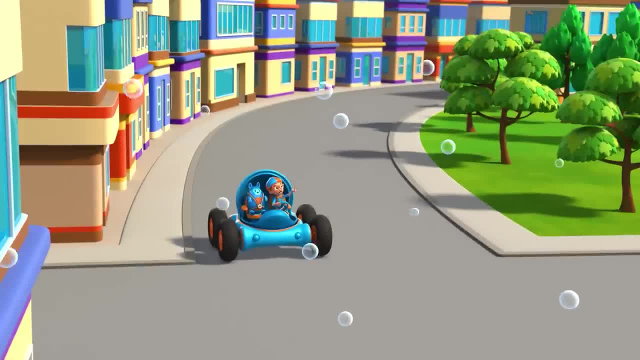 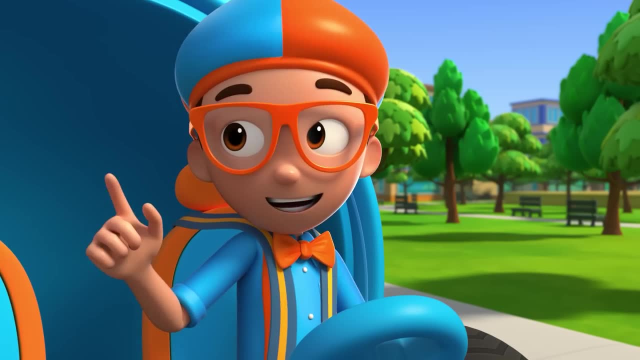 Whoa. Attack of the bubbles. Attack of the bubbles. Attack of the bubbles. That's right, Deebo. Bubbles pop when you touch them. I wonder, how do you make bubbles? I wonder, how do you make bubbles? 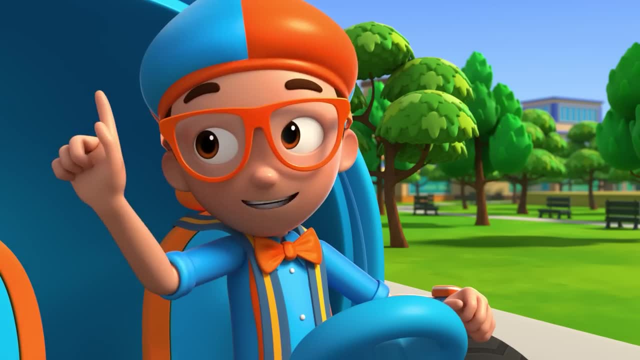 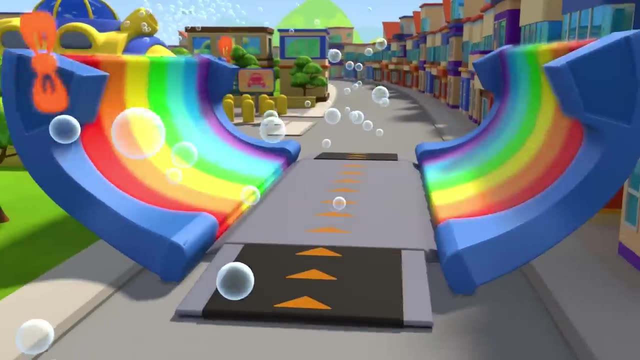 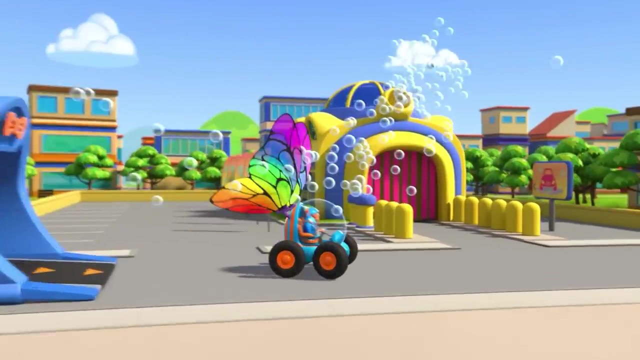 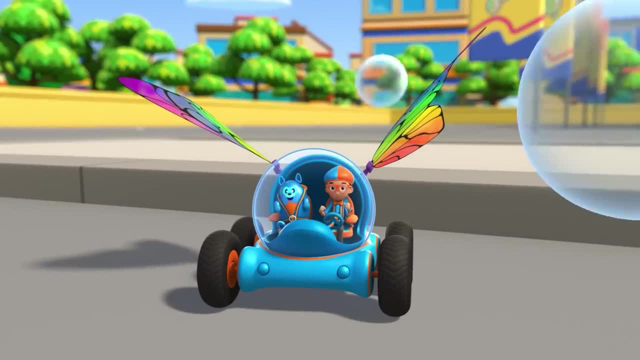 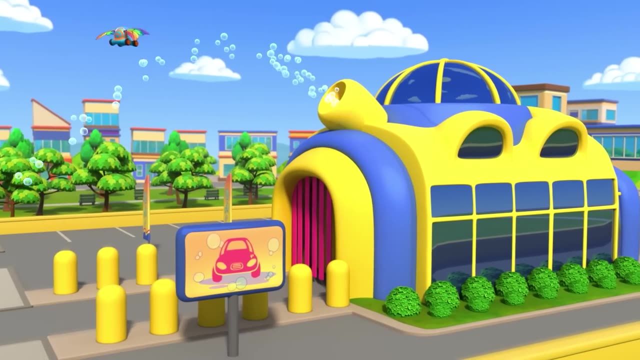 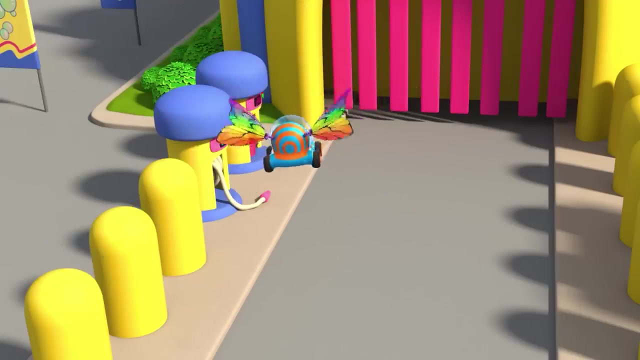 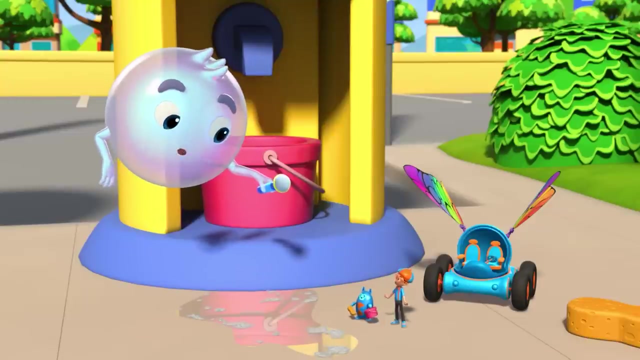 Shrieky down. The Blippi-mobile is ready for adventure. The Blippi-mobile is ready for adventure. The bubbles are from the car wash. The bubbles are from the car wash. Let's give it a wash, Hi. Oh, good boy. 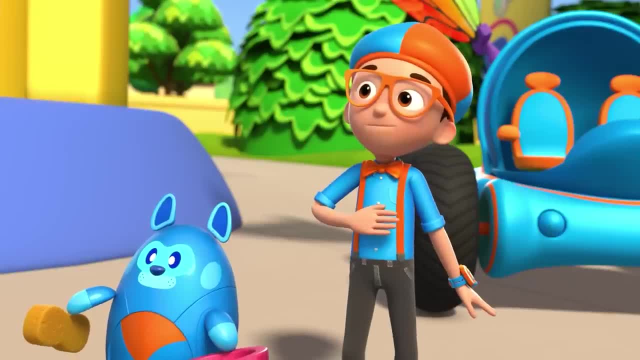 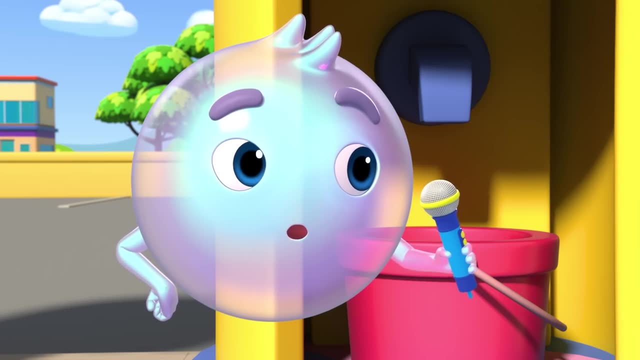 Marvin, Marvin Bubbly. Hey, It's me Blippi, And this is Deebo. We're here to learn how to- Wait a second. Are you a pop star? Haha, sure am. My mom loves you. 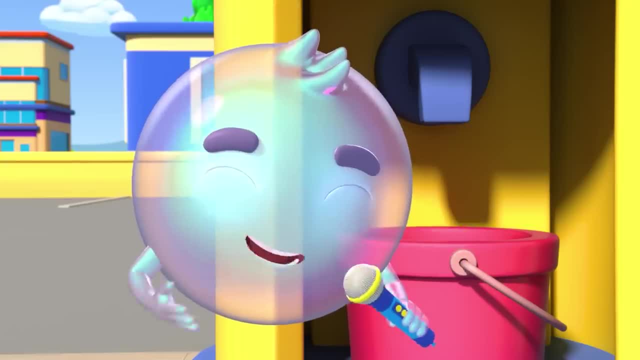 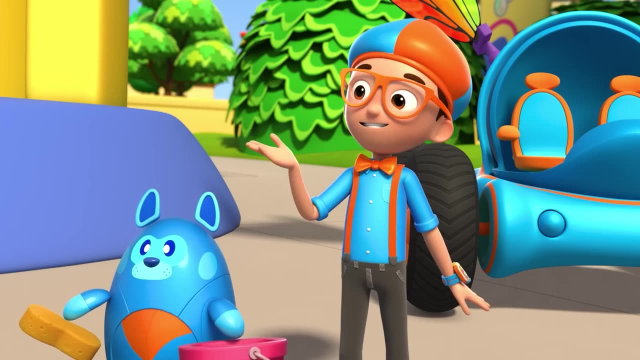 My mom loves you, Thank you. thank you very much. You're far too kind. So what are you here to learn? So what are you here to learn? Deebo and I are here to learn how bubbles are made. Deebo and I are here to learn how bubbles are made. 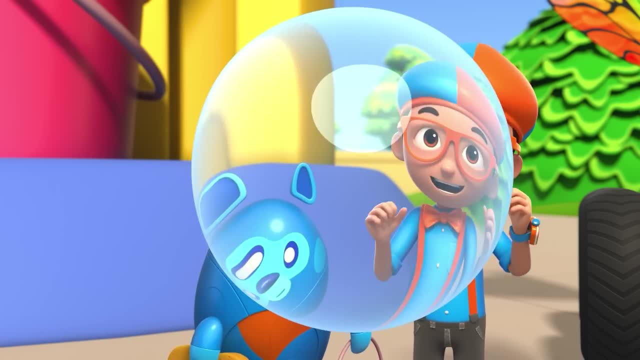 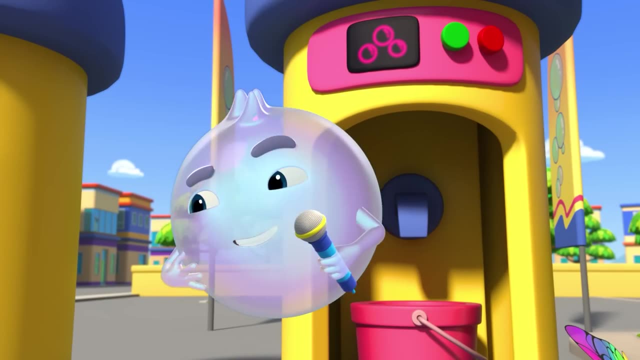 So glad you asked. The surfaces of bubbles are soft. Ooh, which makes them pop easily. Ooh, which makes them pop easily. That reminds me we need more bubbles, And I know just the fella to show you how. 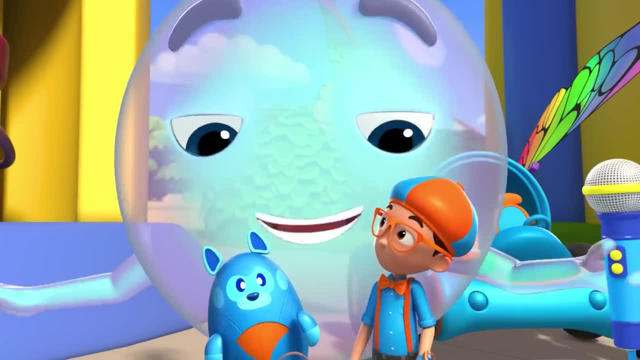 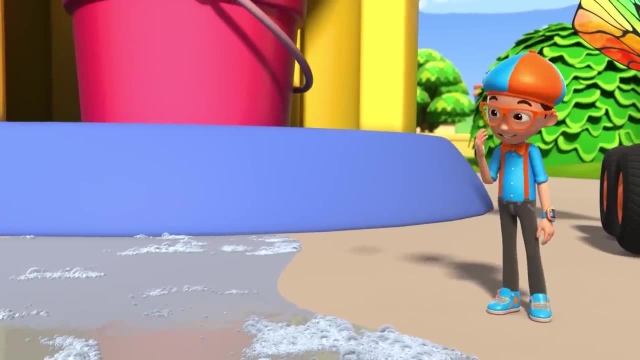 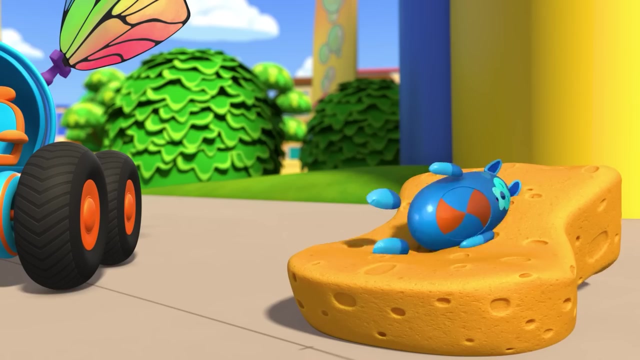 And I know just the fella to show you how. Hmm, Can you guess? It's me Marvin Bubbly. Come on, Whoopsies. The first step is to get water. The first step is to get water. Then we need some soap to mix with it. 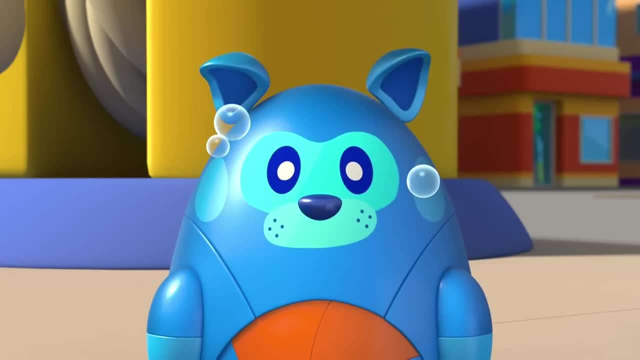 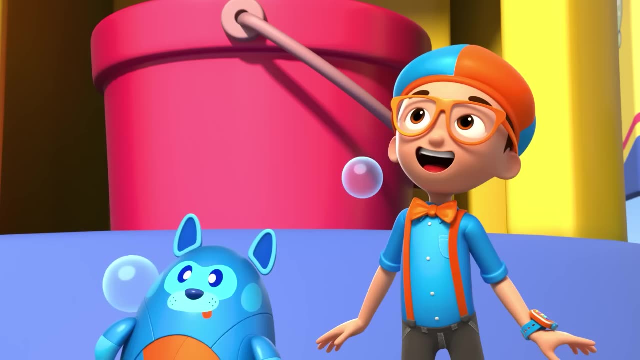 Then we need some soap to mix with it And Shoo-ba-dee-doo-boop, Voila, You've made bubbles. You've made bubbles, And look how they float. Us bubbles can float like that, because we're just air that's trapped inside. 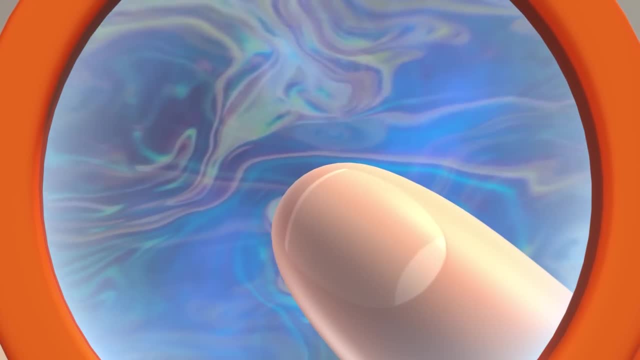 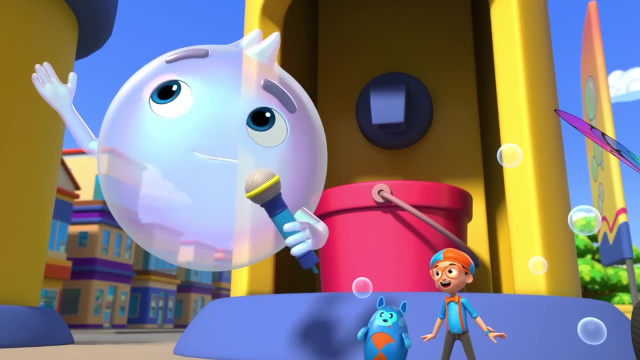 a thin layer of soapy water. a thin layer of soapy water. Whoa So bubbles are made by blowing air into soap. Whoa, So bubbles are made by blowing air into soap. That's right. Which reminds me, Let's make some more bubbles. 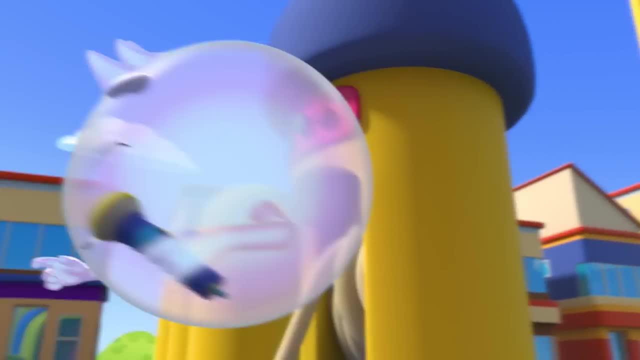 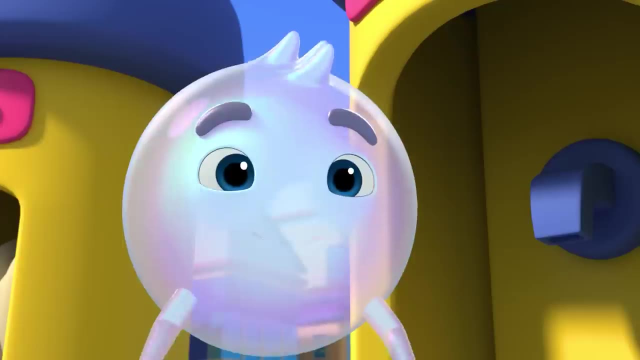 And I know just the fella. to show you how It's you, It is me, Just dip your hands in the water, Get them sudsed up on the soap. Make a circle with your hands and blow. Make a circle with your hands and blow. 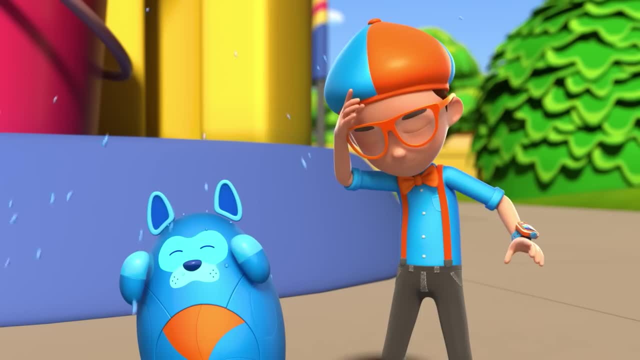 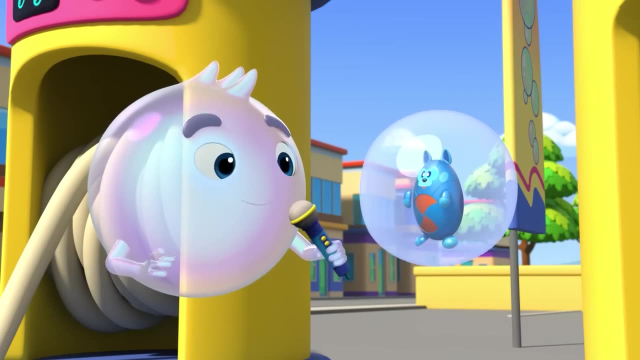 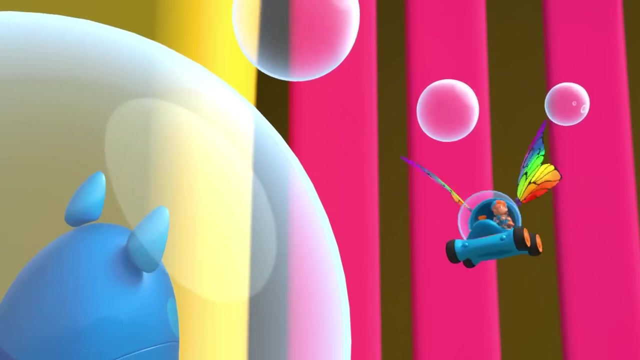 Whoa, It's bigger than you. Check this out. Check this out. Catch me if you can. I've got new heights to reach. I've got new heights to reach. Woo-hoo-hoo-hoo, Keep flying high, Marvin. 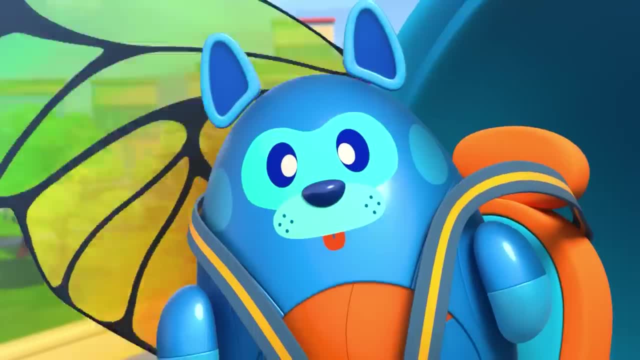 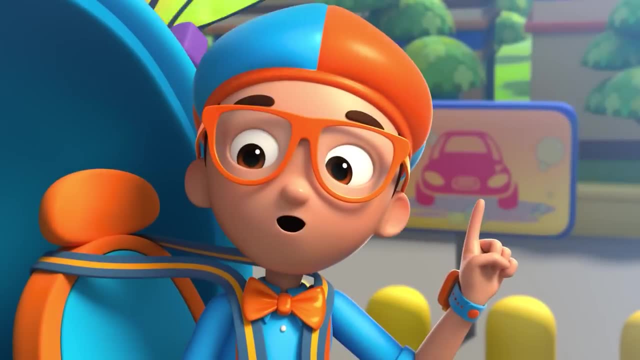 And thanks for helping me get the answer to my question. How are bubbles made? They're made when air gets trapped inside a thin layer of soapy water. Upload answer: Devo. Bye-bye Marvin, Bye-bye Blippi. 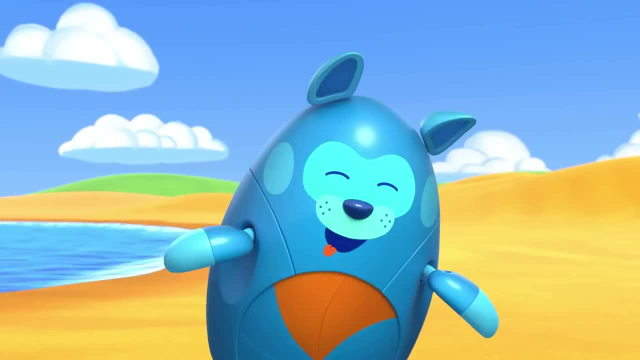 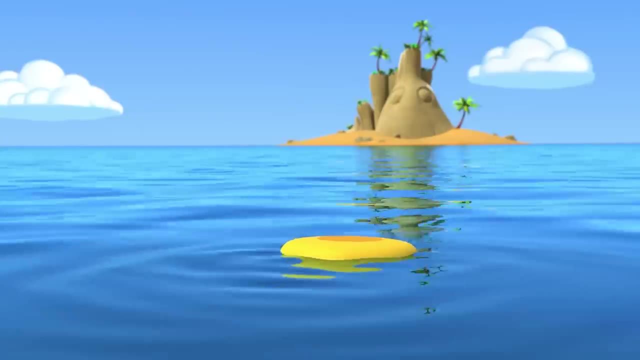 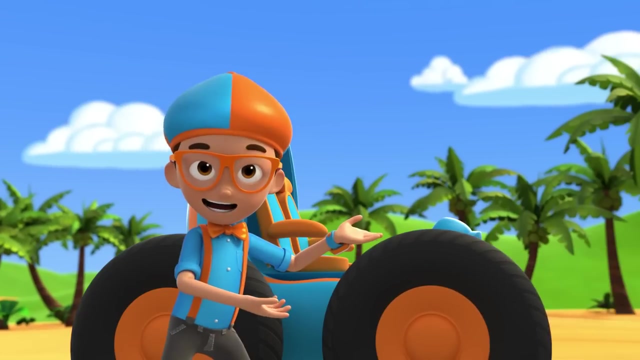 Bye-bye everyone, Bye-bye Blippi. Oh no Devo. Look how the water is carrying the frisbee far away towards that island. Hmm, I wonder, Why don't islands float away? You're right. 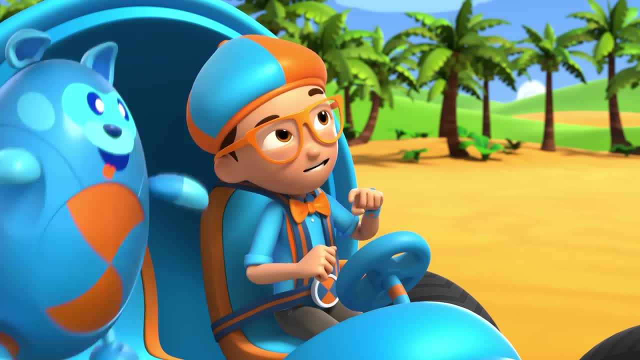 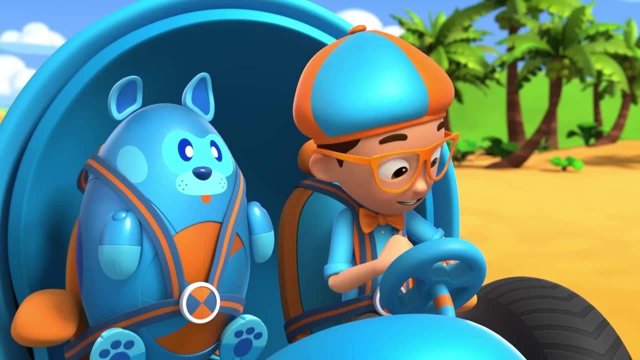 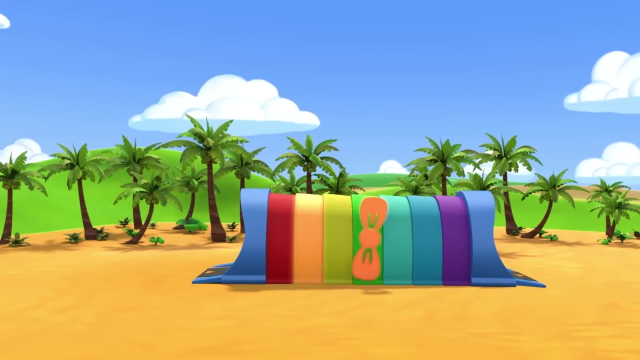 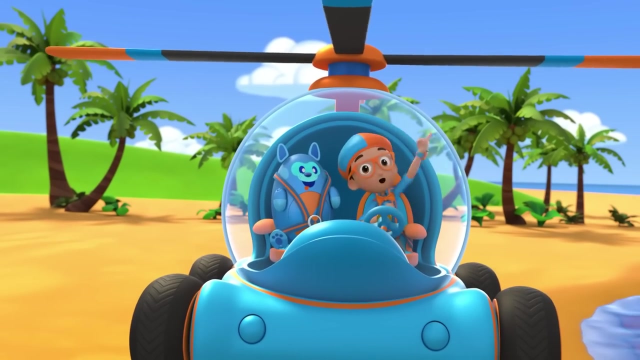 Let's go ask the island and find out. I'm gonna need helicopter blades and duck feet. Helicopter blades, duck feet- confirmed. Activate Blippi Station. Let's go. The Blippi-mobile is ready for adventure. Ooh, Hello up there. 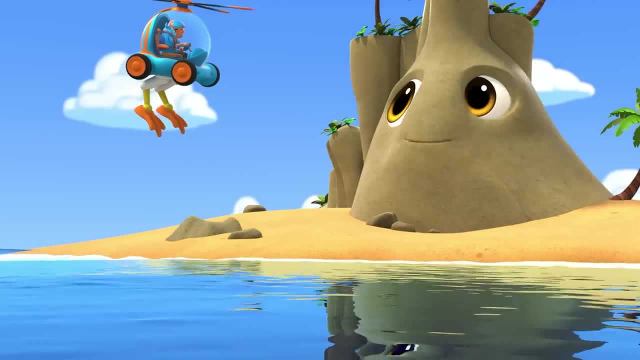 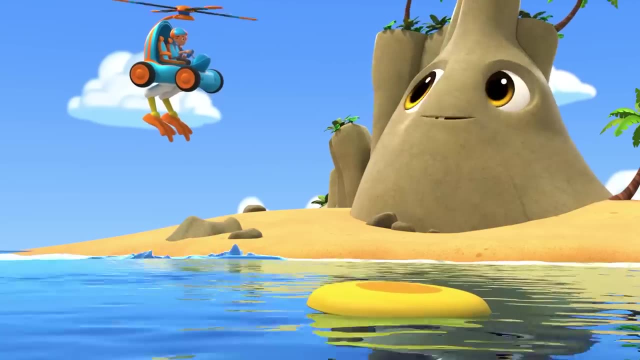 Hey, It's me Blippi, and this is Zubo Nice, to meet you both. I'm Ivan. Ivan, why don't you float away? I think it has something to do with my bottoms. Ooh, I know. 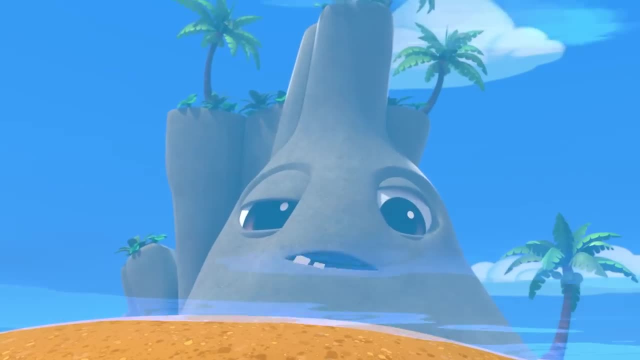 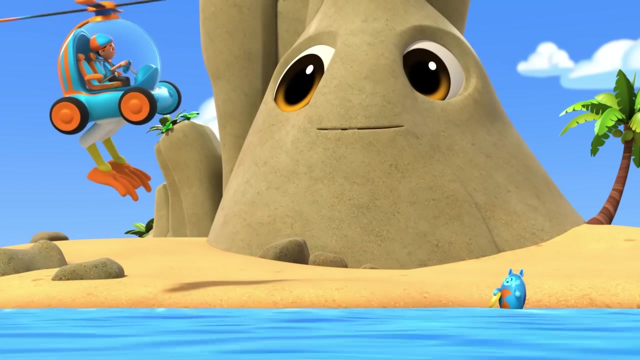 Let's look underwater, where my bottom is, to find out. Oh wait, I can't see down there. You're right, Devo, It would be great if you sucked up the water so we could see the bottom better. I can't wait to see what's down there. 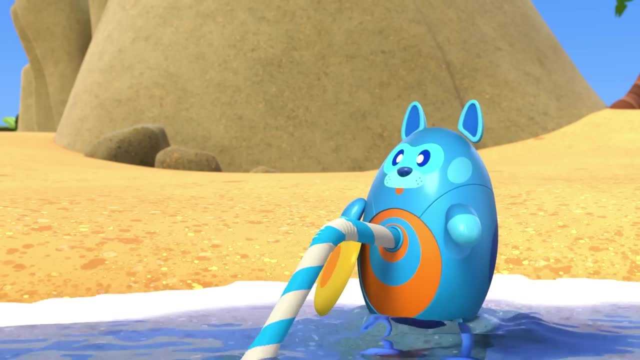 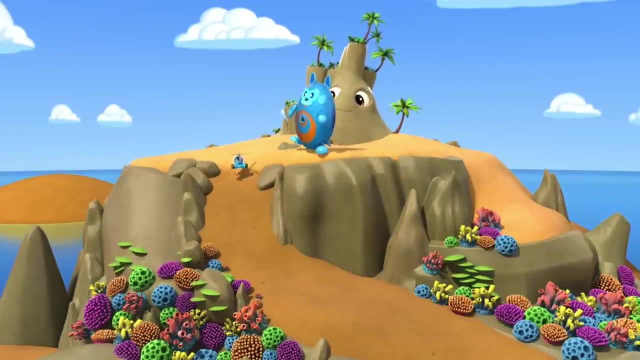 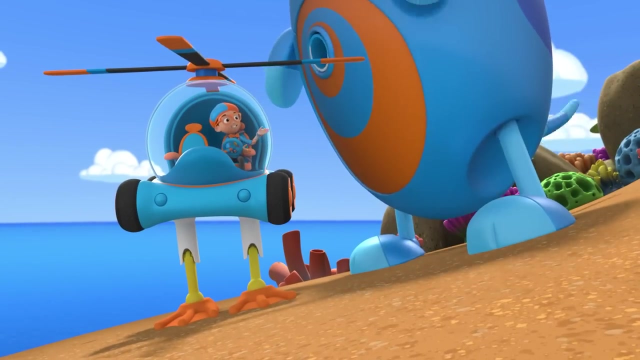 Okay, Devo Drink up. Wow, These colorful coral reefs are so beautiful. We can see so much now. And, Ivan, you're way bigger than I thought. Thanks, I'm even bigger. You're only at my belly button now. 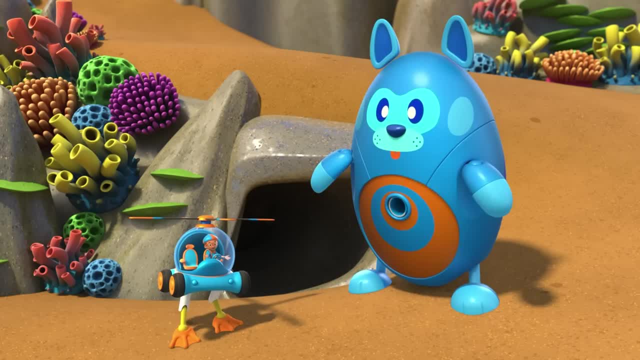 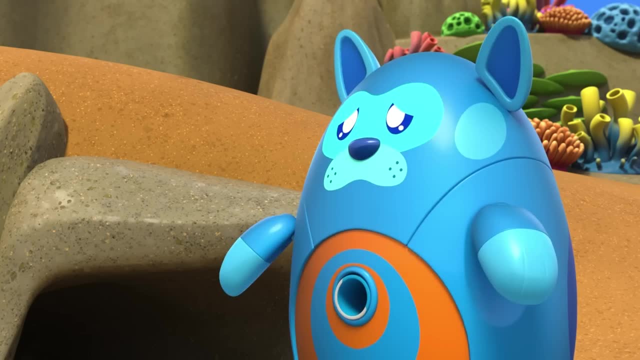 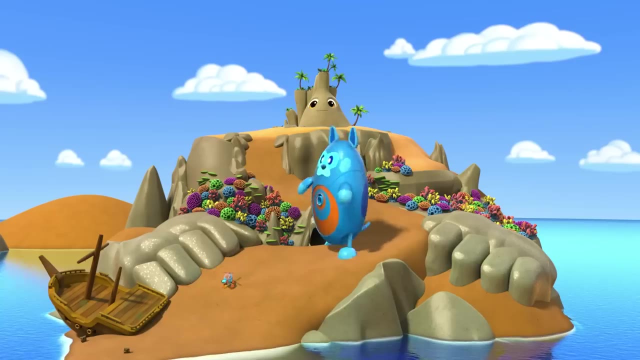 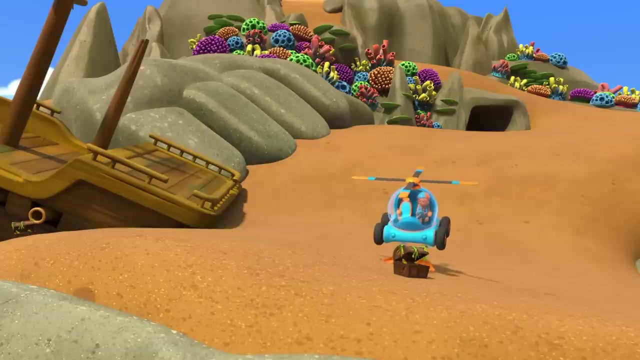 see. Oh, Devo, can you drink up more water so we can see the bottom, Are you okay, Devo? Ivan, You have so many amazing things on you. Hey, wait, Are we at the bottom now? No, 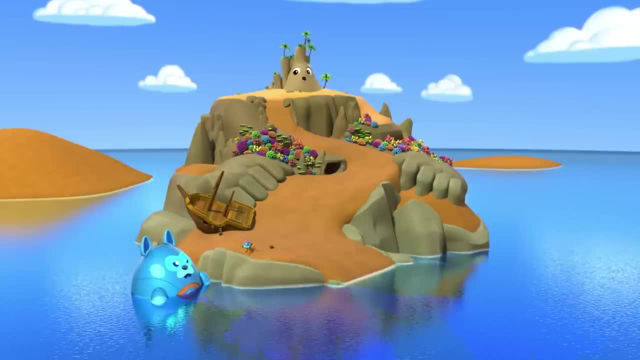 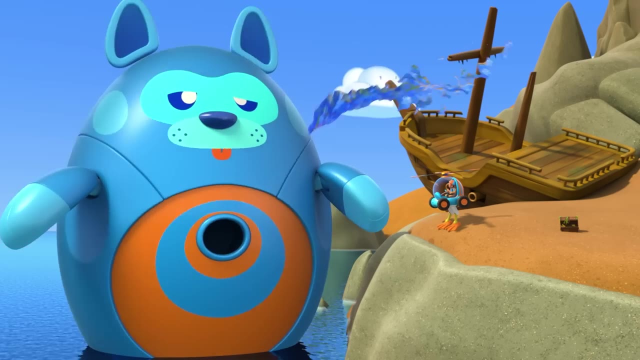 You've reached my knees- Still a bit of a way to go. Do you think you've got one more big goal left in you, Devo? We're so close to being able to see the bottom. Woohoo, I knew you did. 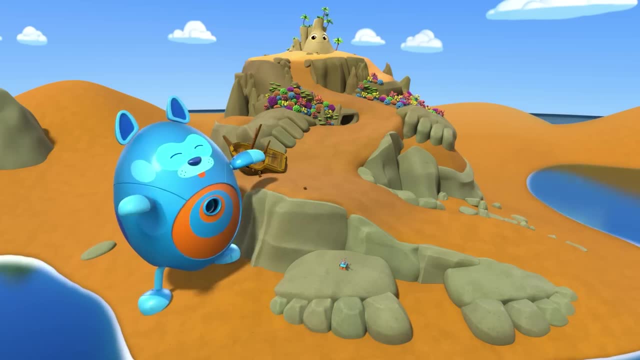 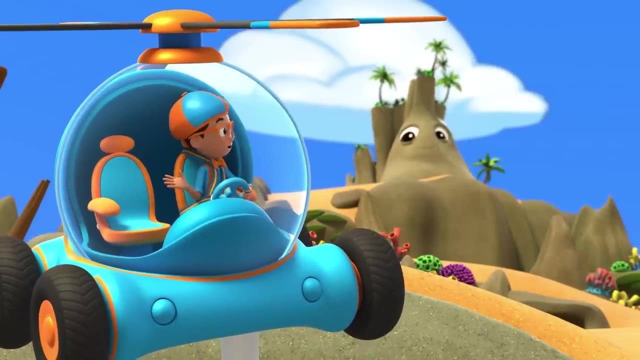 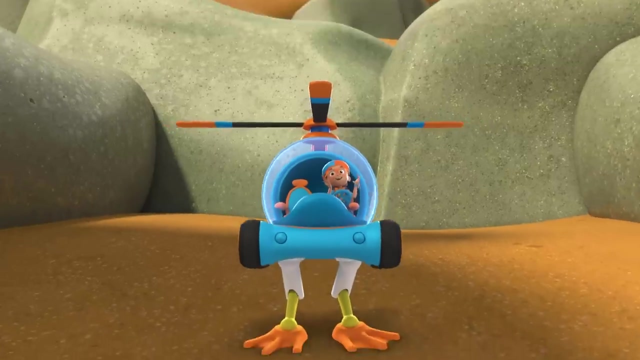 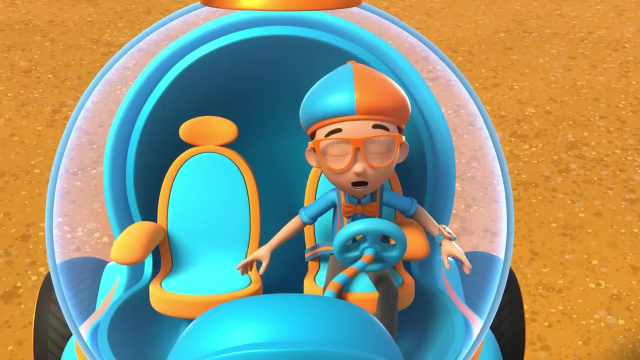 You made it. Blippi, You're at my feet Really. How can you be sure? Because it tickles when you walk around. Ivan, You're attached to the bottom of the sea, You're like a mountain, Oh, Devo. 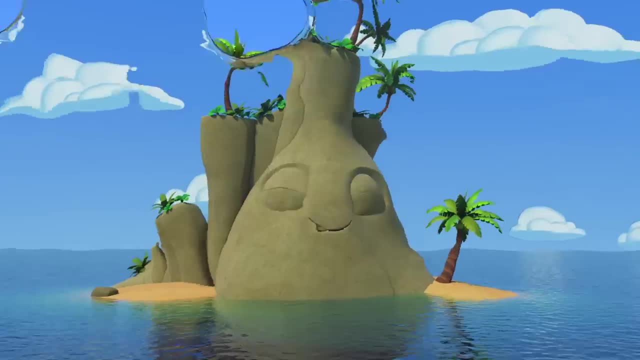 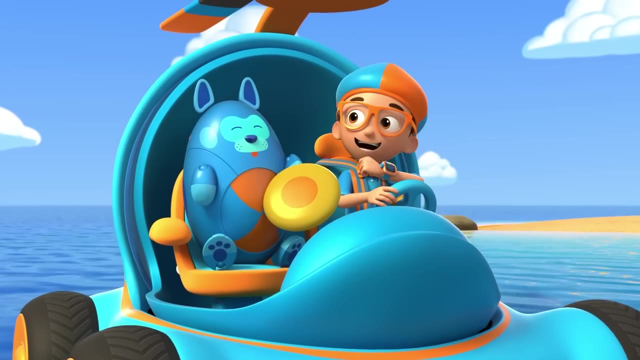 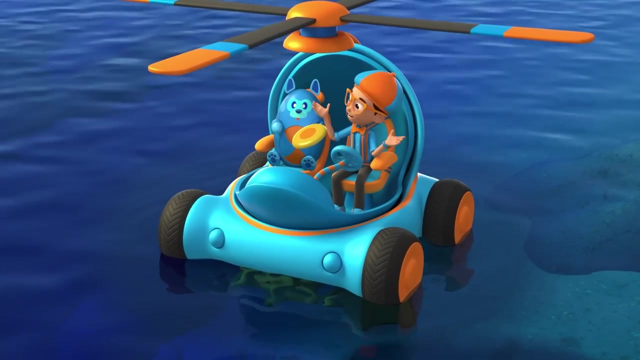 Oh no. Ah Well, that was fun, And now I have the answer to my question: Why don't islands float away? Islands don't float away because they are mountains attached to the sea floor. Upload answer: Devo, Thanks for all. 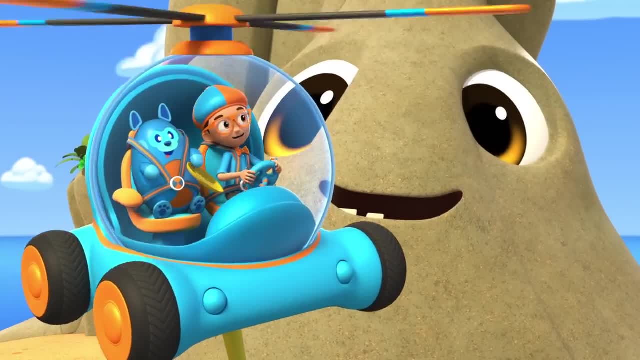 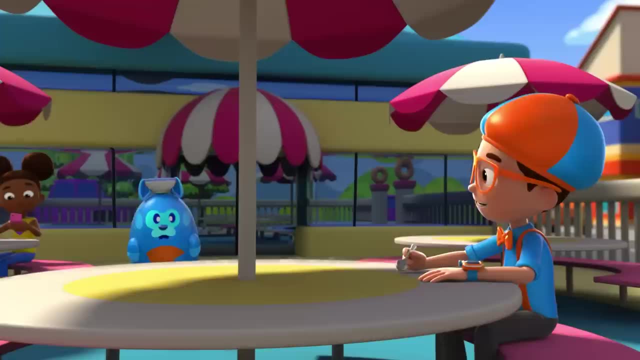 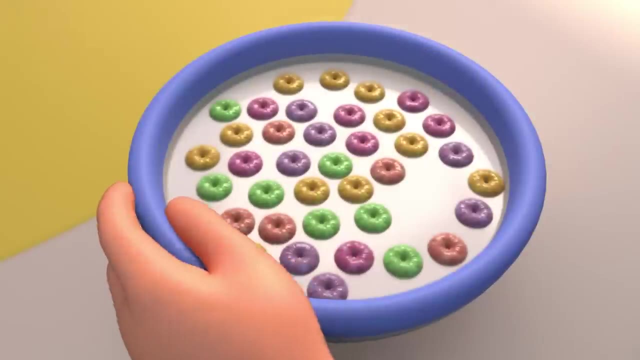 your help, Ivan, You rock. Hope to see you again Anytime. I'm here to stay. Bye-bye, Blippi, Easy, Careful now. Whoa, I'm hungry. This cereal is soggy. Hmm, I wonder. 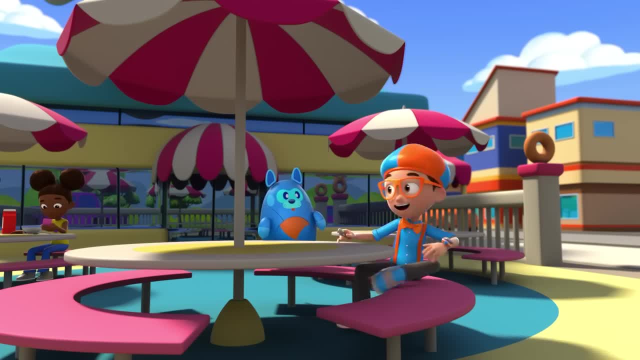 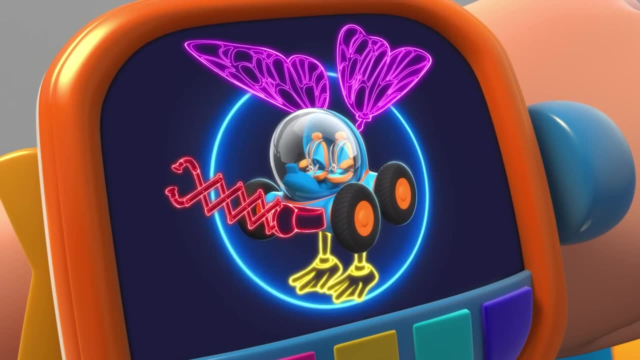 why does cereal get soggy? Great idea, Devo. We'll shrink down and find out. I'm gonna need wings duck feet and the grabber arm. Wings- duck feet. grabber arm- Confirmed. Activate Blippi Station. 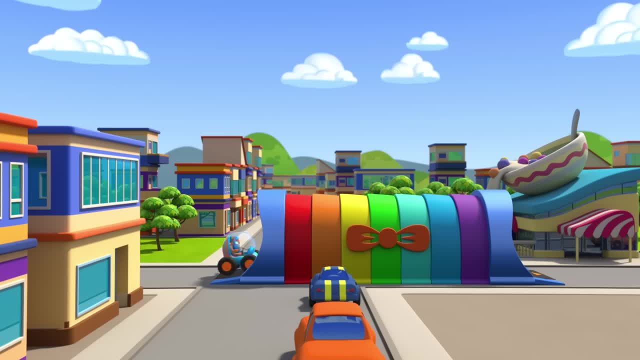 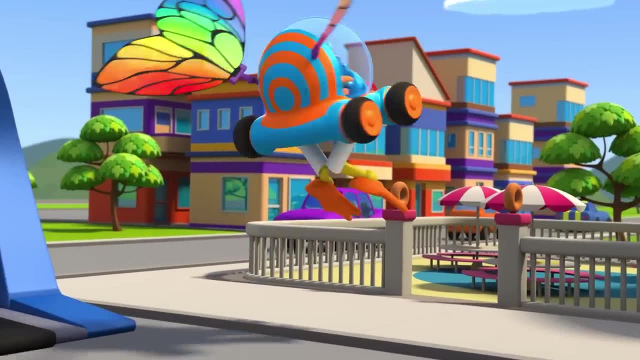 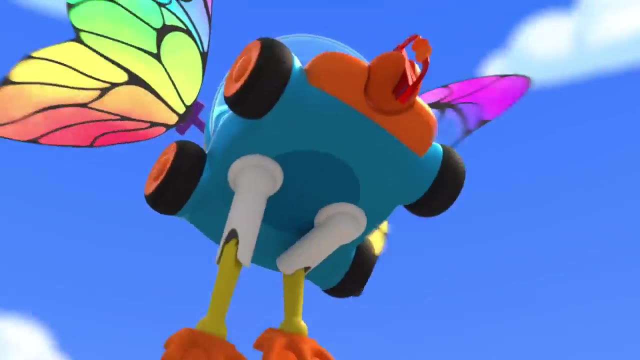 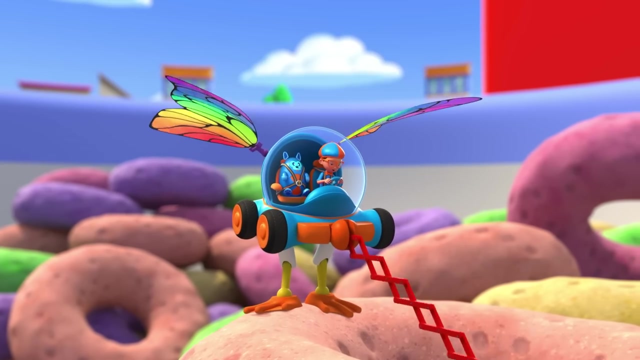 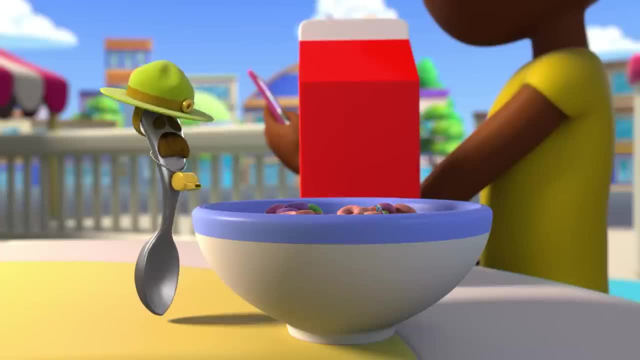 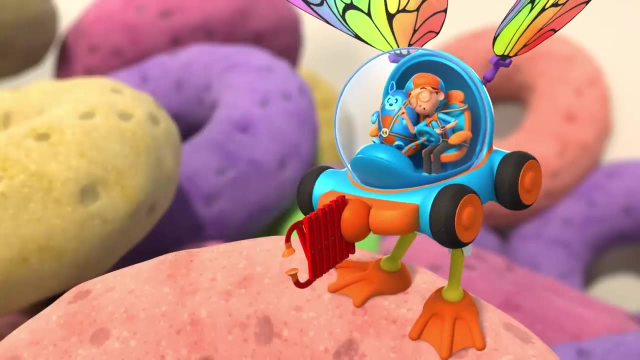 Whoa, Who are you? I'm Scooper the Spoon. That's Sergeant Scooper the Spoon to you. Hey, It's me Blippi and this is Devo. We're here to learn why cereal gets soggy. Well, you came to the best. 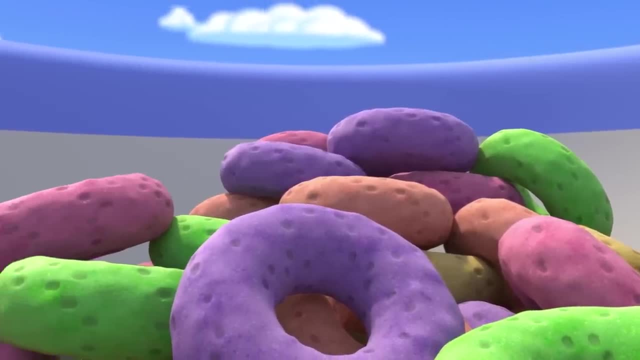 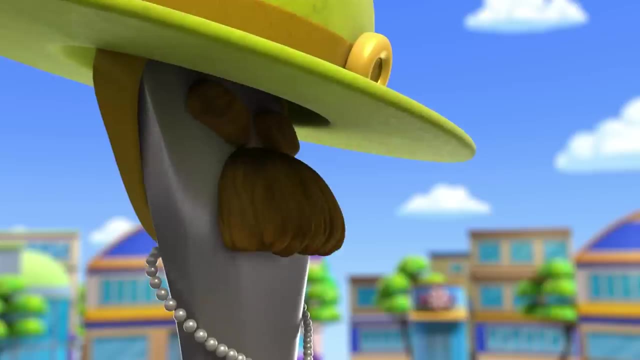 of the best. These crunchy pieces of cereal are as hard as nails. The only problem is we got incoming milk in T-minus 30 seconds. What happens then? The cereal gets all wet Blippi. At first it may seem like cereal is 100% solid. 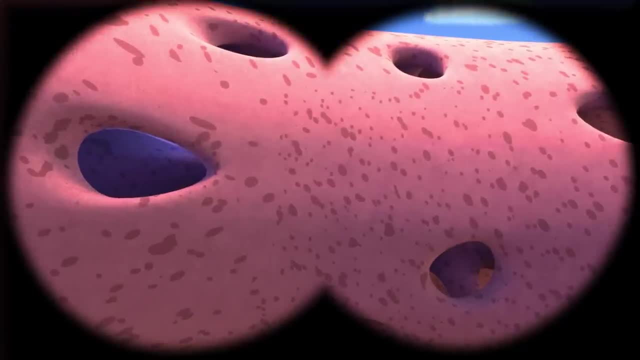 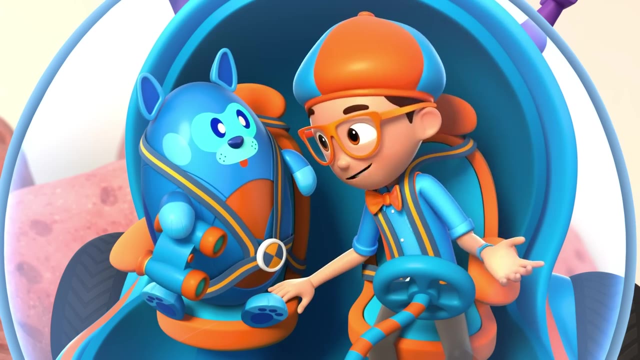 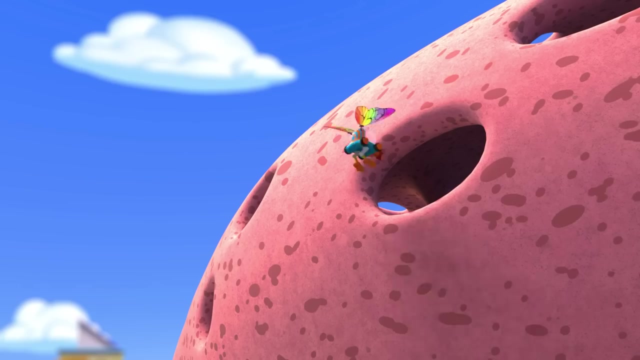 but if you look closely it's actually porous. That means full of tiny little holes. Good idea, Devo, I'll go gather some intel and you stay here on the lookout Shrinking down again. It's like a cave made of. 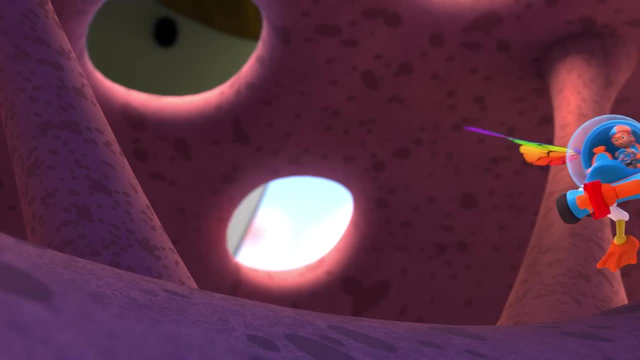 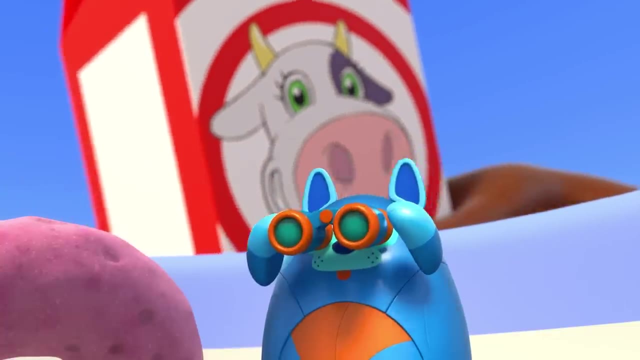 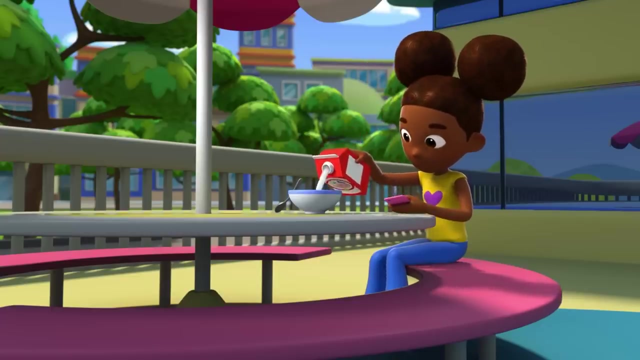 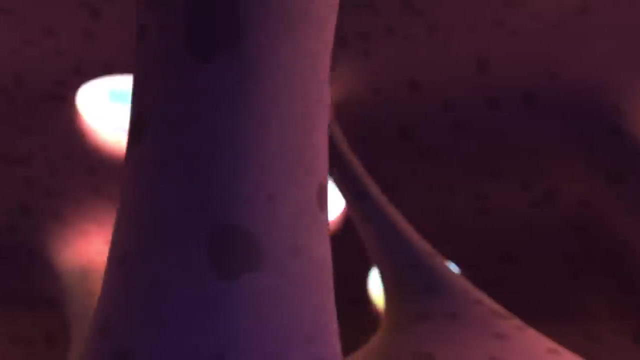 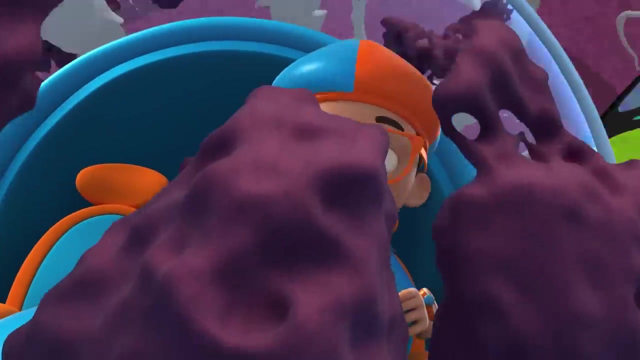 cereal. All those holes you're flying through are open space for milk to fill And make the cereal soggy. Then it expands and falls apart. Milk incoming Whoa, The cereal is falling apart. Time to get out of here Throwing off. 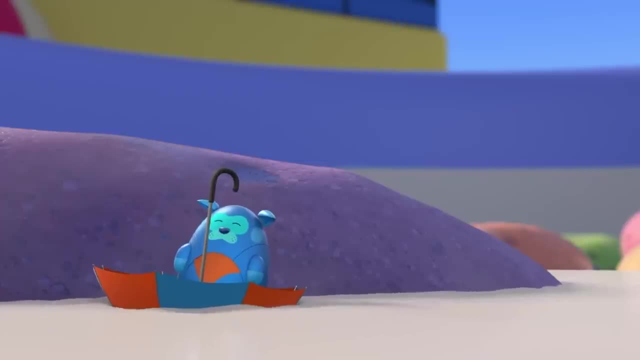 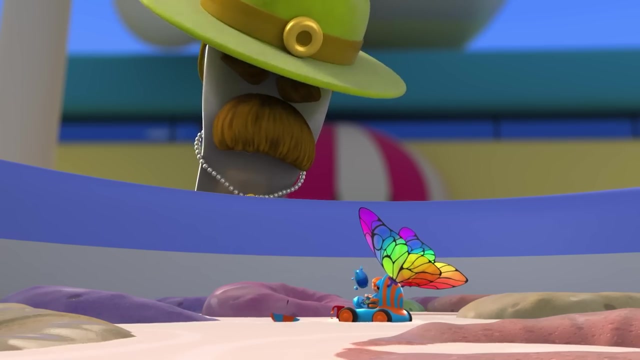 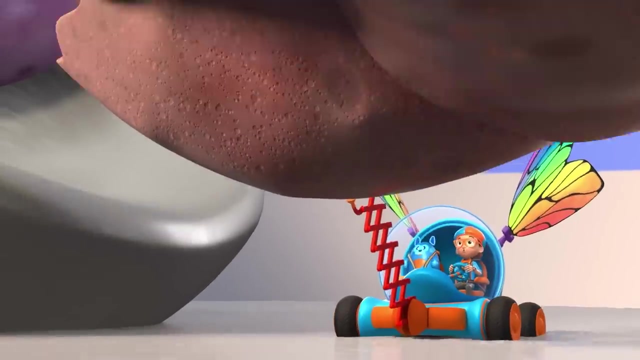 No time to float around. We've got a cereal rescue mission to complete. Now that the milk has infiltrated the cereal, we've got to scoot fast. before the cereal gets soggy, We're on it. Oh no, I got it. 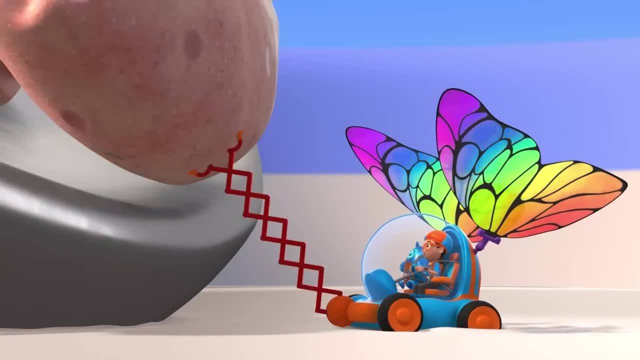 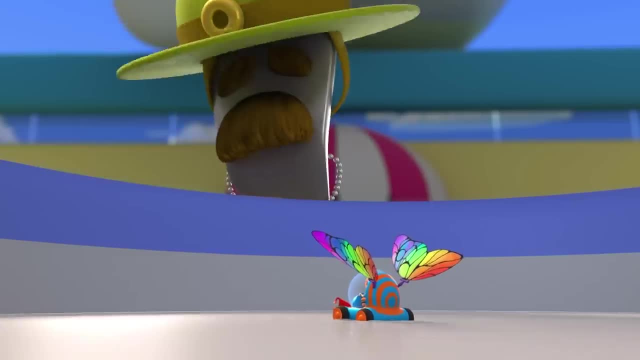 You see, in the few minutes the cereal has been in milk. it has absorbed the liquid through the holes, A lot like how a sponge absorbs water. With your help, we got all the cereal out safely. Well done, troops. Thanks, Sergeant Scooper. 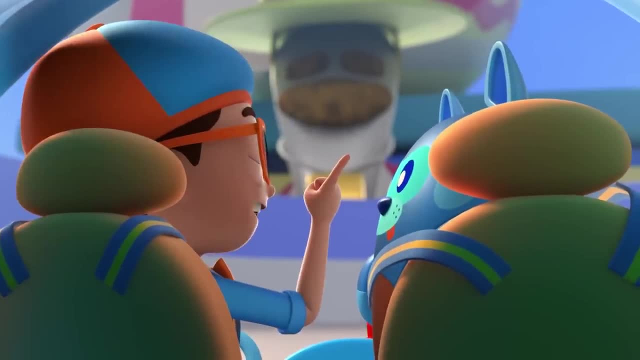 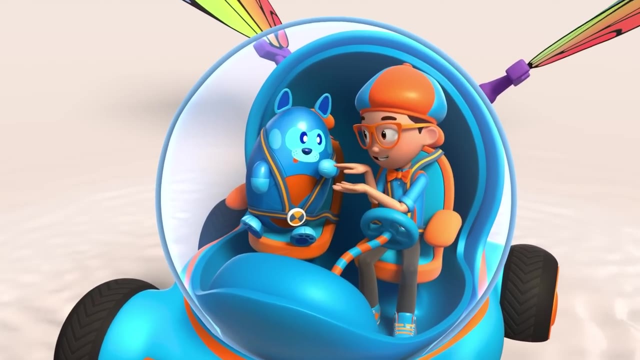 And I got the answer to my question: Why does cereal get soggy? Cereal gets soggy when milk fills in the tiny holes of the cereal and causes it to expand and fall apart. Upload answer: Devo. Goodbye, Blippi. 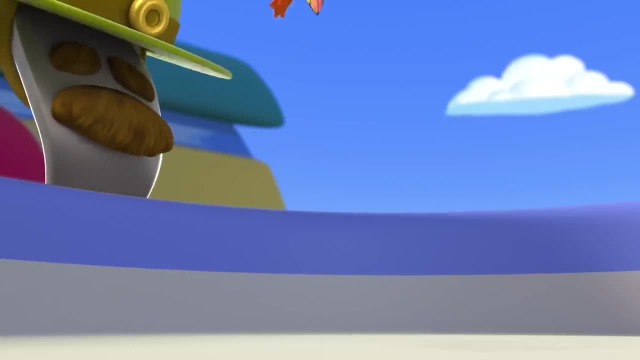 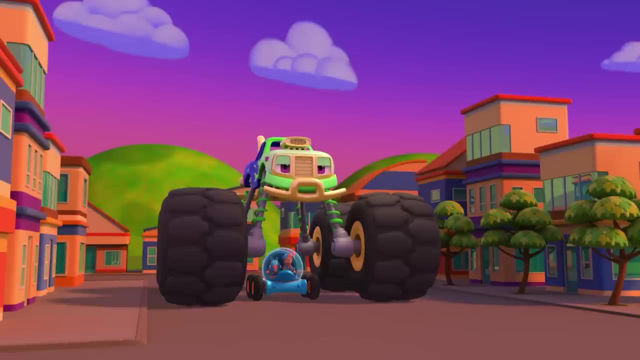 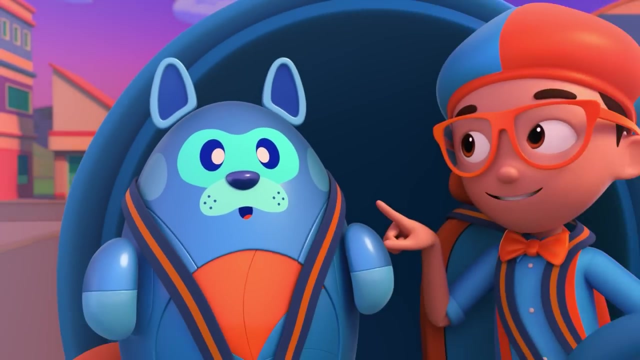 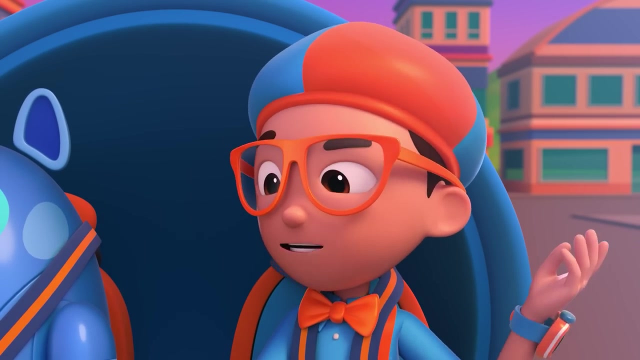 Bye-bye, Sergeant Scooper. Thanks for the scoop. Whoa, That was a gigantic truck. You're right, Devo, I think that was a monster truck. Hmm, I wonder what makes a monster truck special? Good idea. 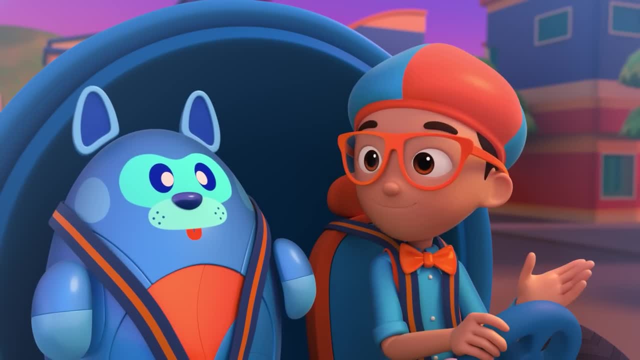 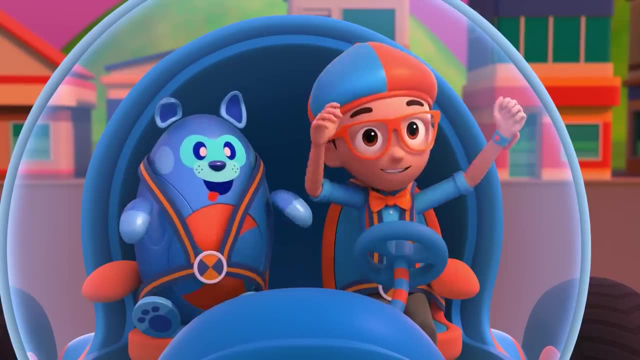 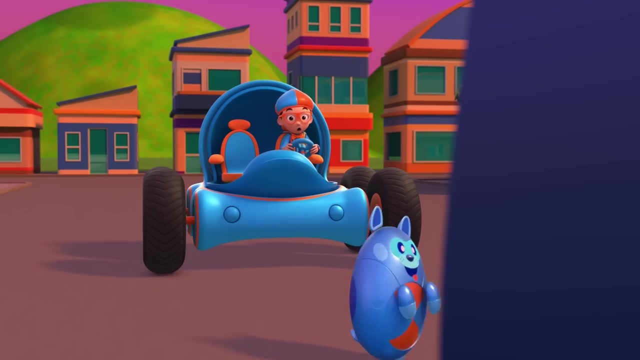 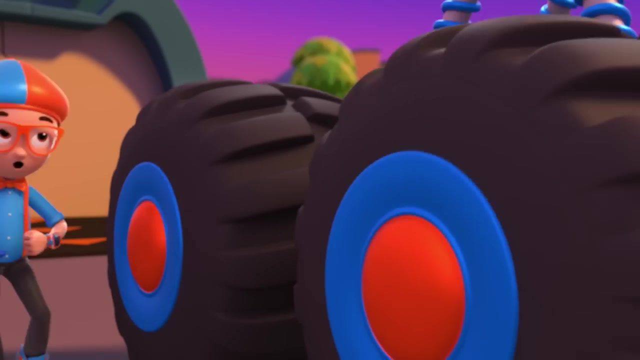 We can catch up with that monster truck and find out. I'm gonna need monster truck wheels. Monster truck wheels confirmed. Activate Blippi Station, Devo, Whoa, Devo. You have the monster truck wheels attachment. You're like a. 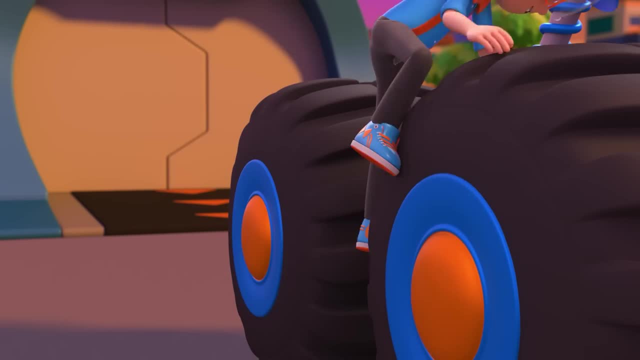 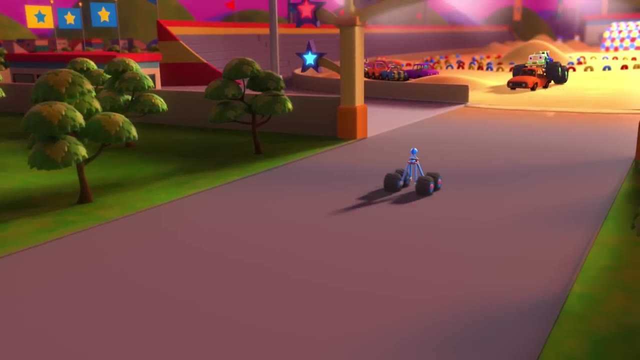 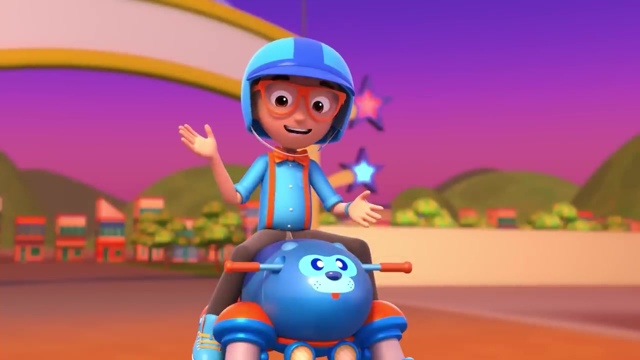 monster truck. Alright, let's ride Devo. the monster truck is ready for adventure. Crush, Crush. Hey, It's me Blippi and this is Devo. You really crushed that car? Hi, Blippi, I'm Megan. 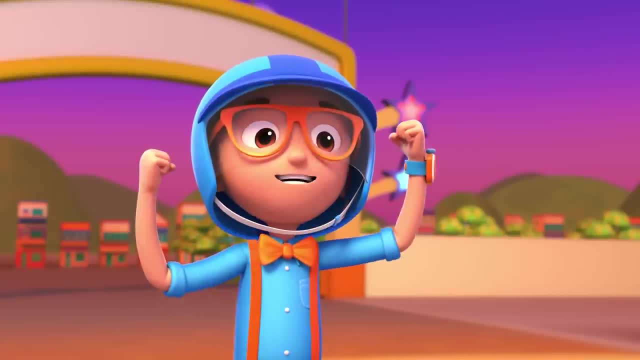 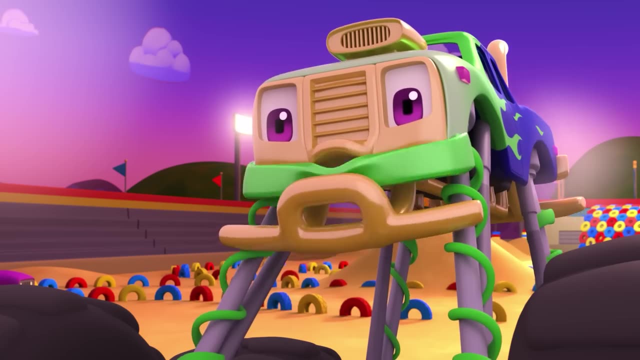 So, Megan, we're here to find out what makes a monster truck special, Cool. Well, I think the best way to answer your question is to show you what I do. Great, You see, I'm a monster truck with big. 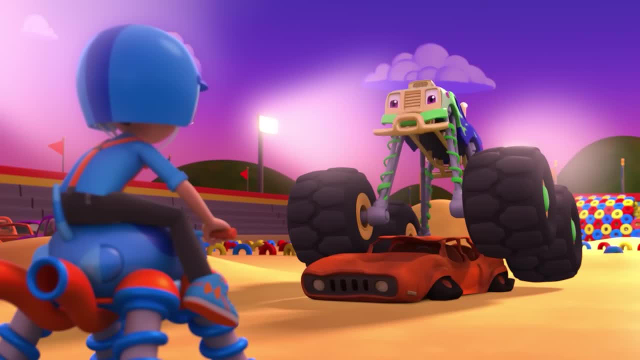 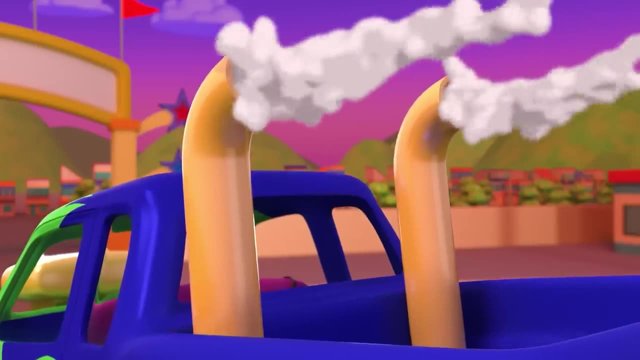 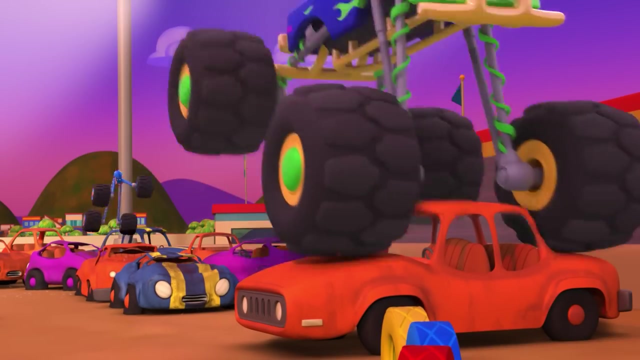 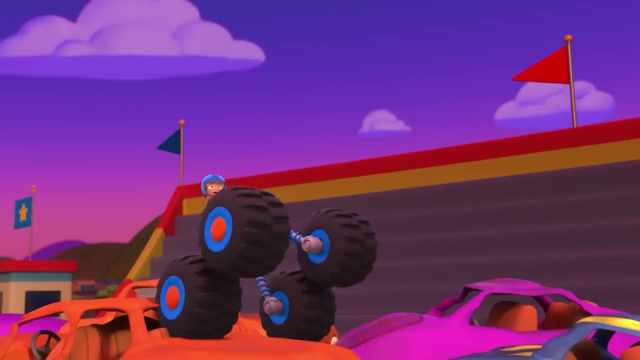 tall monster tires. I'm 13 feet tall. Wow, Let's do this. Alright Crush. We can't bounce as high as you, Megan, And, oh boy, we're almost tipping over. Well, I have heavy duty suspension, which are special. 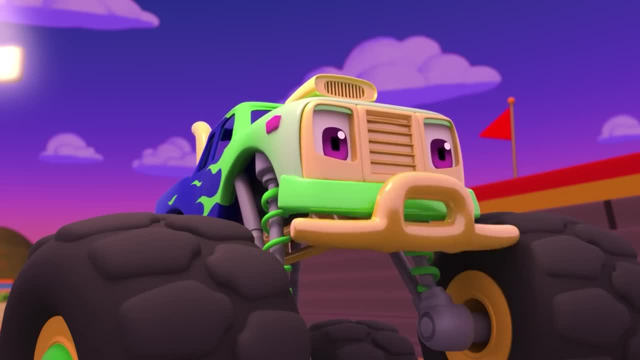 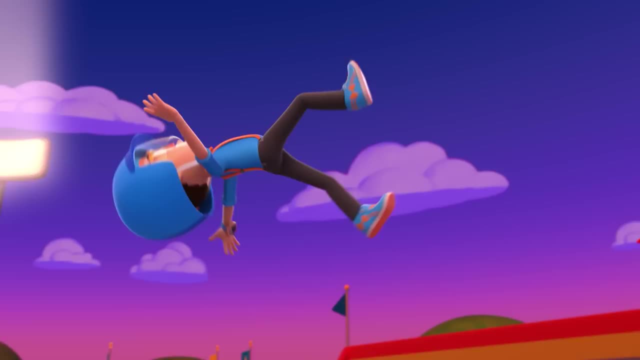 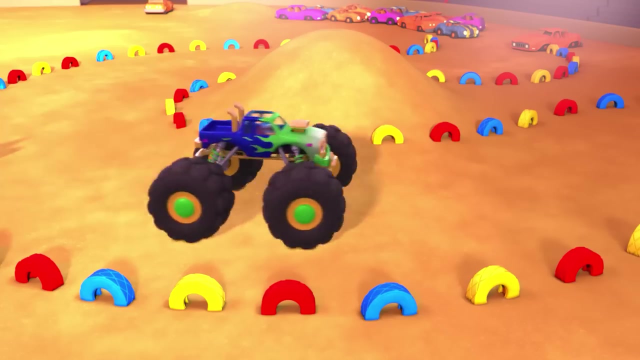 springs so I can bounce way up and down and not tumble over. I use them when I race and have competitions. Cool Yeah, Welcome aboard. Blippi. Buckle up, It's time to dominate the obstacle course. Whoa. 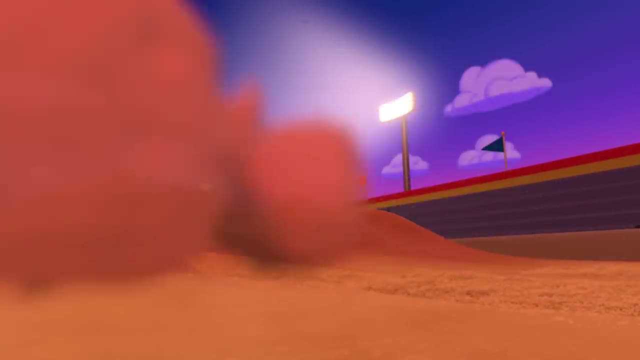 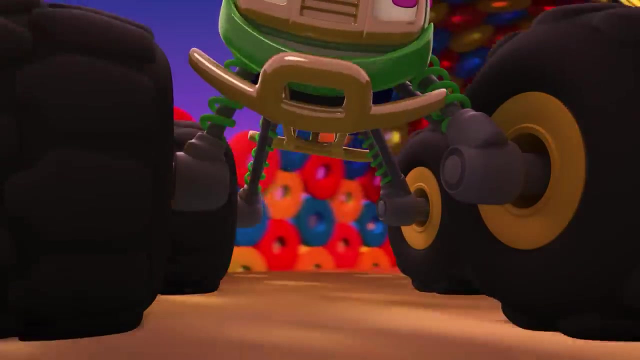 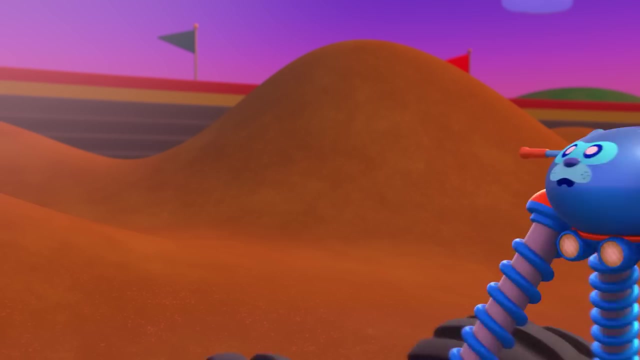 Whoa, Whoa. This is awesome. How can you turn and zigzag so fast? I have something called four-wheel steering so I can turn all four wheels at once instead of just two wheels like a lot of regular trucks- Us monster trucks. 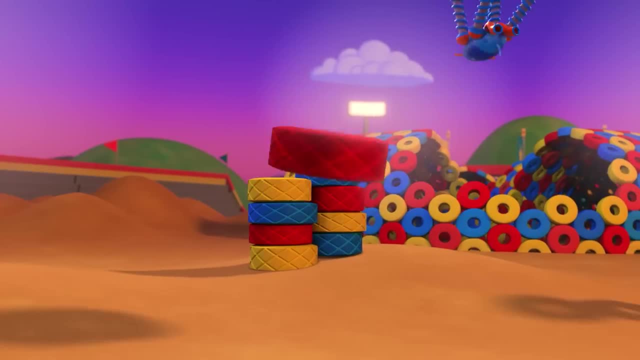 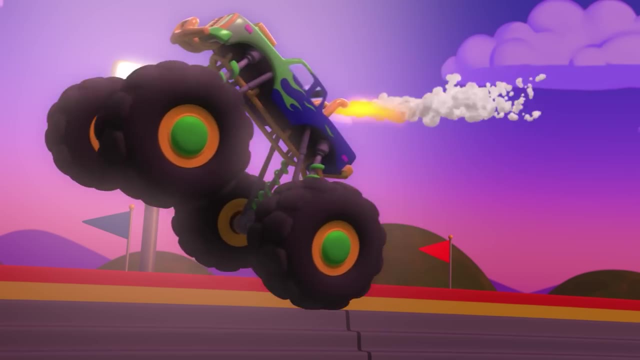 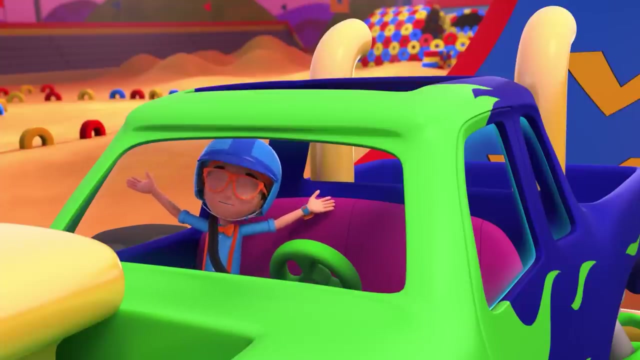 are built for short, high-powered speed. Woo-hoo, Woo-hoo, Woo-hoo, Whoa. Yeah Wee, I nailed that, Megan. that was amazing, And I have the answer to my question: What makes a monster truck special? 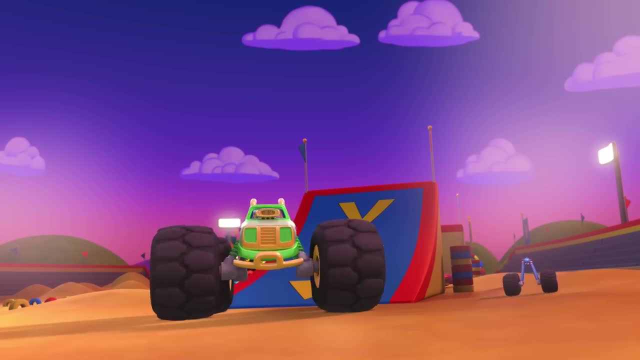 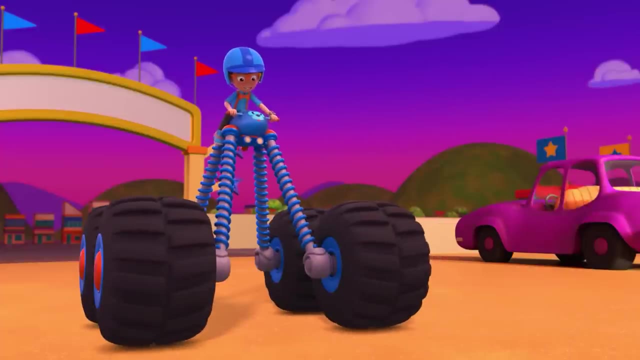 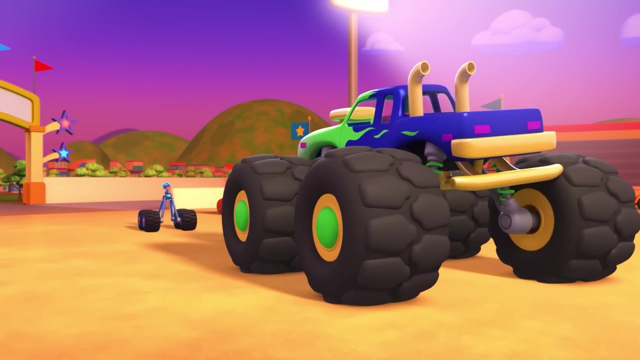 Monster trucks are a special kind of truck with big tires, heavy duty, suspension and four-wheel steering. Upload answer Deebo. Bye, Megan, It was so cool to ride with you. Bye, Blippi, Keep on crushing. 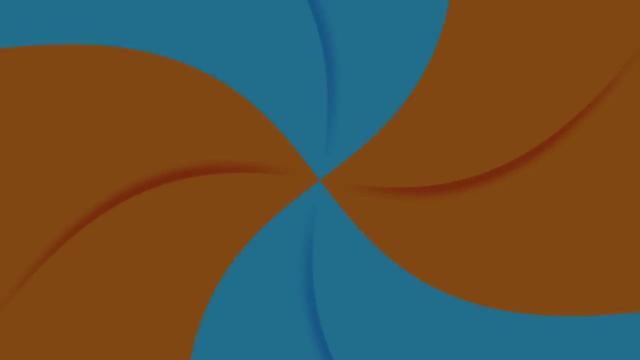 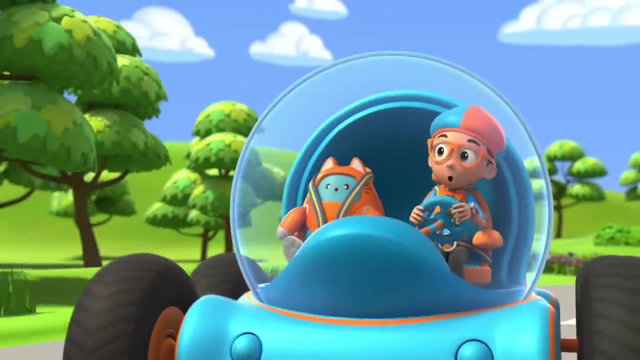 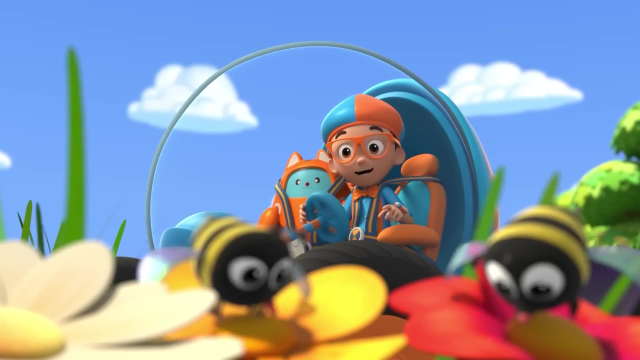 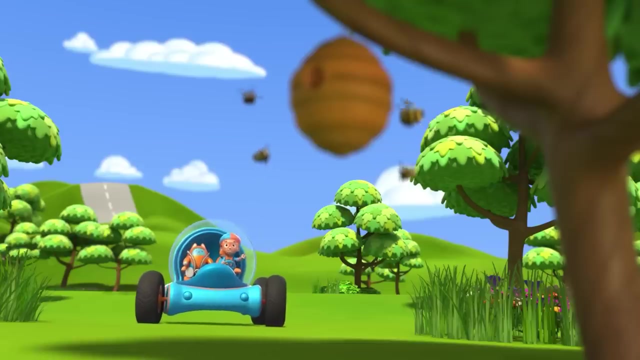 Ha-ha, Woo, Wow. That bee sure seems busy, And so does that one, And that one too. They're all so busy, Ha Well, except that one, Those bees are busy making honey. Hmm, I wonder how do. 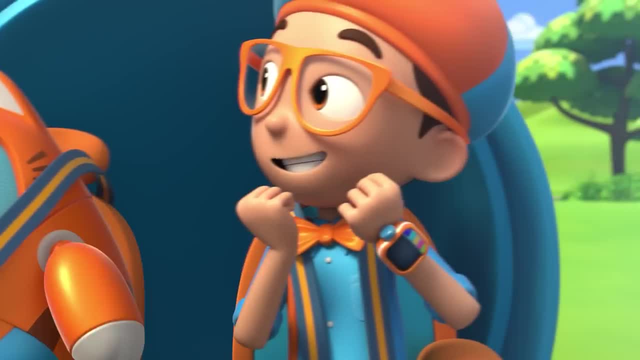 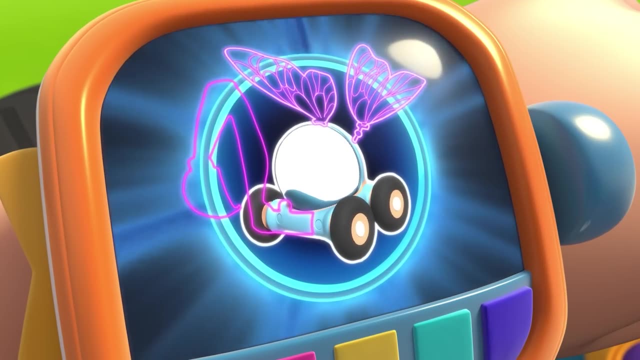 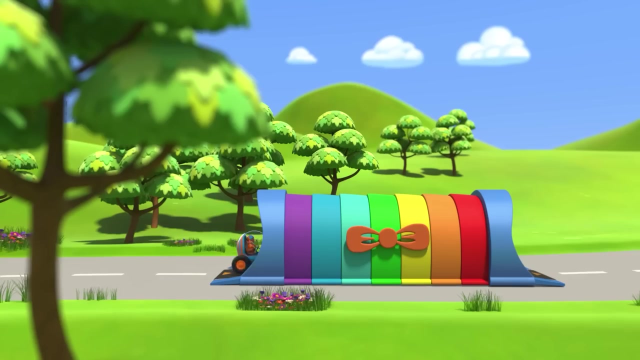 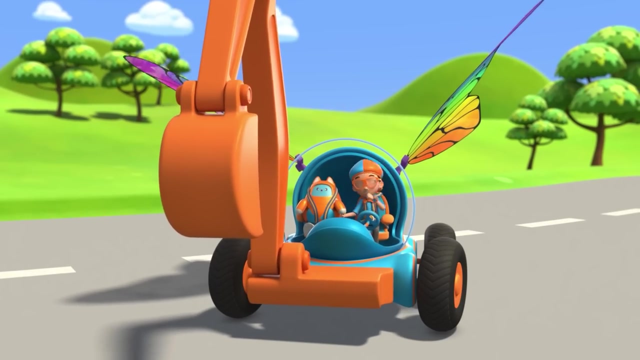 bees make honey. Yes, Let's go into the beehive. I'm gonna need wings and the excavator arm. Wings, excavator arm confirmed. Activate Blippi Station. The Blippi Mobile is ready for adventure. Now we just need to make like a bee. 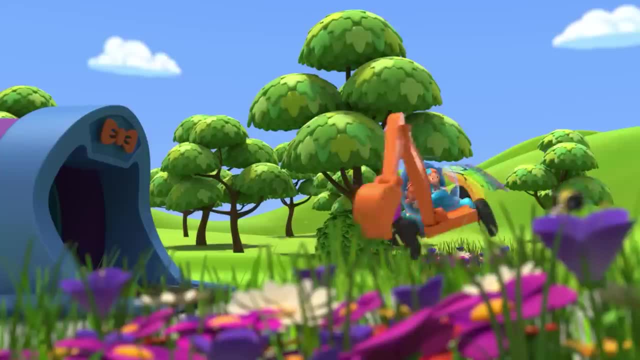 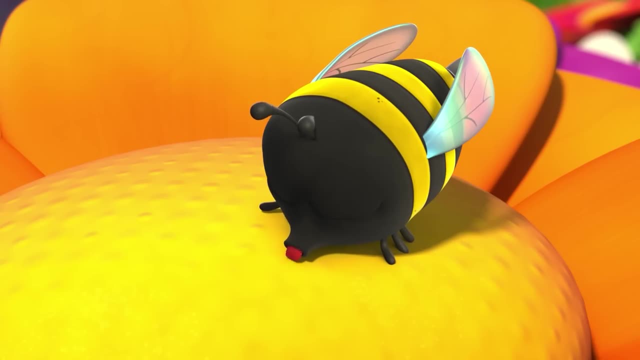 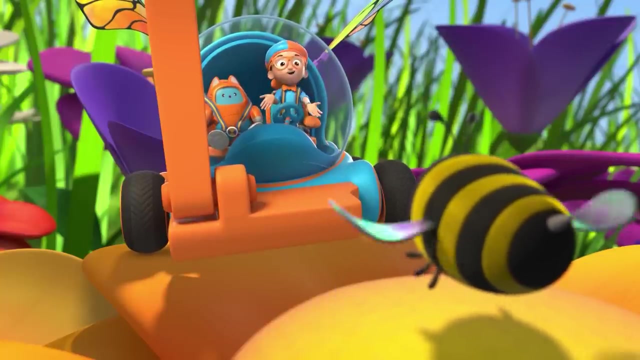 and bee tinier Shrinking down. You're right, Tabs. The bee's tongue is in the flower. Hey, It's me Blippi. This is Tabs. I was wondering how you make honey. Hey, Blippi, I'm Beejon. 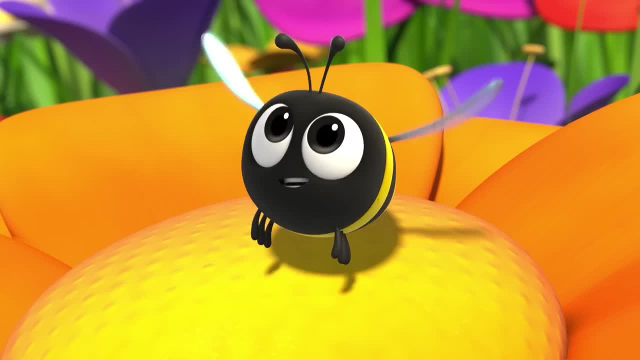 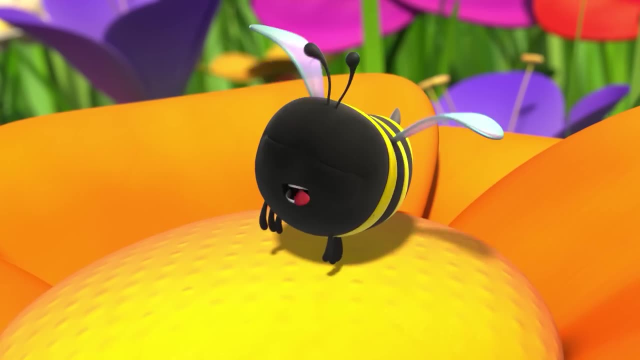 Honey. huh. This is the place to bee, So I'm using my tongue to drink in this sweet nectar. It's how we bees start to make honey. Okay, Time to buzz Into the beehive. Follow me, Spoiler. 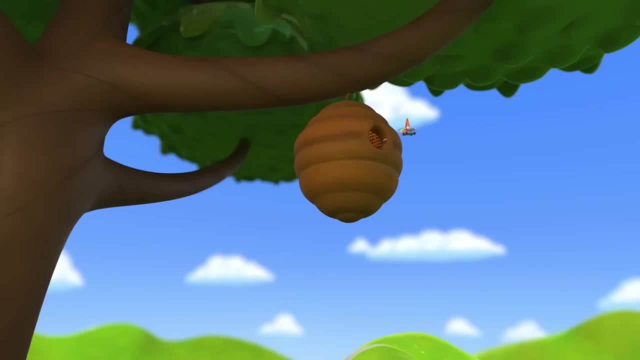 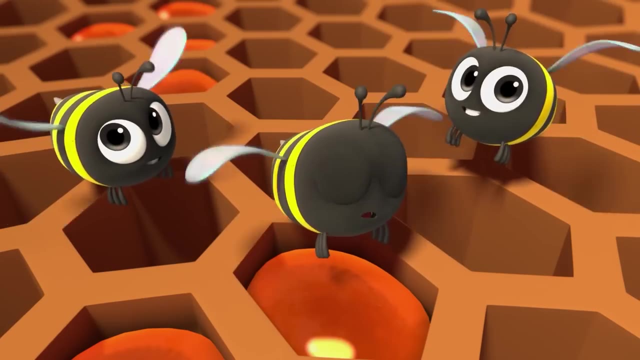 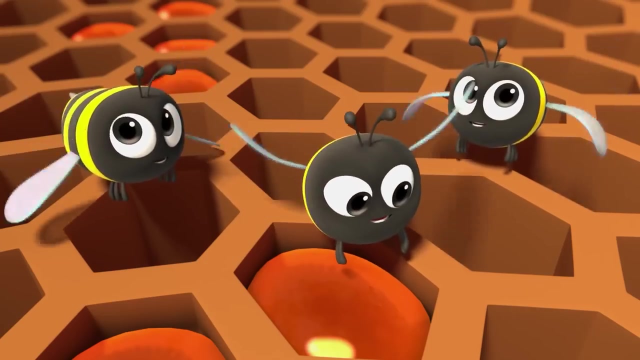 Lots of bees working. It's like a honey factory in there, Beejon, Are they all chewing nectar? Sure are Gotta chew. That's what we do. Chewing makes it thicker. Can't have runny honey. I rhymed again. 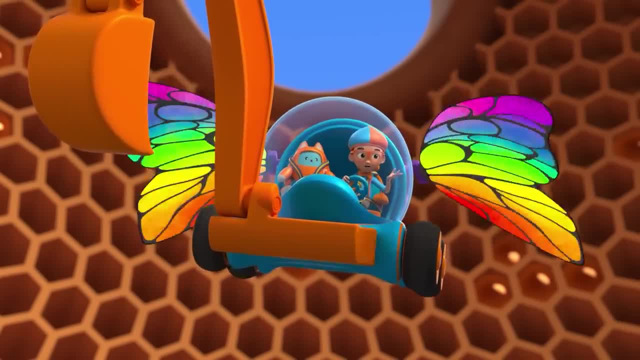 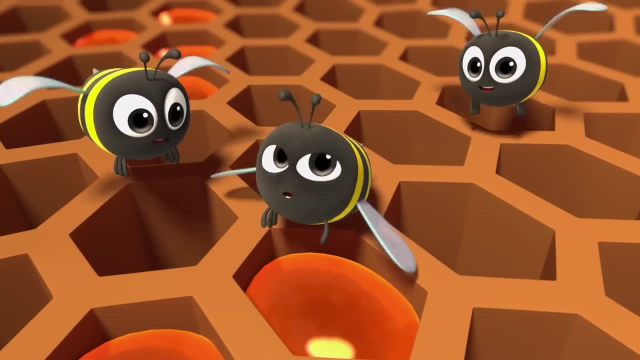 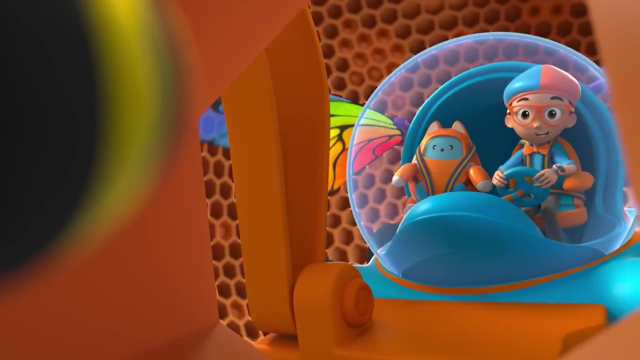 And after you chew, then you have honey. No, no, There's more to show. We chew, then we swallow. the nectar stays in our bellies, becomes honey, then we put it in the honeycomb- The honeycomb. 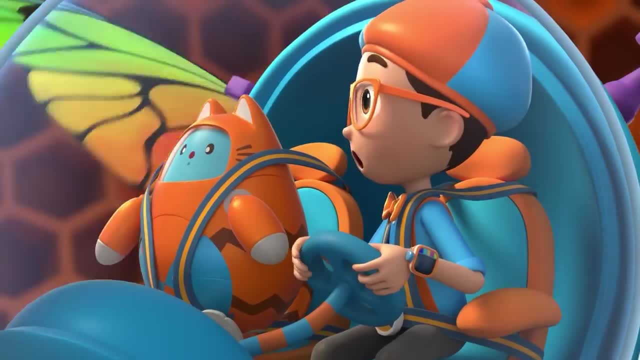 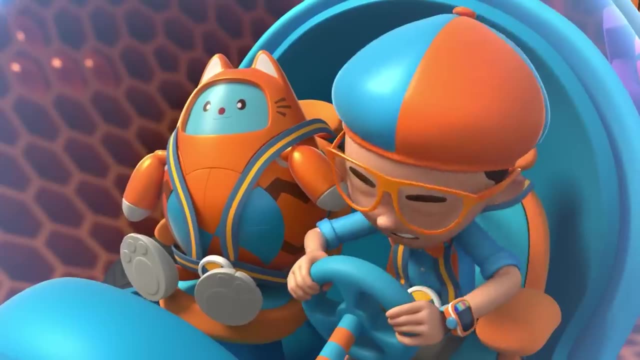 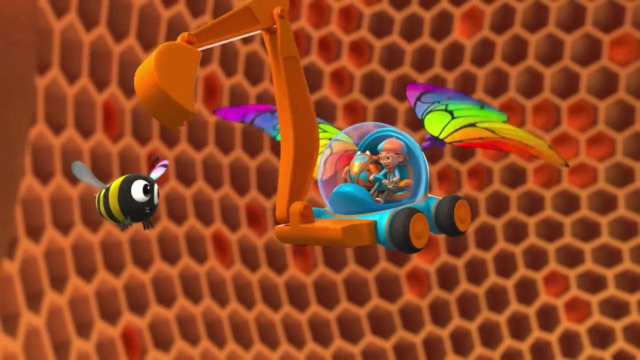 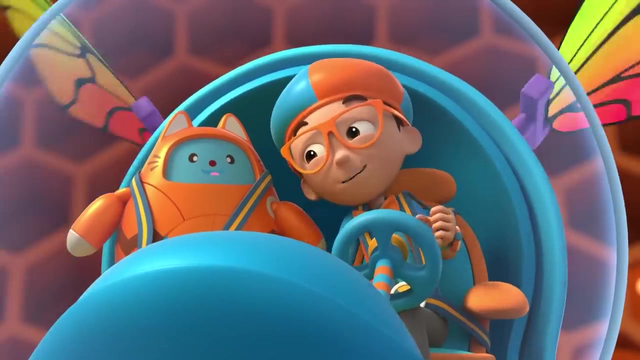 Yep, We store the honey in the honeycomb. Maybe I can taste some honey. Oh dear, This may look funny, but flapping our wings is how we make thicker honey. It's a bee thing. Whoa, Yes, Tabs, I have the answer. 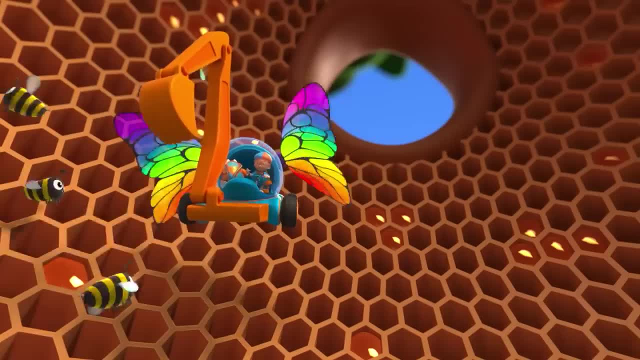 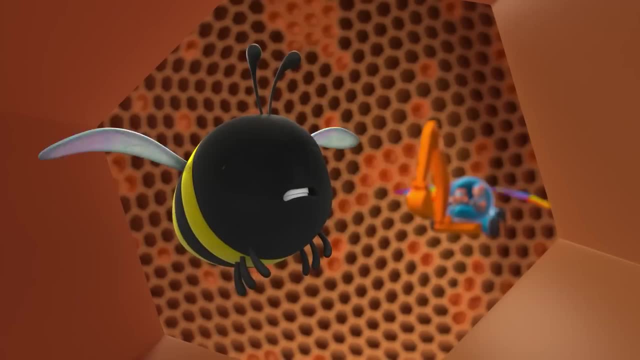 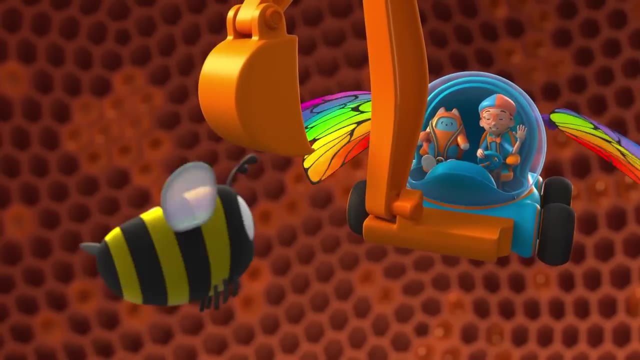 to my question. How do bees make honey? They get nectar from flowers, chew it, store it in their stomachs, then put the honey in a honeycomb and flap their wings over it. Upload the answer Tabs Bye Beejon. 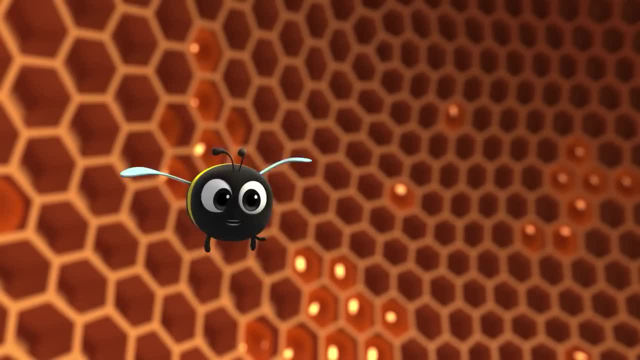 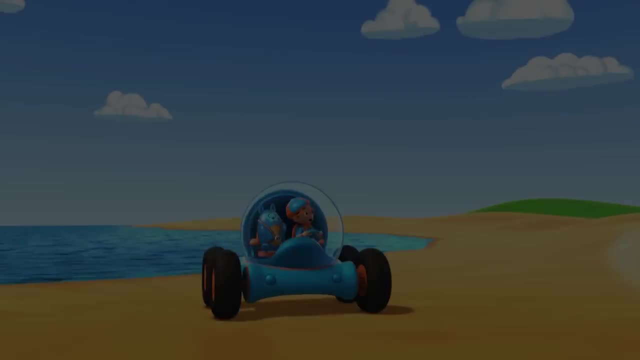 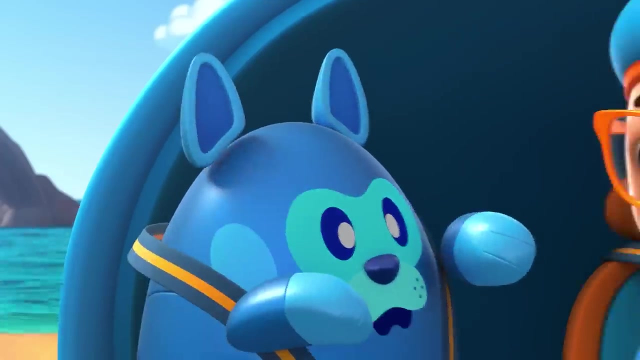 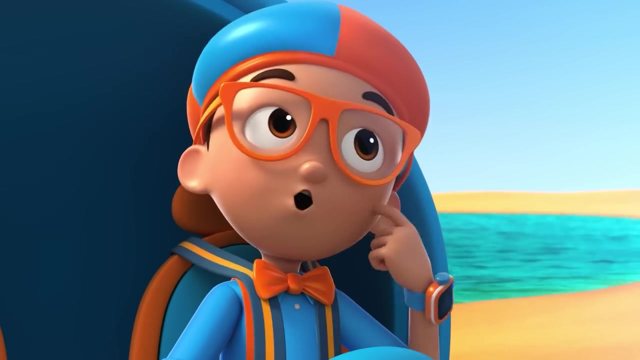 Thanks for bee-ing you Bye. Woo-hoo, Yeah, Holy smokes, A volcano. That's right, Debo. When a volcano erupts, smoke and hot lava come out the top of it. Hmm, I wonder what makes a volcano. 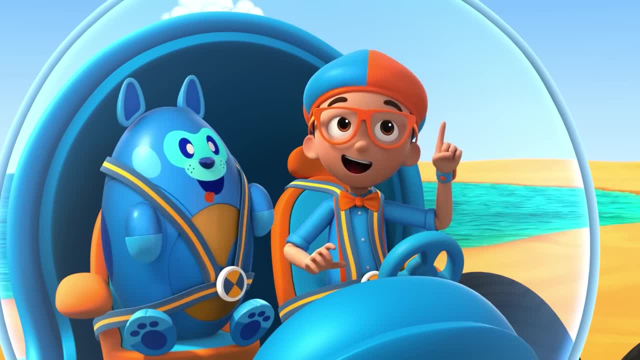 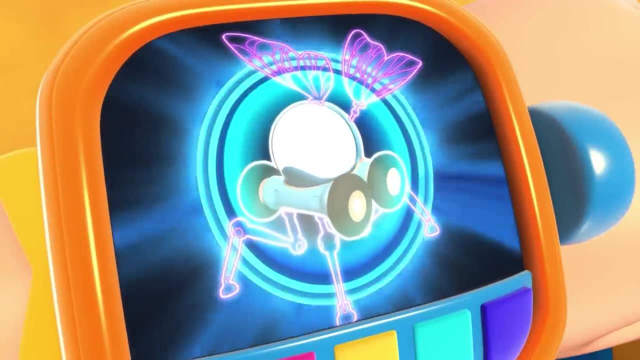 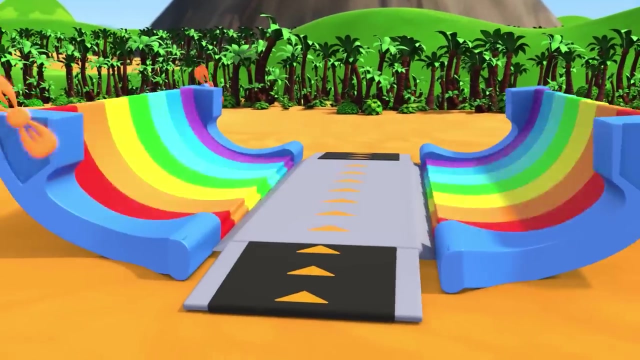 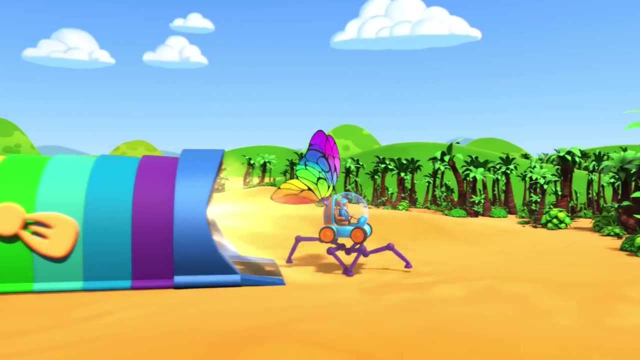 erupt. Great idea. We'll go inside a volcano and find out. I'm gonna need wings, spider legs and the heat shield. Wings, spider legs, heat shield confirmed. Activate Flippy Station. The Flippy-mobile is ready for adventure. 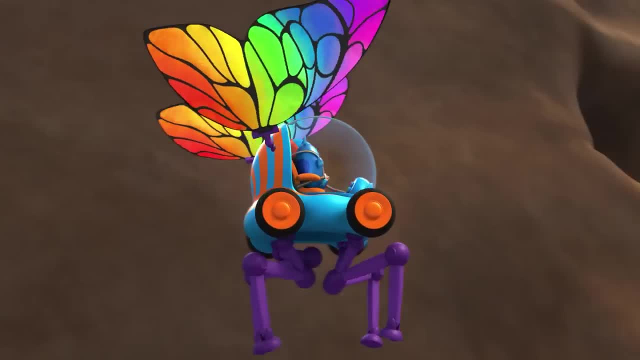 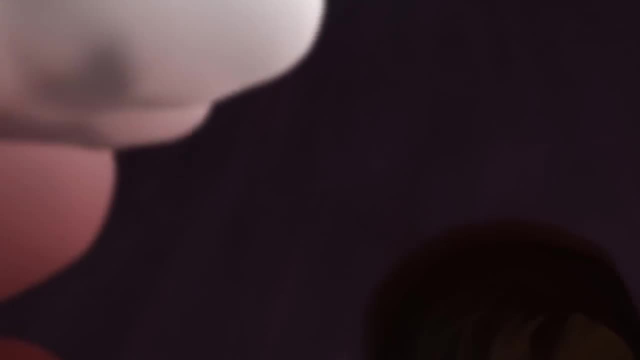 Let's go through the side vent into the volcano. Let's go through the side vent into the volcano. Whoa-ho-whoa, Whoa-ho-whoa, Whoa-ho-whoa. It sure is hot in here. 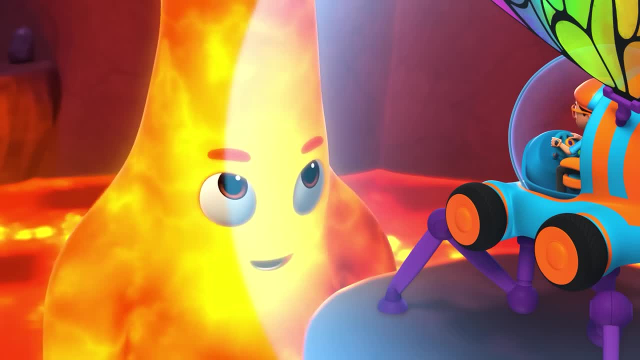 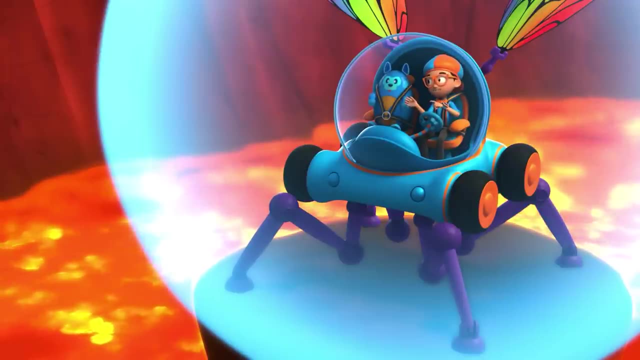 Whoa-ho-whoa, Whoa-ho-whoa, Hey there, I'm Maggie the Magma Monster. Hey, it's me Flippy, and this is Debo. We want to learn what makes a volcano erupt. 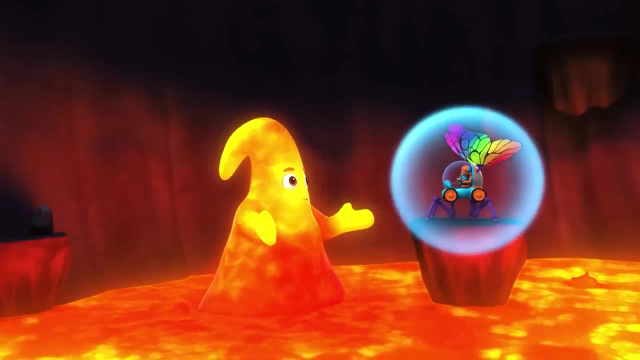 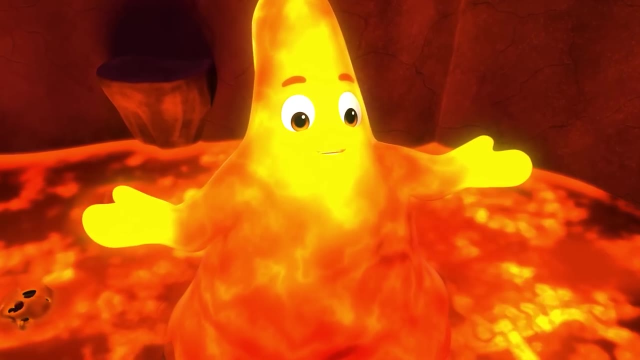 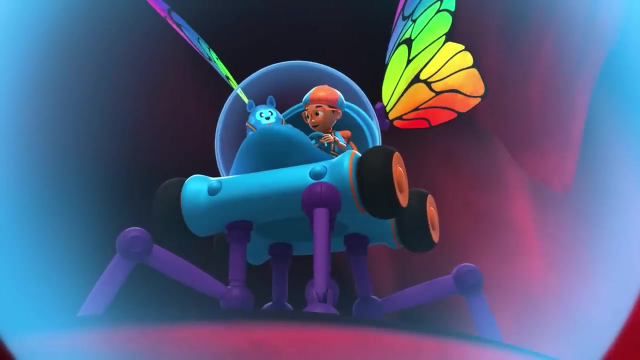 You're in for a real treat, Flippy and Debo. Speaking of treats, Whoa-ho, Below us, deep in the Earth, the planet's heat is melting rocks into liquid, also known as magma. like me, You're right, Debo. 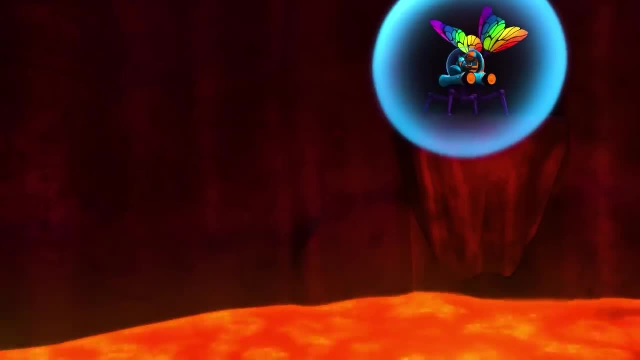 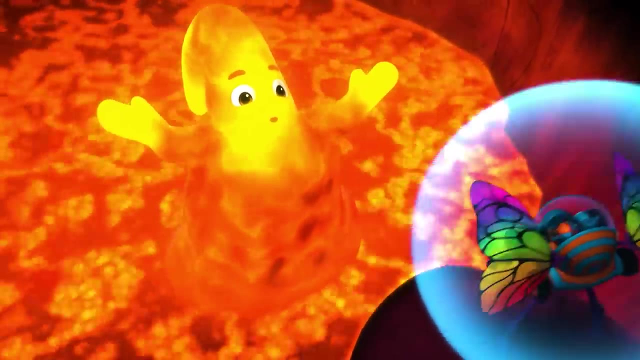 It IS like one of our favorite games. The floor is lava. Whoa-ho. Magma becomes lava after it erupts out of the volcano Whoa, So I guess I'm the floor. Whoa-ho-ho, We're getting. 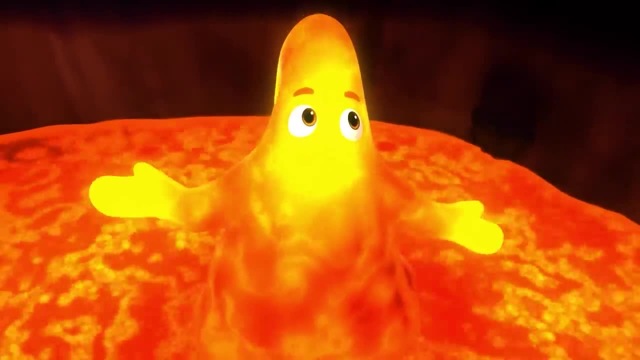 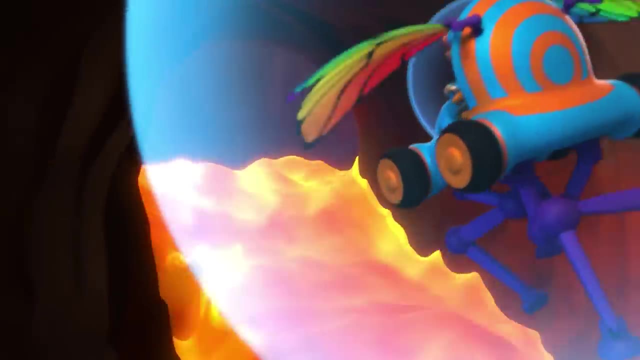 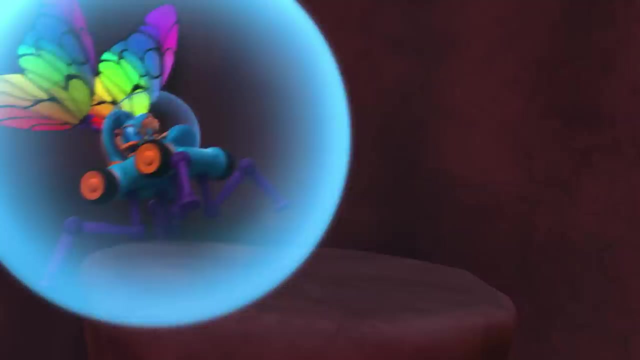 higher. That's because the more rocks melt below, the more magma rises here in the chamber. Hey, I wonder where this goes. Look out, Flippy Magma. Phew, That was close, Maggie. you almost filled the whole cavern. 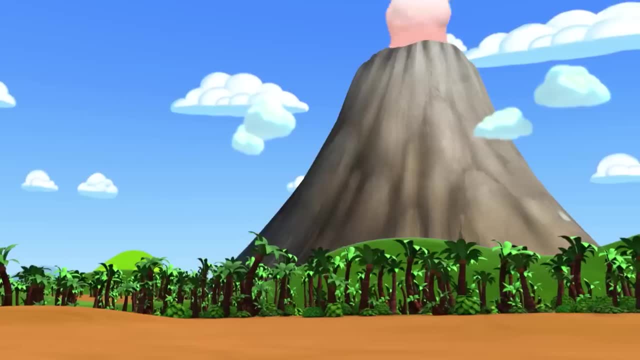 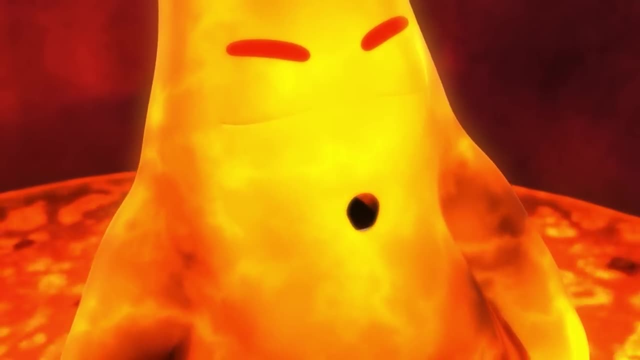 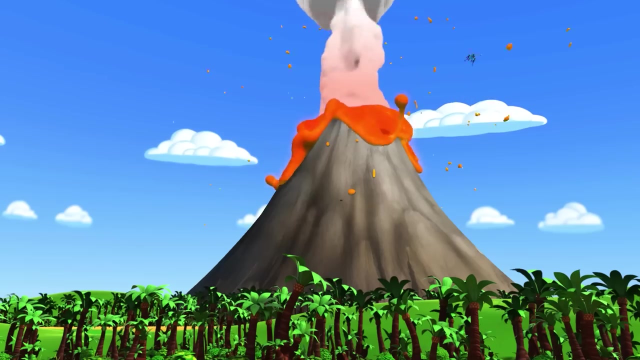 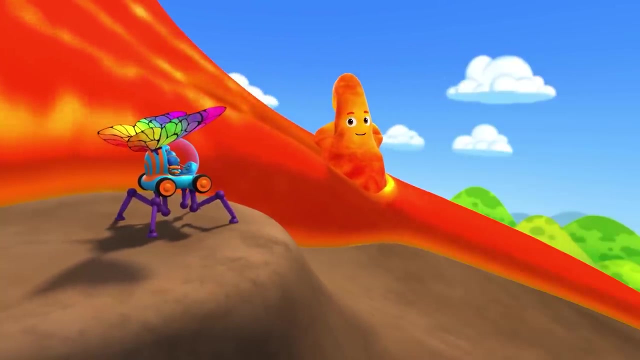 now? I sure do, And as I throw the pressure inside, the volcano builds Until we push through the crust or the top of the Earth. Hold on, Whee, Ah, Much better, Maggie, What a blast. And I got. 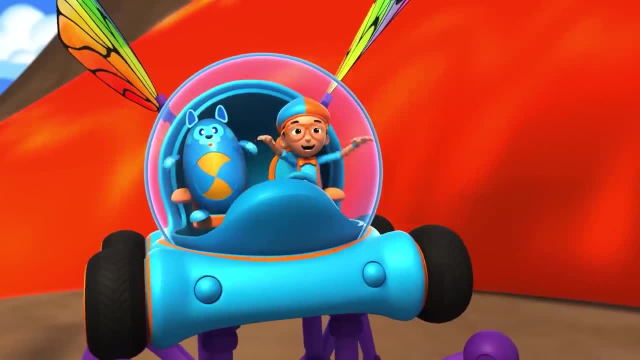 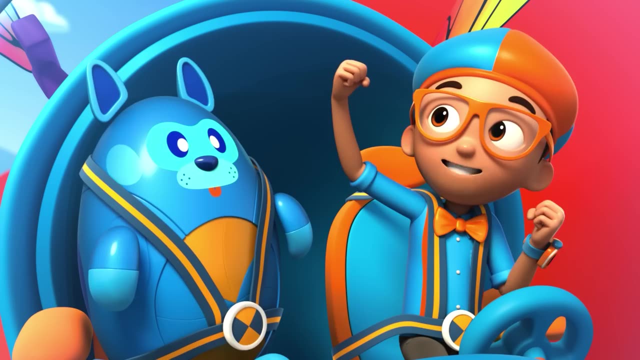 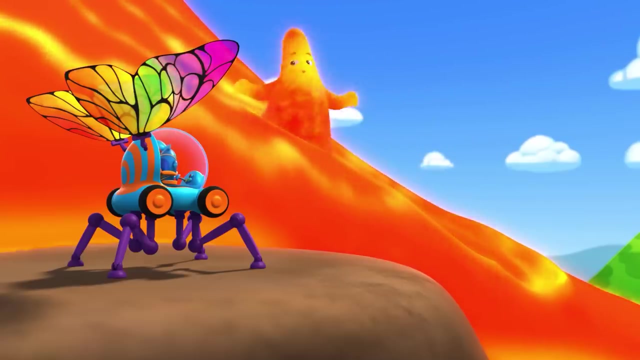 the answer to my question: What makes a volcano erupt? A volcano erupts when the hot magma inside it builds pressure and bursts through the surface of the Earth. Upload answer. Deebo, That was fun, Flippy. Hope you loved it. 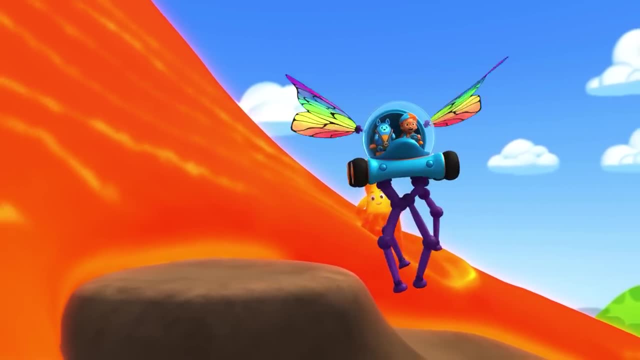 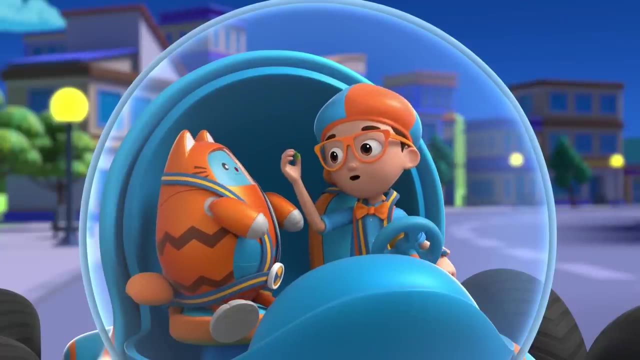 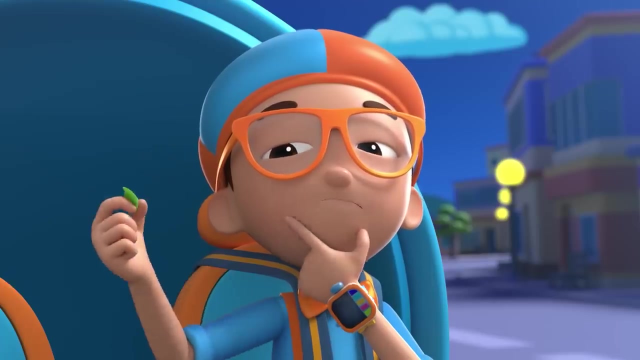 We did Bye-bye Maggie Salad. Oh, thanks, Tabs, Didn't know. this lettuce was stuck in my teeth. I guess a toothbrush would help. Hmm, I wonder: how do you use a toothbrush to clean your? 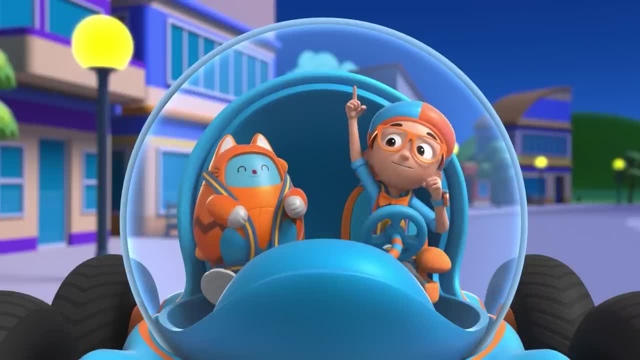 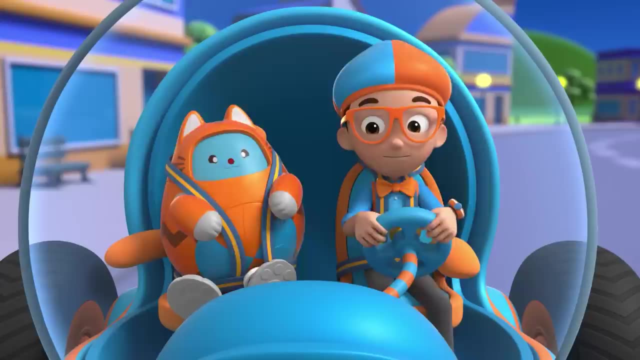 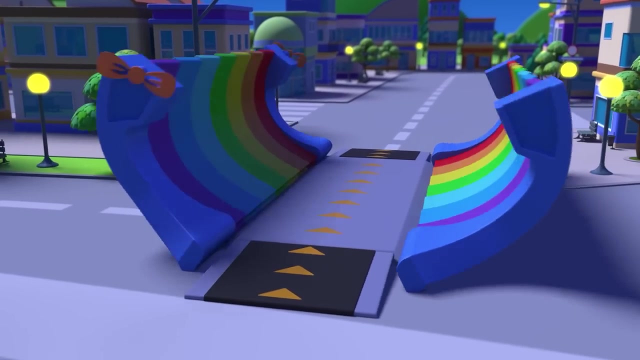 teeth. Great idea: We can go meet a toothbrush in a mouth. I'm gonna need wings- Wings, confirmed. Let's go explore. Activate Blippi Station. The Blippi-mobile is ready for adventure. It's time to shrink down and go into a mouth. 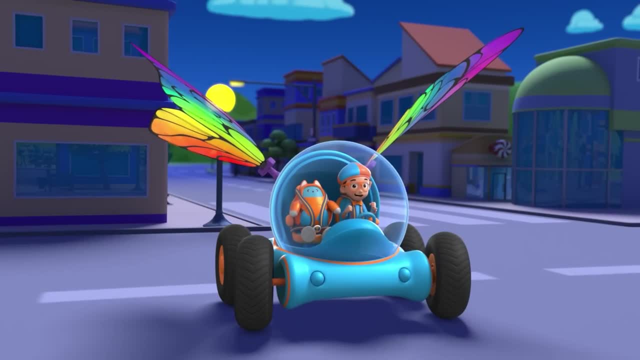 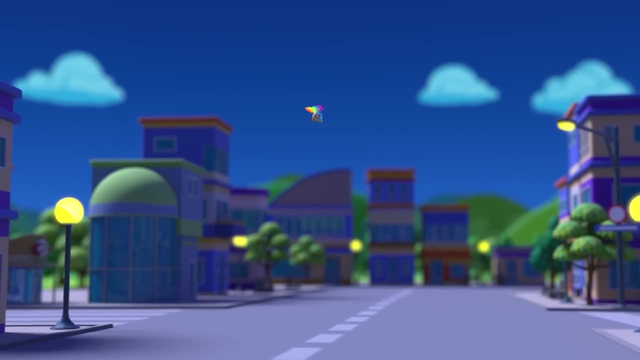 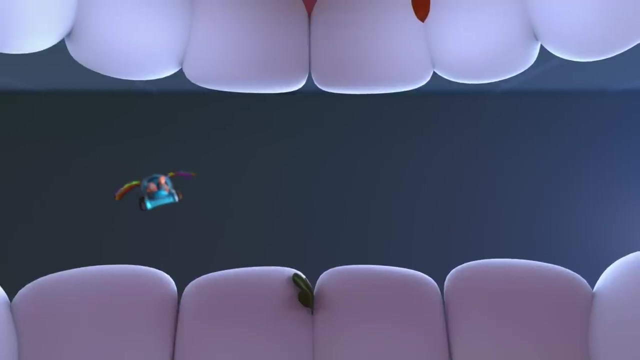 Shrinking down. We're inside a mouth. You're right, Tabs. We need a way to clean our mouth. We're inside a mouth. We're inside a mouth, You're right, Tabs. We need a way to clean these teeth. 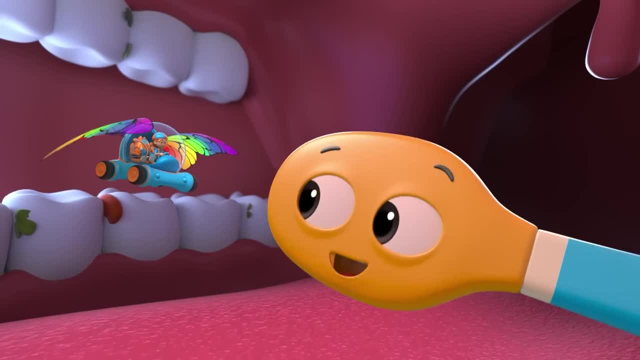 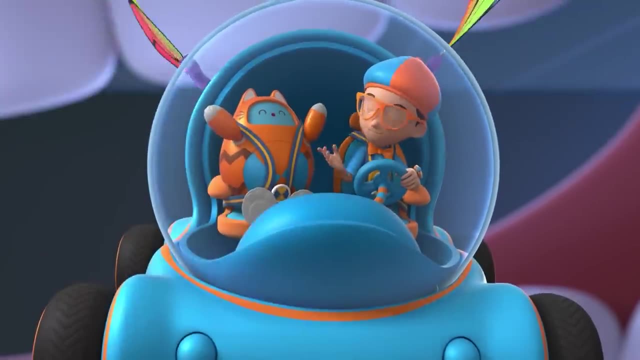 Would a brush help? Hi, I'm Bill Brushy And you are. Hey, It's me Blippi, And this is Tabs. I want to find out how to use a toothbrush to clean teeth. Well, you're asking the right. 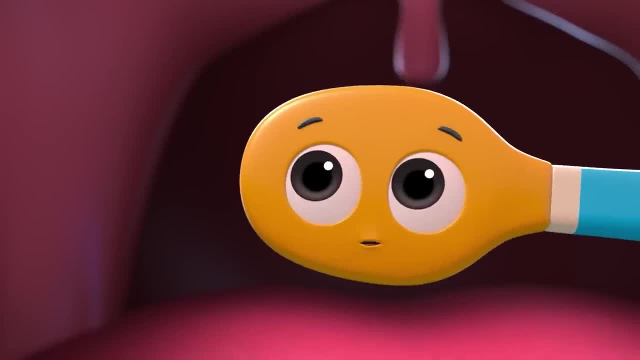 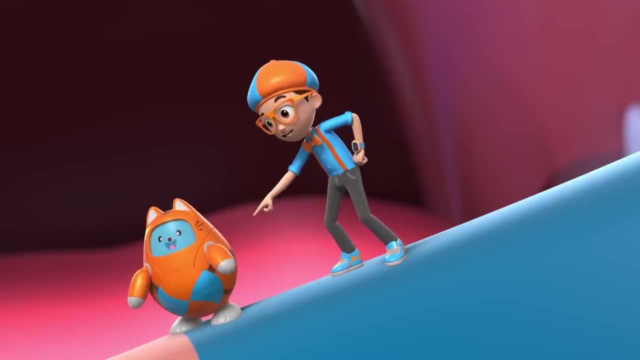 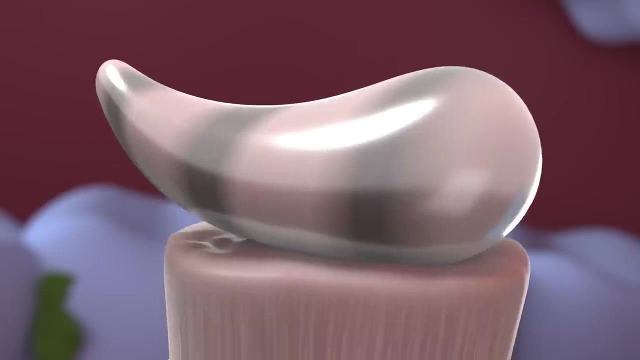 brush. Hop on and I'll show you the best way to clean your teeth. Alright, Hey, Bill Brushy, Is that toothpaste on your brush part? Yes, sir, It helps keep teeth healthy and food-free. Okay, now here's how to brush your teeth. 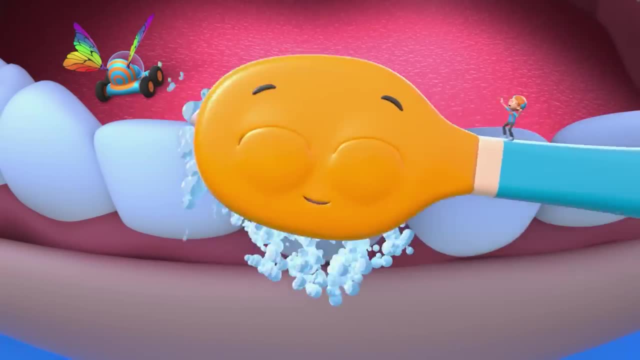 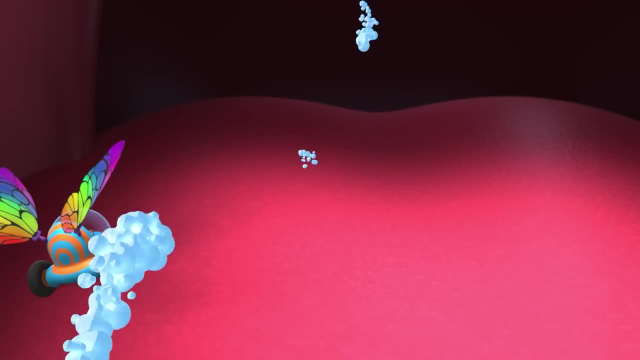 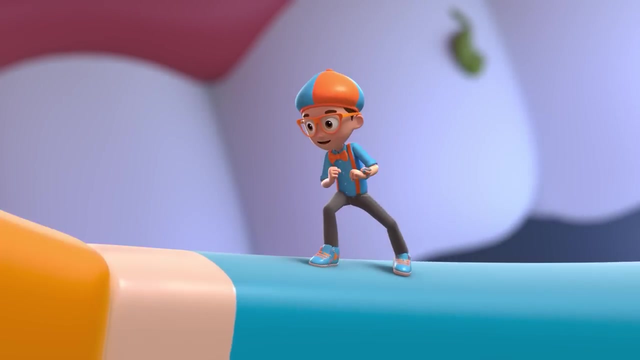 Let's go to the front first. So small circles on every tooth. Okay, That's the front done, Let's go to the back. now We turned, We flipped Little circles round and round. Let's make some more Circles, Circles, Circles. 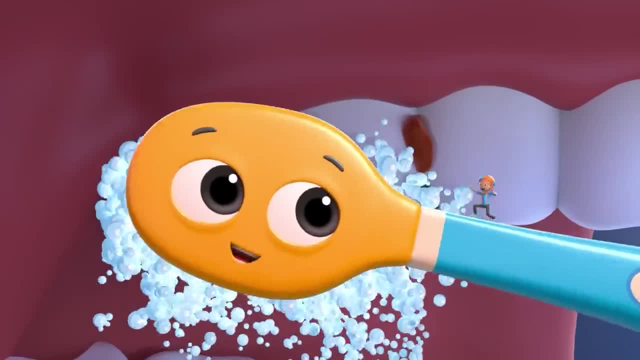 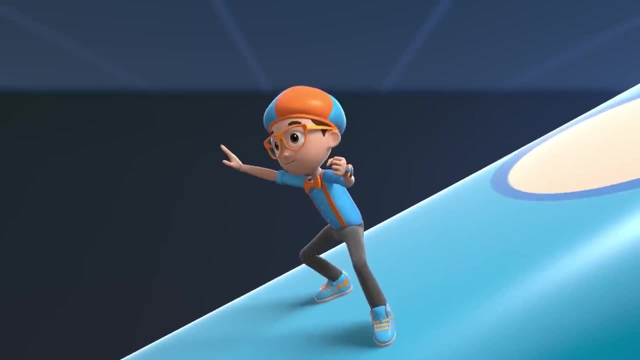 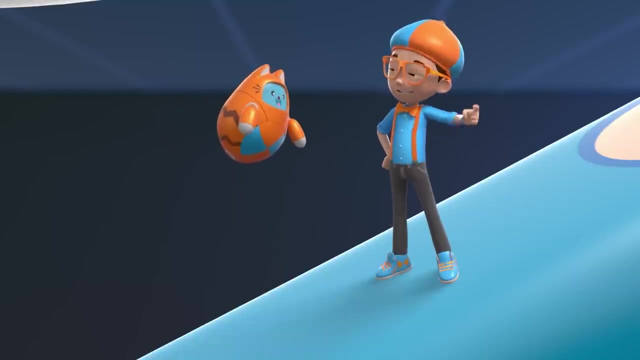 These teeth are the molars. I call them the Chew Crew, Since they do most of the work. I know Tabs. Toothbrushing is a wild ride. Wow, I think I have the answer to my question. How do you use a toothbrush to clean your teeth? 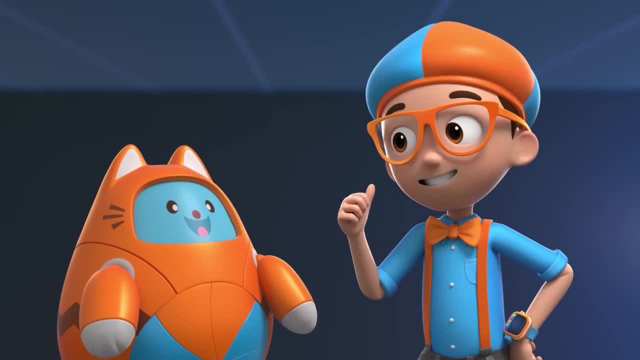 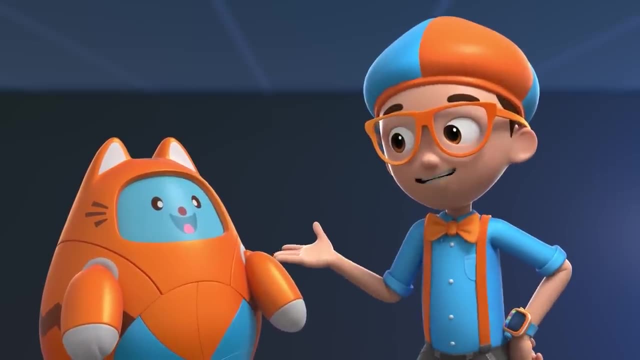 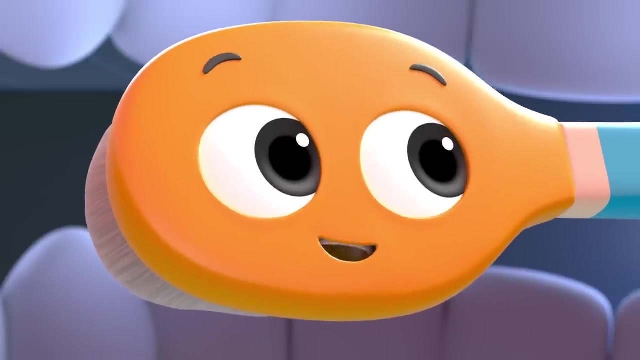 It cleans by brushing the front, back and in-between of all teeth in little circle motions And that pushes all the food out from between the teeth and makes them nice and clean. Upload- answer Tabs. Thanks for your help, Blippi and Tabs. 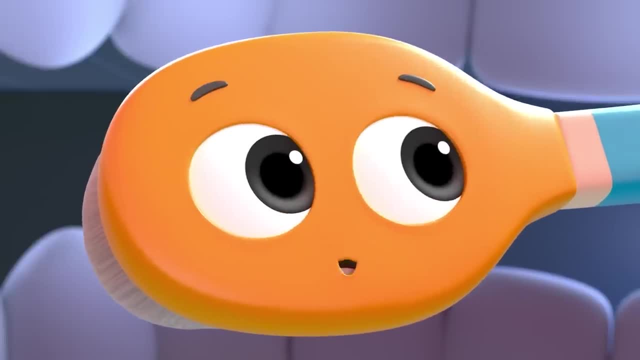 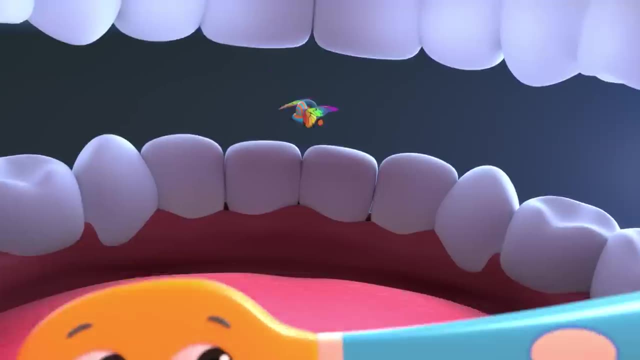 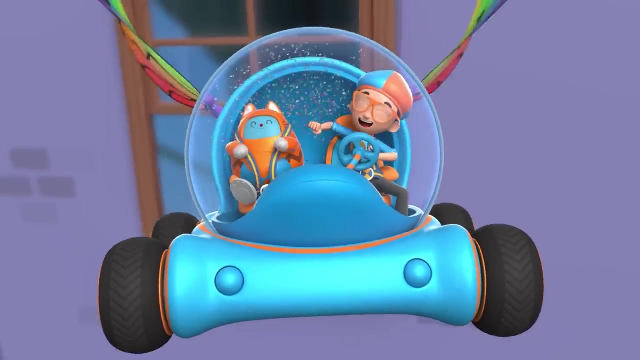 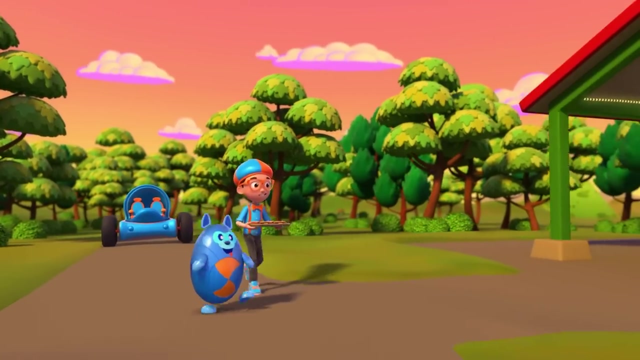 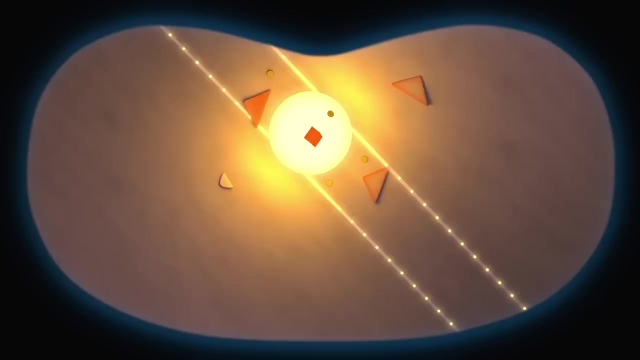 Remember to brush twice a day for two minutes each time for super sparkling teeth. We will Thanks for letting us ride along Brushy. Bye-bye. Yum, These turkey sandwiches are going to be delicious. Oh, What a mess. 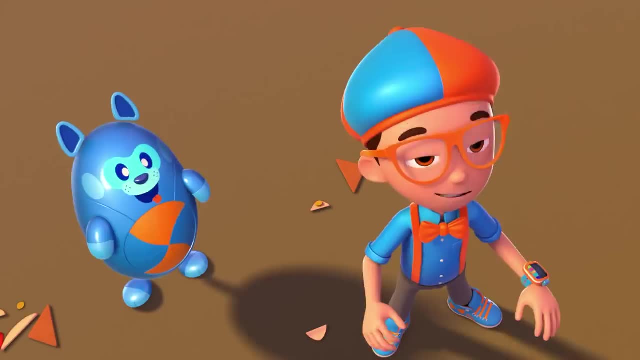 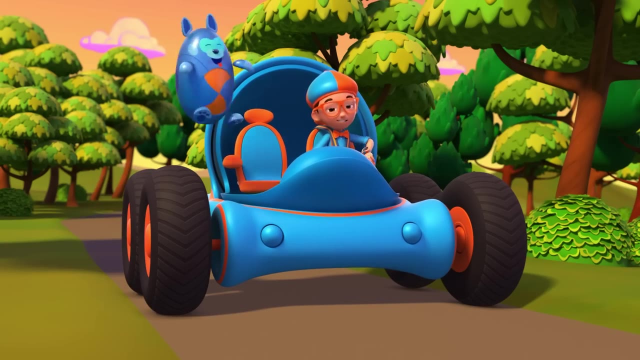 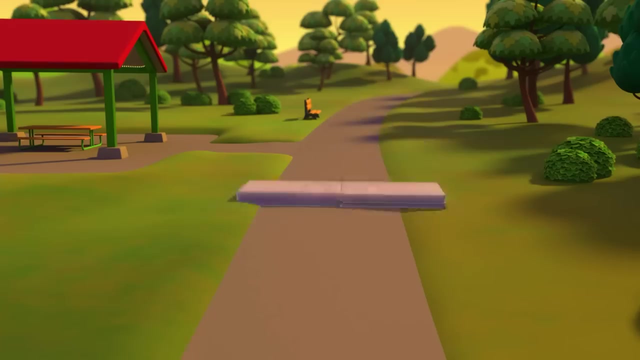 Hey, Look at that fly walk on the ceiling. Hmm, I wonder How do flies walk on the ceiling? I'm gonna need wings and spider legs. Wings, spider legs, confirmed Activate Blippi Station. Shrinking down, Shrinking down. 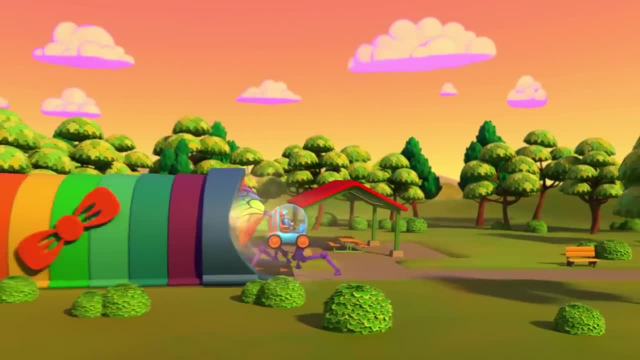 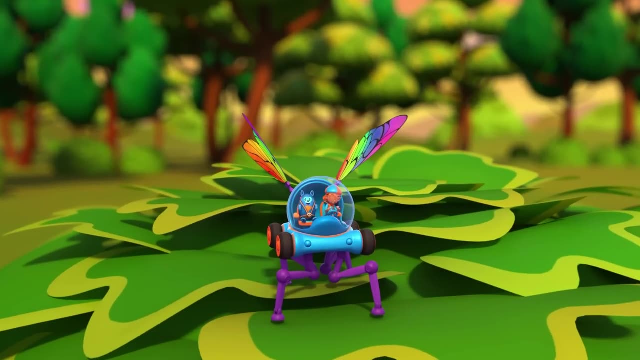 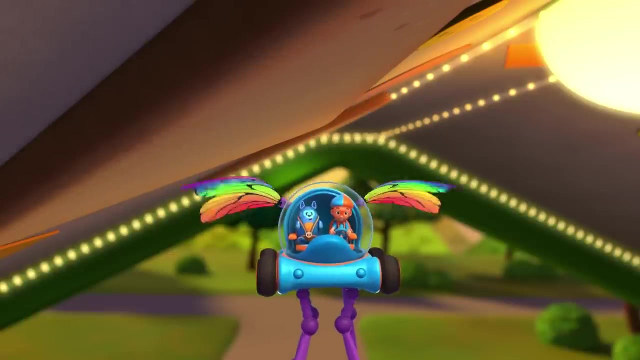 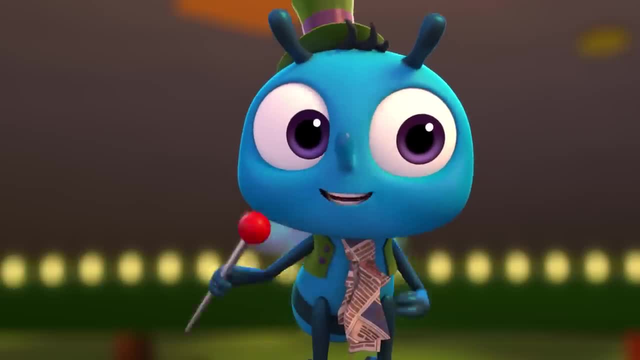 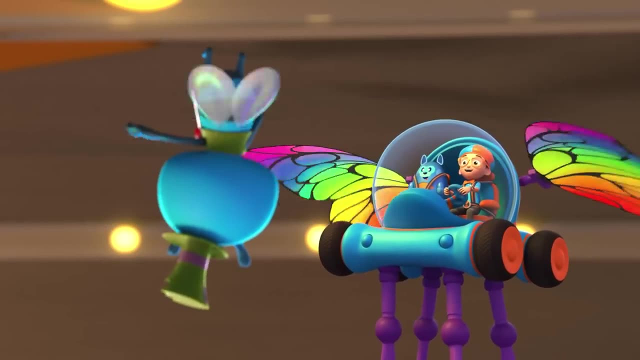 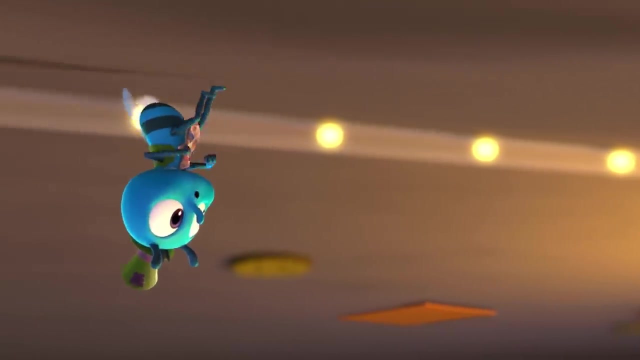 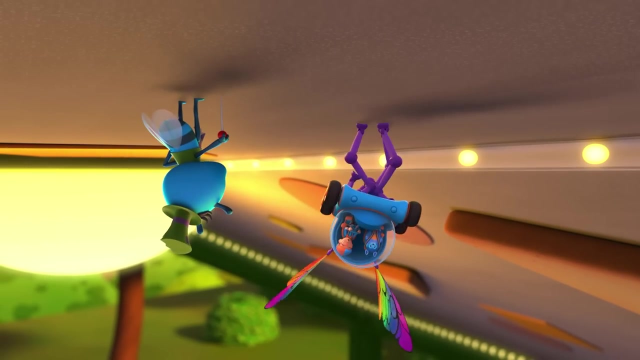 How did you get on the ceiling? Oh, it's easy. Watch this Ta-da. Wow, Yes, sirree, The ceiling is my own personal dance floor. Now you try. Here goes Whoa, Why can't the Blippi-mobile? 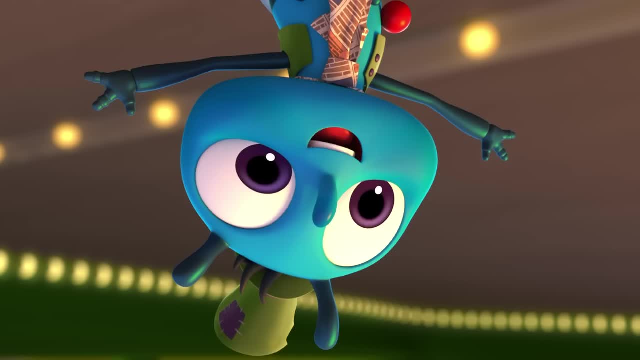 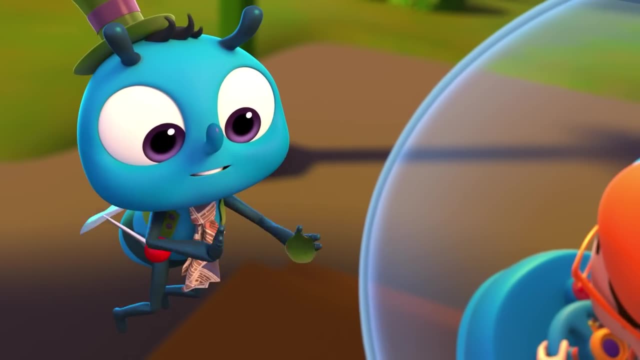 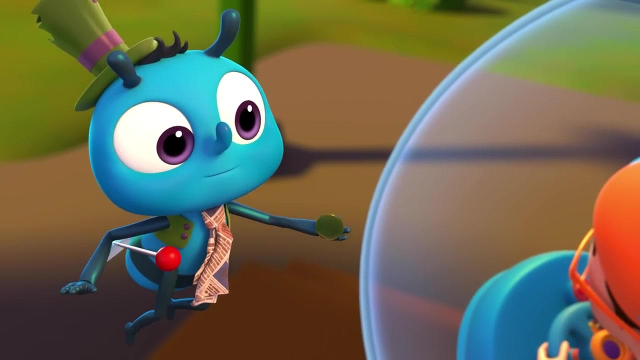 stand on the ceiling too. What's the trick? Here's the trick: Stick, Stick, Mm-hmm. You see my feet make a super sticky glue that helps me stick to the ceiling Here. try some. Don't mind if I do. 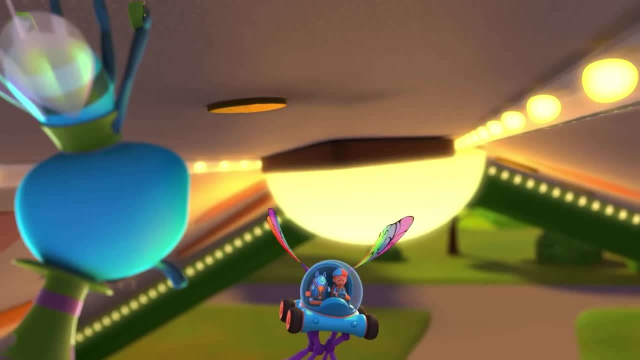 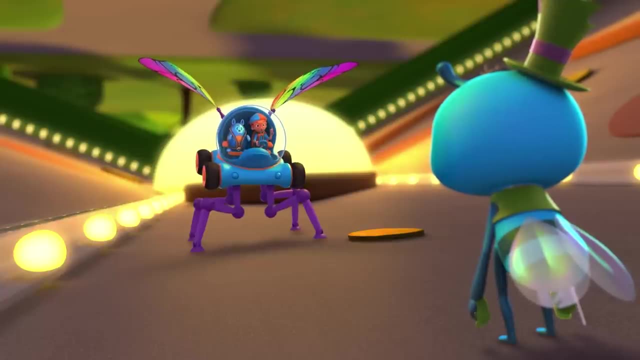 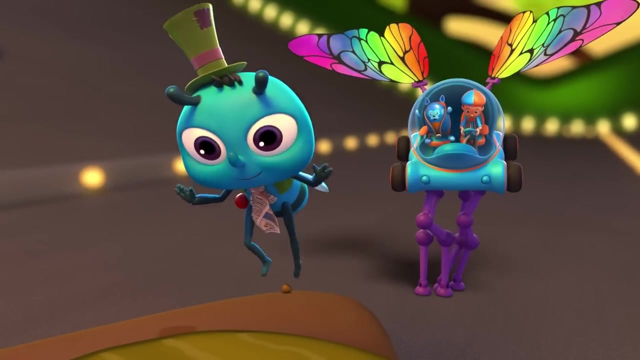 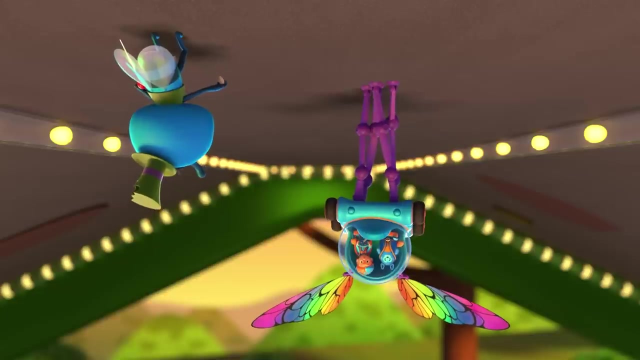 Here goes Whoa, Whoa. Now I stick to the ceiling too. Look at all that mess. Oh, The glue has us stuck in place. That's because you're not doing the fly leg twist, The fly leg twist. 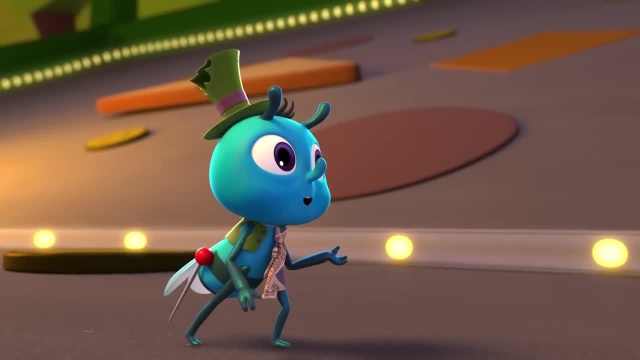 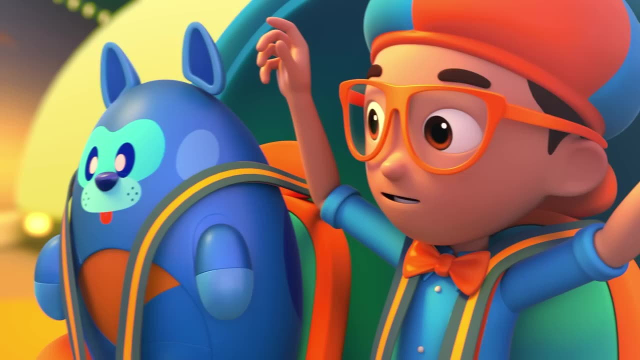 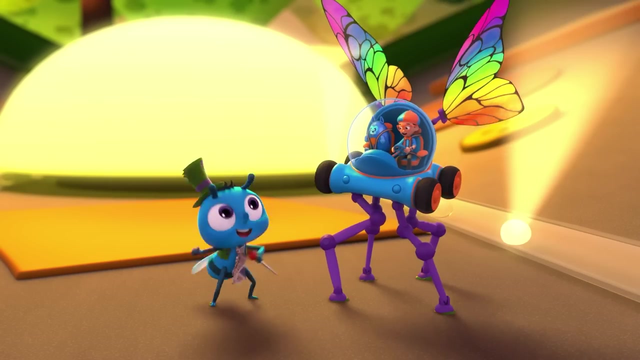 That's right. Fly glue is so strong that we have to push ourselves off the ceiling to walk Like this, Like this. You got it, Now let's hit it. Do the fly leg twist. Do the fly leg twist. Get your feet unstuck. 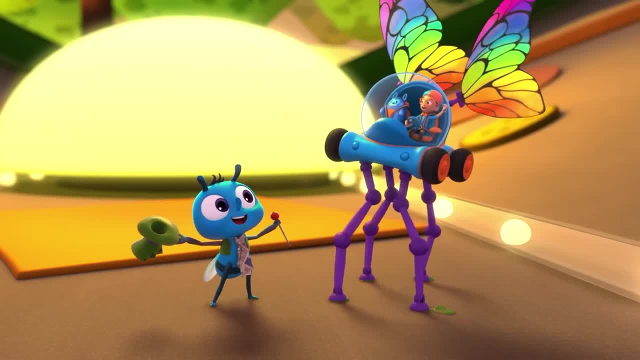 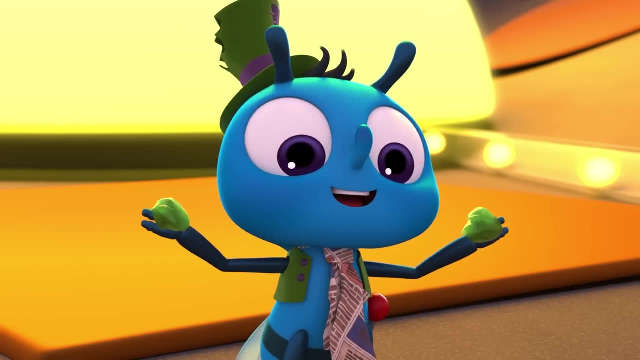 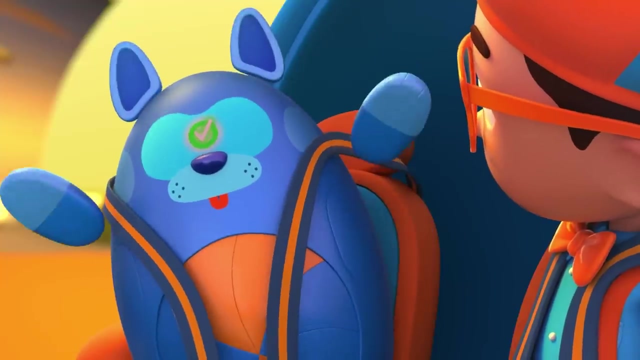 when you go like this. We did it And I have the answer to my question: How do flies walk on the ceiling? Fly legs have a special sticky glue that keeps them stuck to the ceiling. Upload answer. Deebo, Well, I'm off to eat. 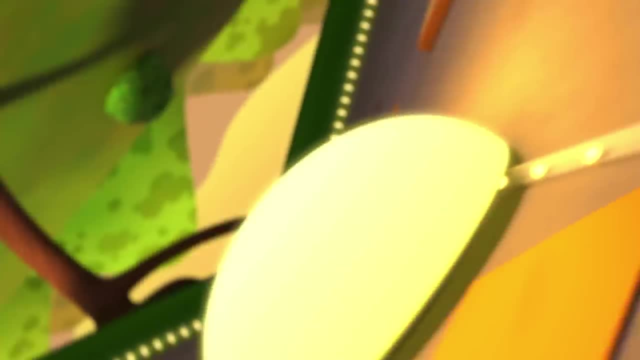 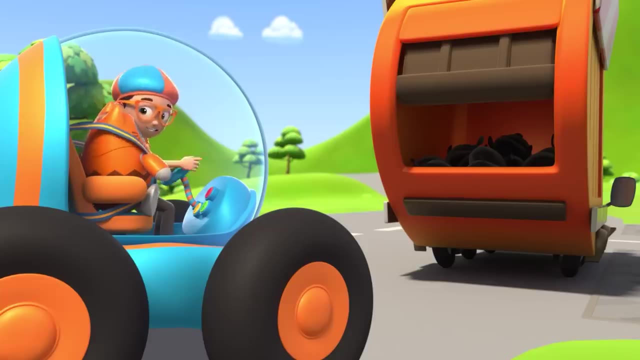 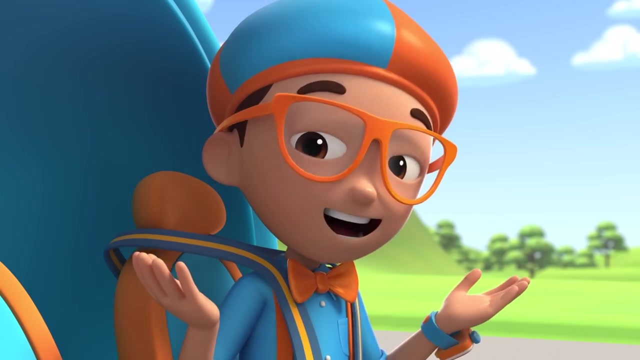 a little bit of dinner now. See you later. Blippi, Buh-bye. Hey, It's a garbage truck. I can see it and smell it too. Wow Tabs, Even you think it's stinky And you're a robot. 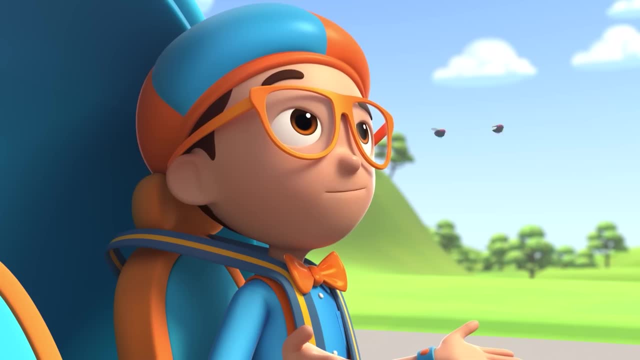 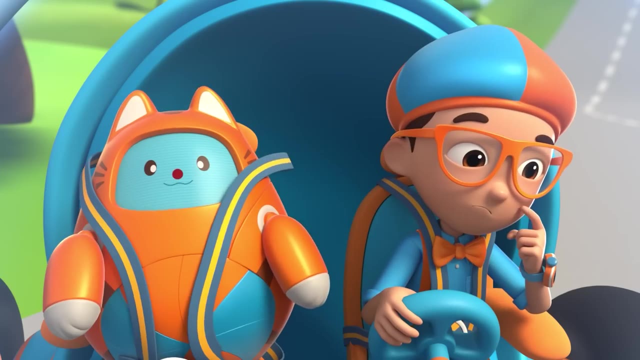 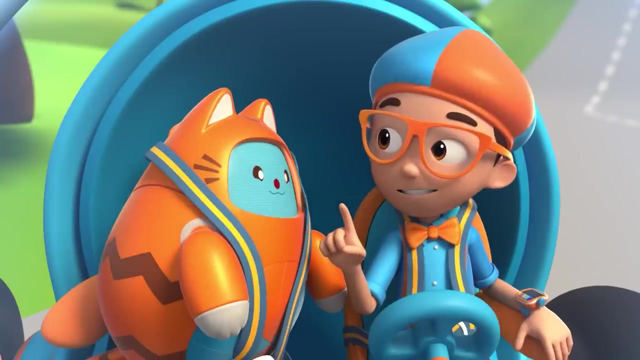 Wait, Where's that buzzing sound coming from? Oh, Flies. Hey, Those flies just flew into the garbage truck. Hmph, I wonder, why do flies love garbage? Good idea, Tabs: We can go into the garbage truck to find out the answer I'm gonna need. 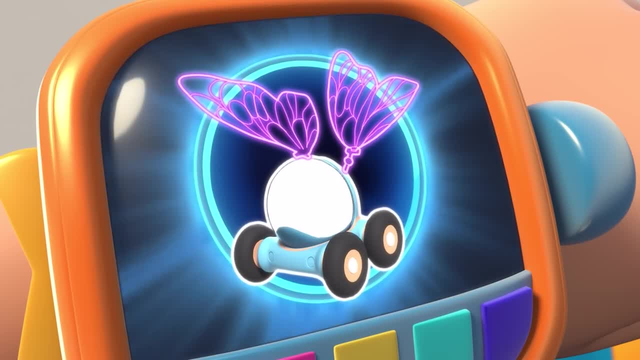 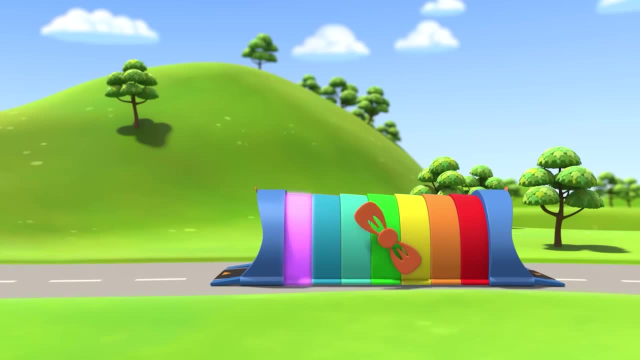 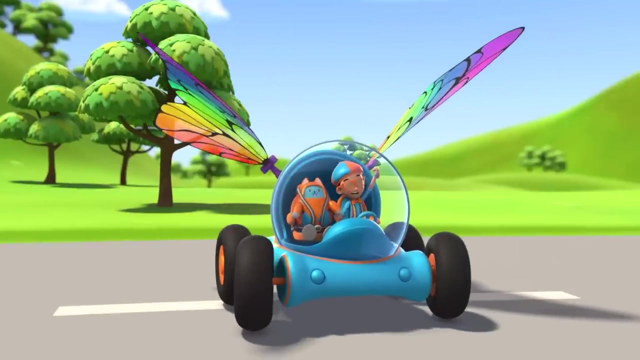 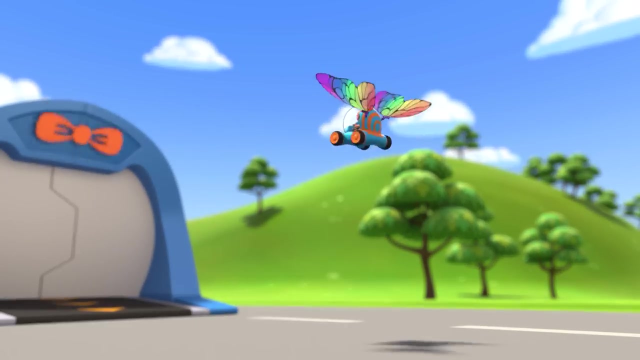 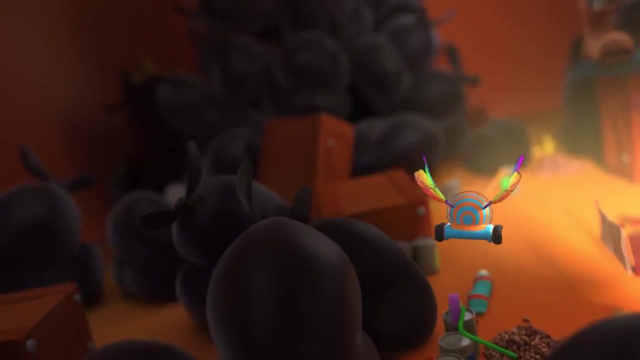 wings, Wings confirmed. Activate Blippi Station. The Blippi mobile is ready for adventure. Let's go find out why flies love garbage Shrinking down. Hold your breath, Tabs, We're going in, I'm in the garbage truck. 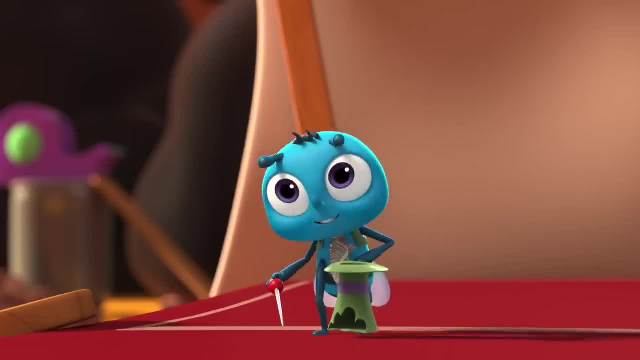 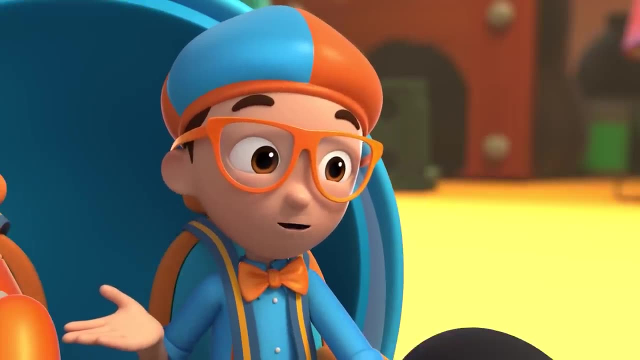 Welcome, I'm Horace. the Fly Looks like your first time here. hm Hi, Horace, It's me Blippi. This is my first visit to a garbage truck. Little stinky huh, Oh, Not for me. 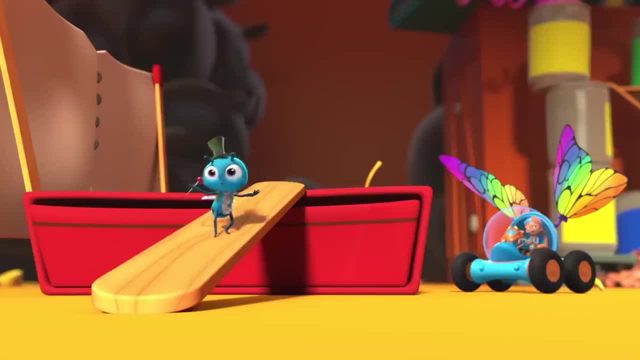 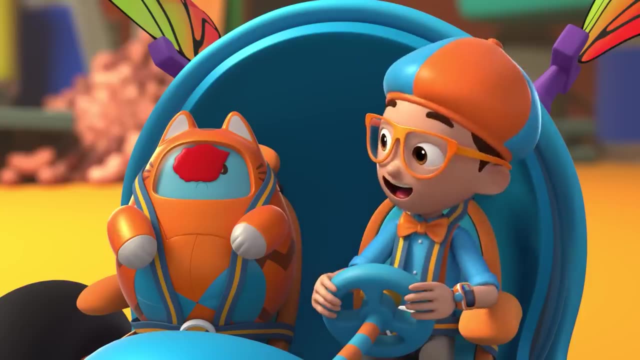 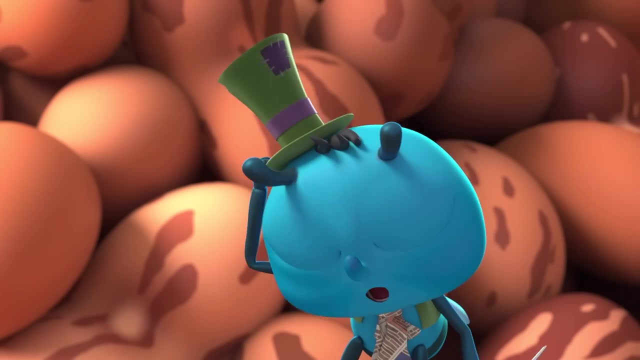 I love smells. Follow me, I'll show you around. This place is like my playground. Ho ho, Shoot me Whoopsies. Sorry about that, Hey, Horace, Why do flies love garbage? Because it's delicious and garbage. 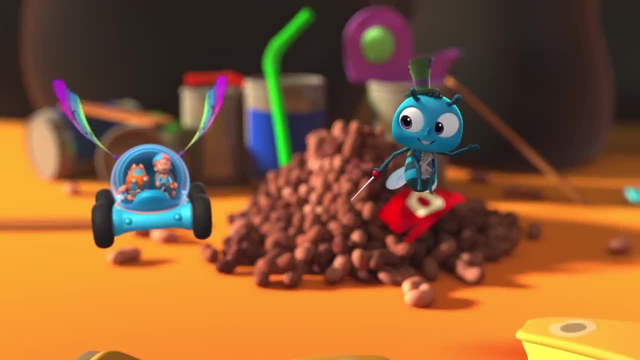 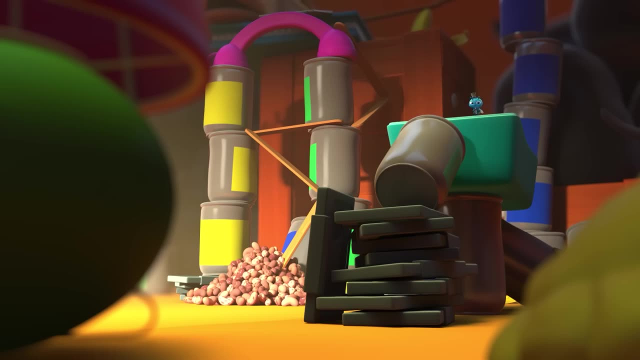 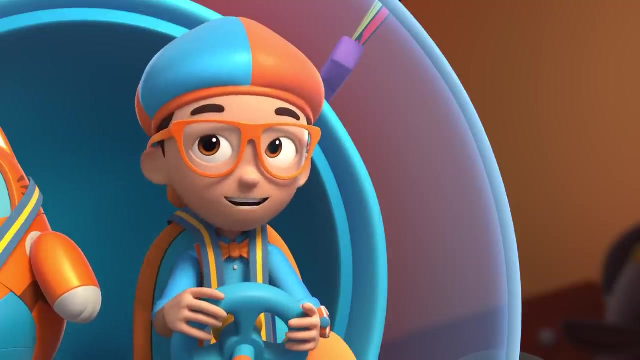 makes me fly. We've got stinky beans, moldy cheese, greasy pizza boxes and even leftover mush. Sorry, Must have been the beans. I could give you a ride to the nearest garden or fly restaurant. Horace, Where are you? 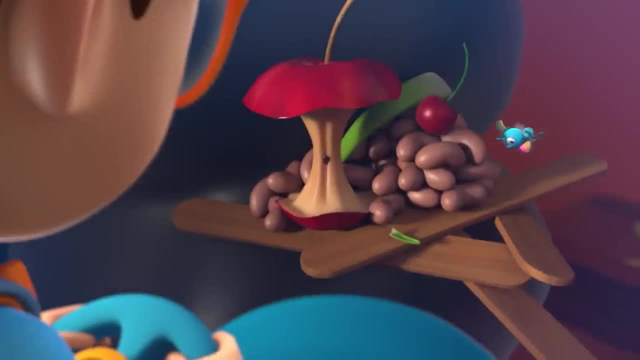 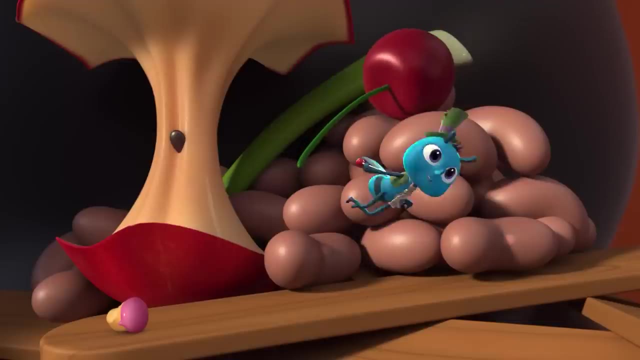 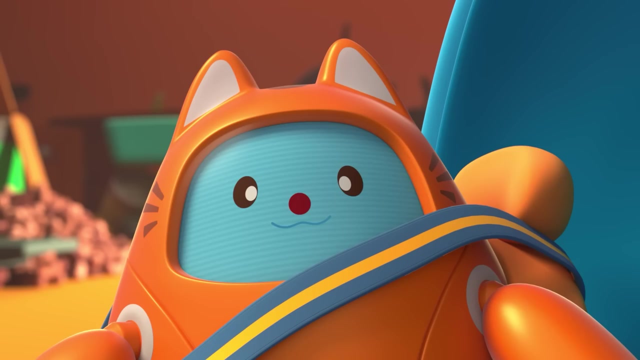 Everything's coming up Garbage. Oh, is that cake? Oh, no, that was not cake. Still good, though Gotta dash and eat all the trash. Horace has more energy now, Aha, Which means I think I have the answer to why flies. 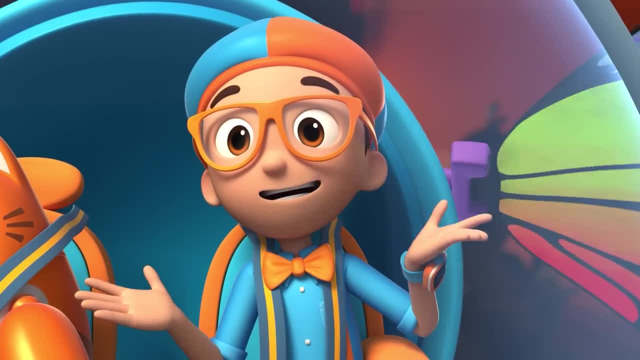 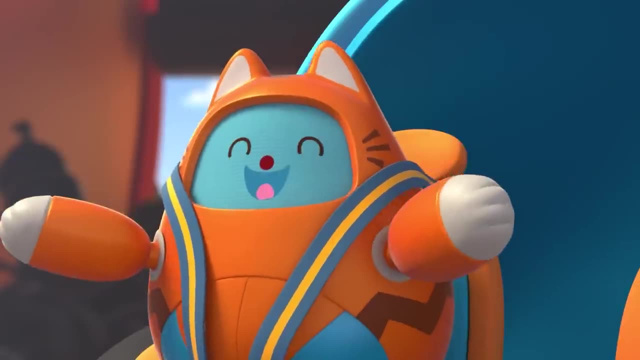 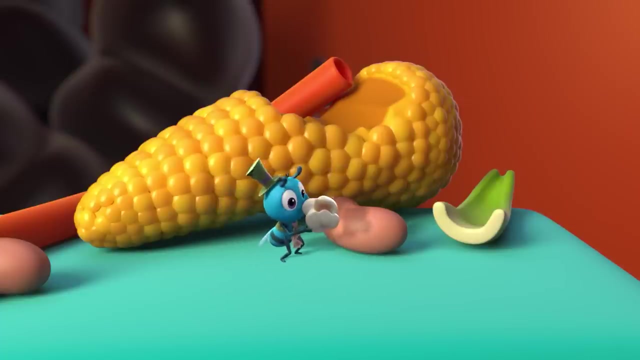 like garbage. It's because they love the smell and they find food there. That's so silly. Upload answer tabs. Yes, sir, Bippy, For me a garbage truck is a 24-7 all-I-can-eat restaurant. 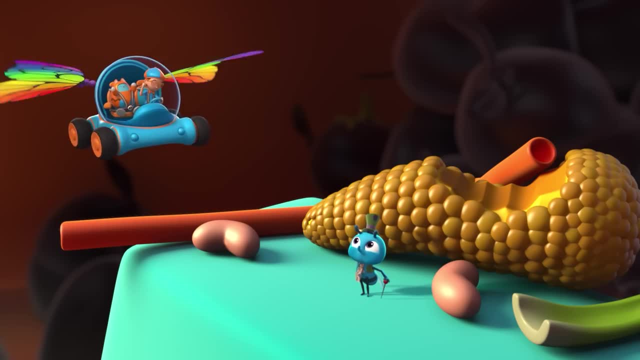 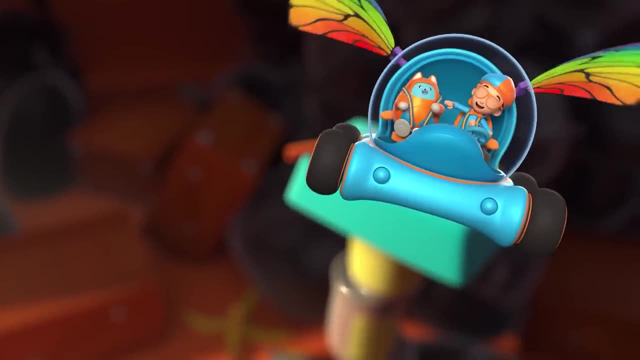 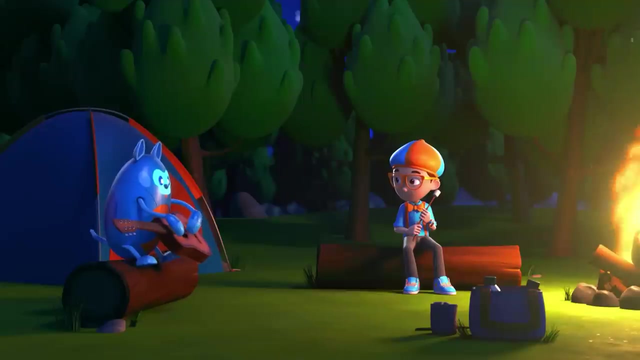 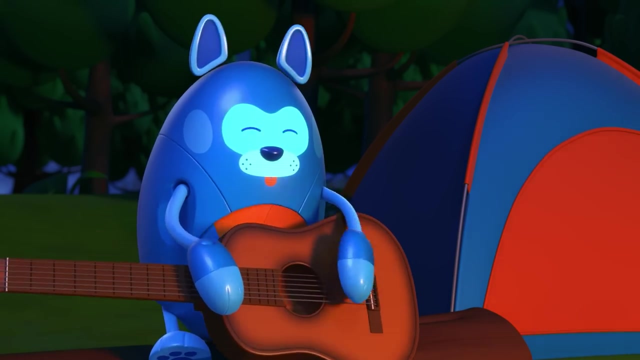 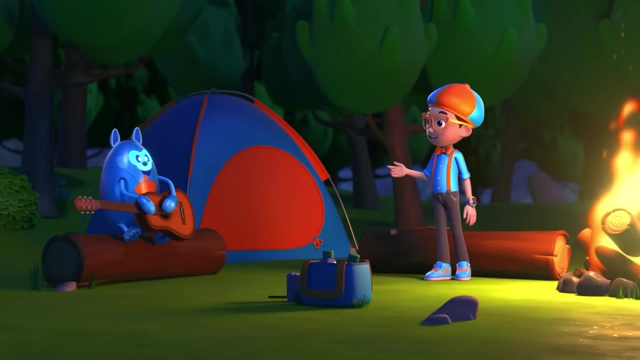 Woo hoo, Go Horace. Thanks, Cheers Blippi. Wait, I don't think your guitar is working, right, Deebo. Hmm, I wonder, How does a guitar work? You're right, Deebo, Let's go find out. 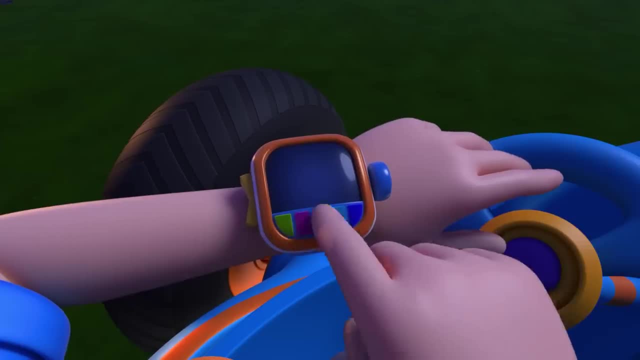 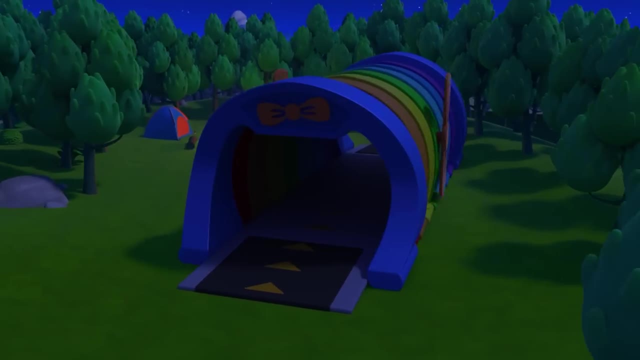 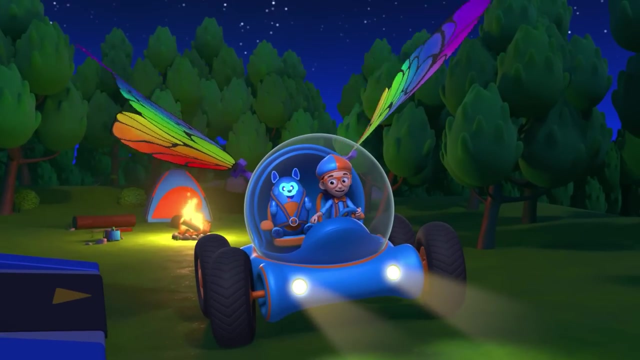 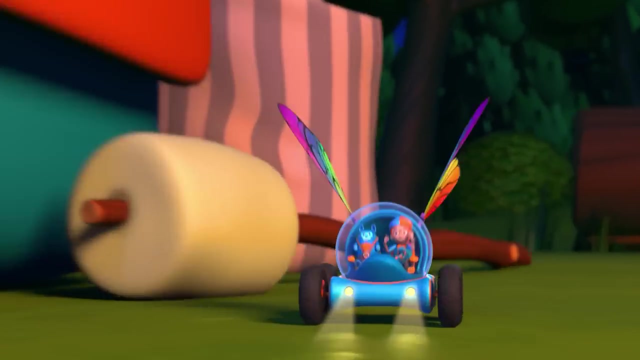 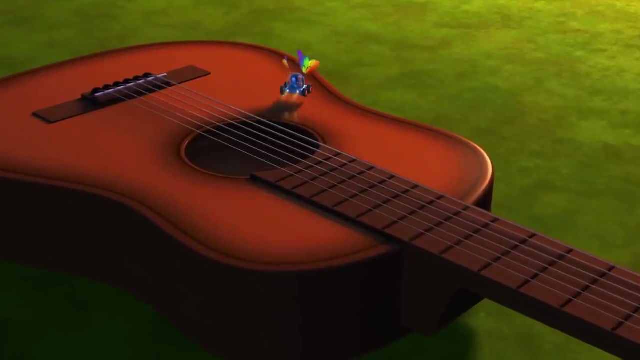 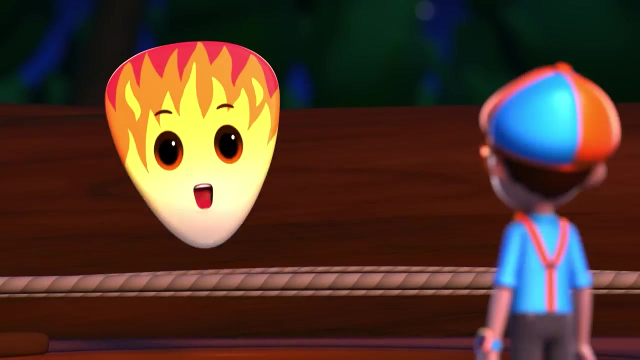 Haha, Gonna need wings. Wings confirmed. Activate Blippi Station Shrinking down. The Blippi-mobile is ready for adventure. Rock and roll. That sounded great. I love it, Thank you. Hey, It's me Blippi and this is Deebo. 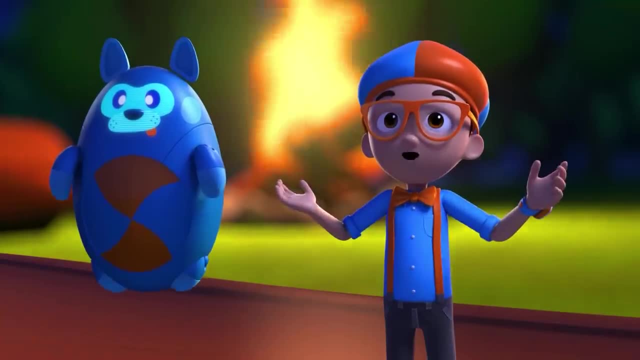 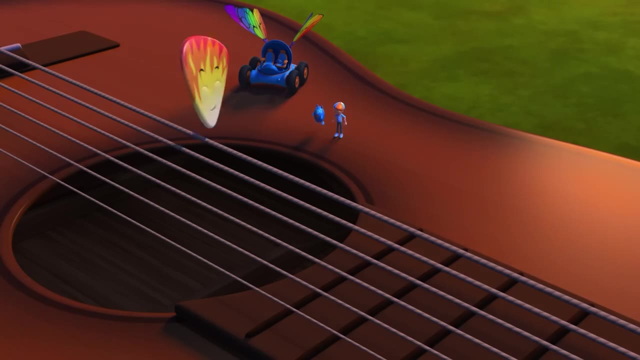 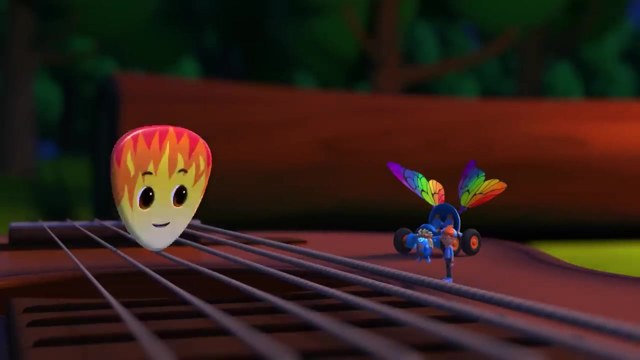 I'm picky. We were wondering how a guitar works. Can you show us? I can, but I can't work the guitar by myself. I'll need your help to play it right. Okay, When I pick a string it goes back and forth. 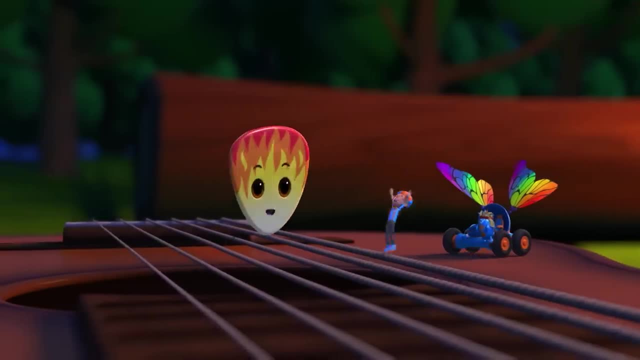 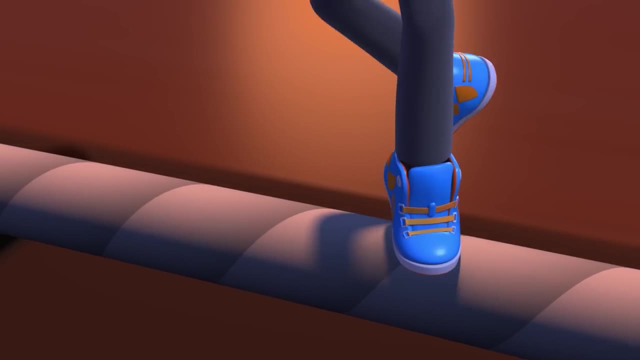 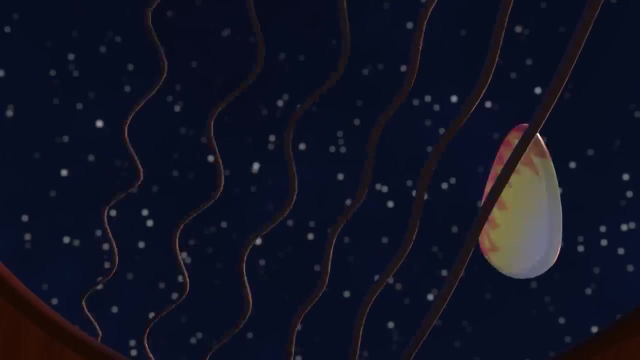 really fast, which makes a note. Whoa, You're right, Deebo. My string is much thicker than yours. I bet it's harder to balance for you. The faster the string goes back and forth, the higher the note. How do you make other? 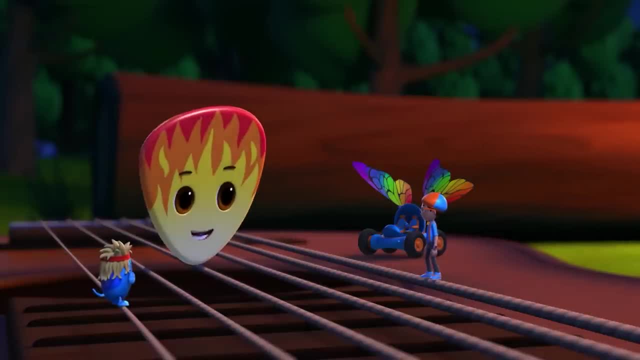 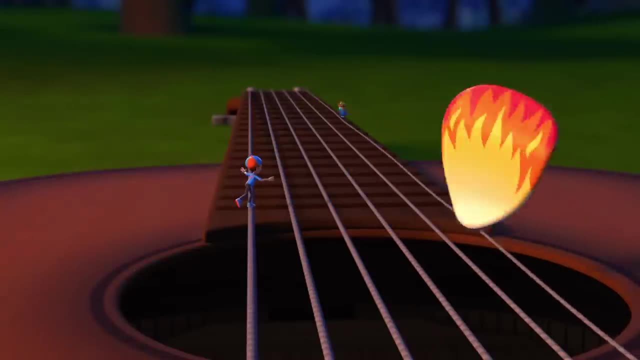 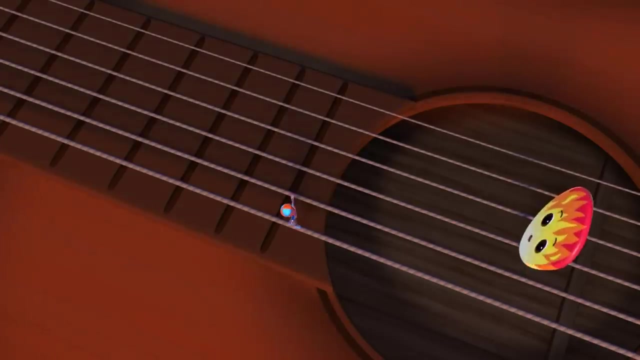 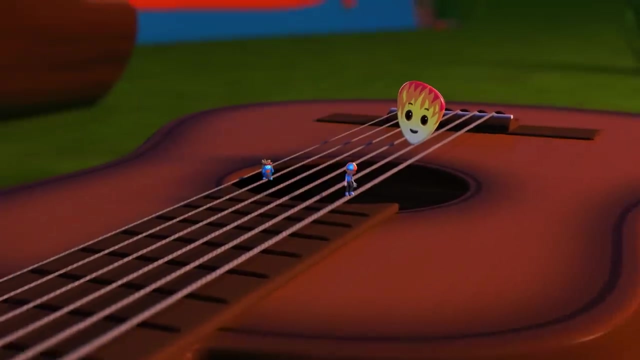 notes on a guitar. That's why I needed your help. Hey Deebo, could you move towards the far end of the neck mate Now back towards me, So low? Well, that explains how different notes are made. Why does the guitar have such a? 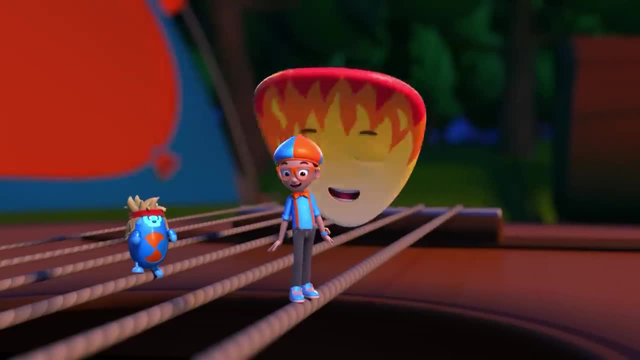 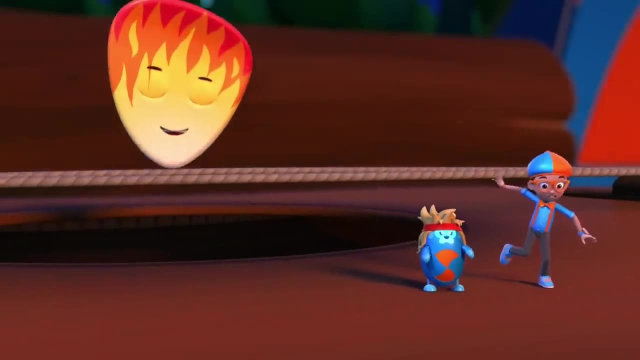 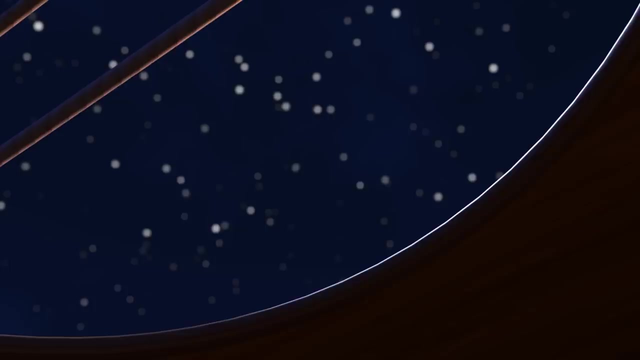 big body. That's the part that makes it low. Thank you, Hey. come stand over here on the soundboard. We're going up and down too. When I pluck the string, the whole guitar body vibrates and the 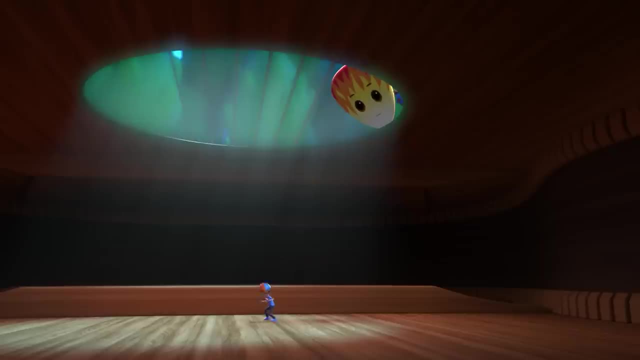 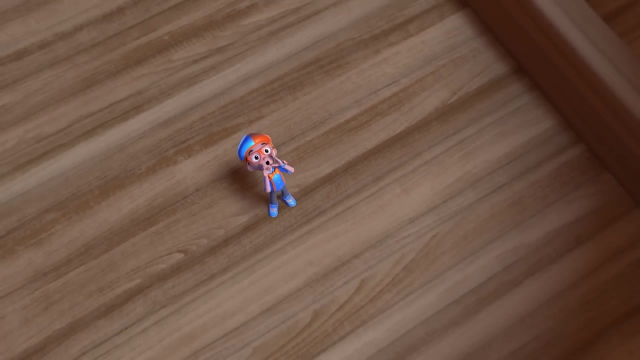 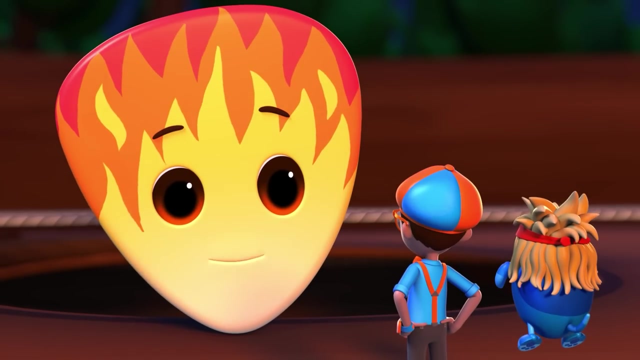 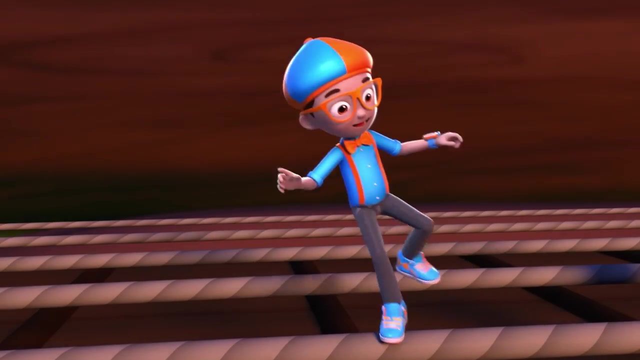 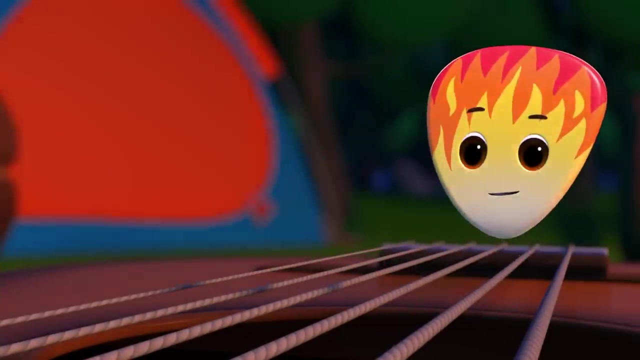 sound hole there makes it super loud, like shouting while cupping your hands over your mouth. Hello Whoa, That was loud, Right? Practice is over Time to jam. One, two, three, four, Thank you, And now I have the. 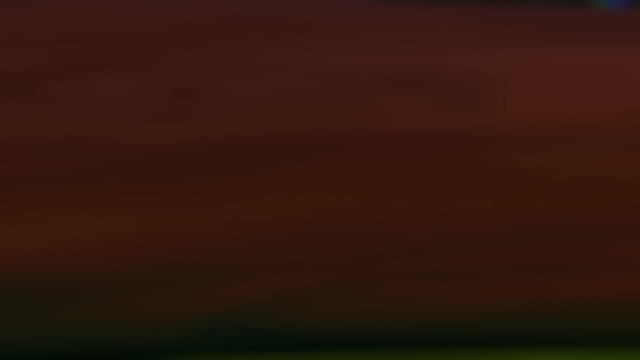 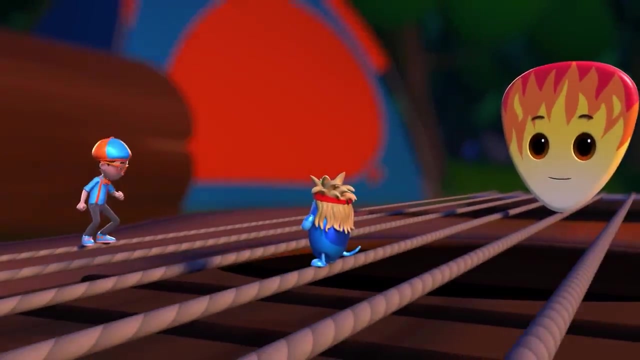 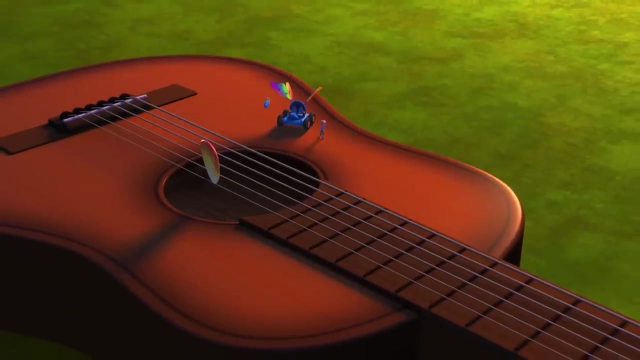 answer to my question: How does a guitar work? Guitars work because the strings vibrate and make sound, which is made louder by causing the whole hollow guitar body to vibrate. Upload answer: Deebo Buh-bye Picky. 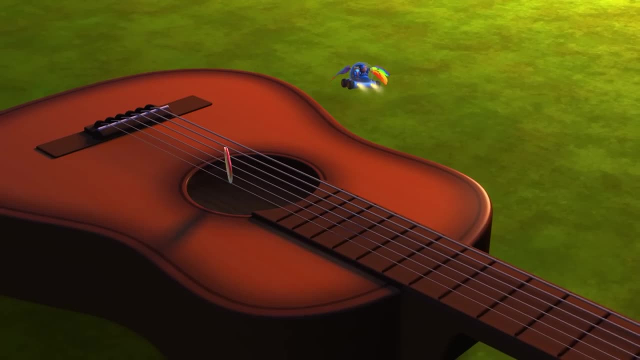 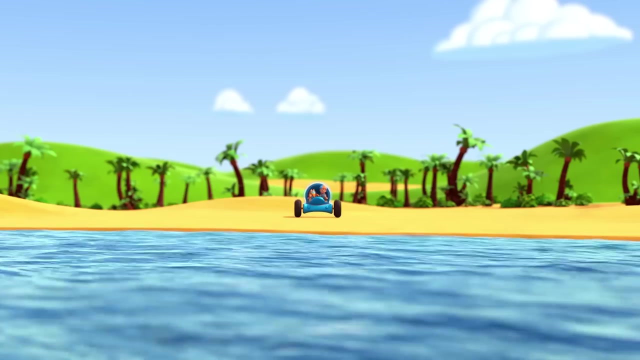 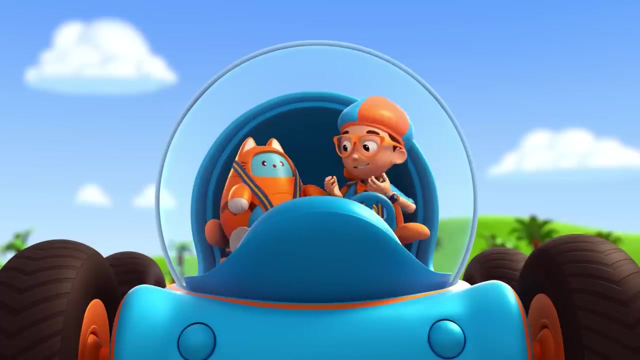 Bye Blippi, Bye Deebo. Remember to always keep rockin'. I love being at the beach. Whoa, A flying fish. Hmm, I wonder what's underneath the ocean. Good idea, Tabs: We can go into the ocean and find out. 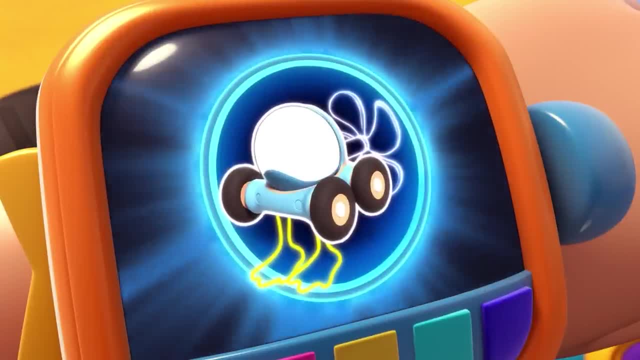 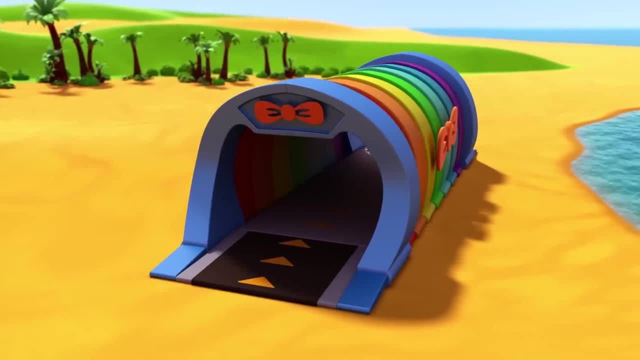 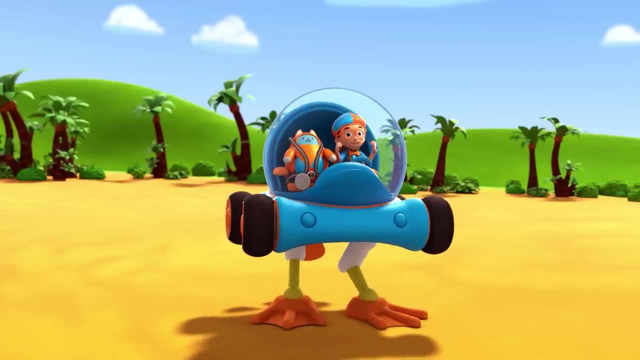 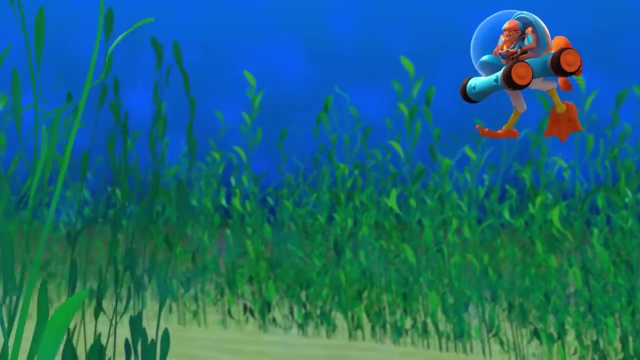 All need duck feet and a propeller. Duck feet, propeller confirmed, Activate Blippi Station. The Blippi-mobile is ready for adventure. Wow, It's a whole other world down here. Is this like some kind of underwater forest? Exactly. 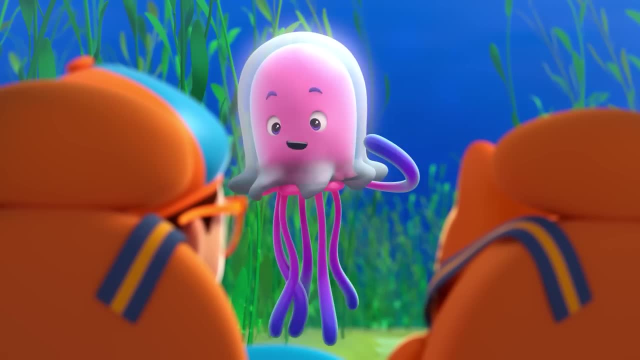 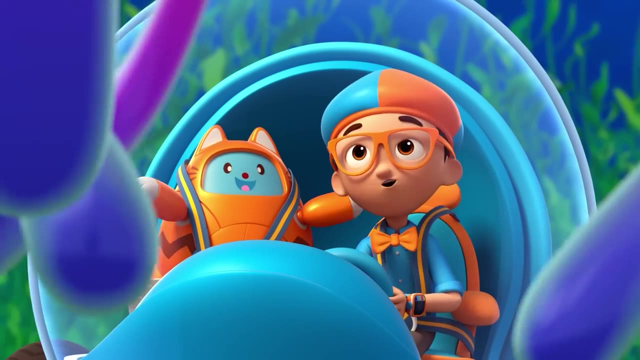 It is a forest. Welcome to my neighborhood. My name's Jerry, Jerry the Jellyfish. Hey, It's me Blippi, And this is Tabs. We're down here to see what's in the ocean. Oh yeah, there's a lot The ocean's. 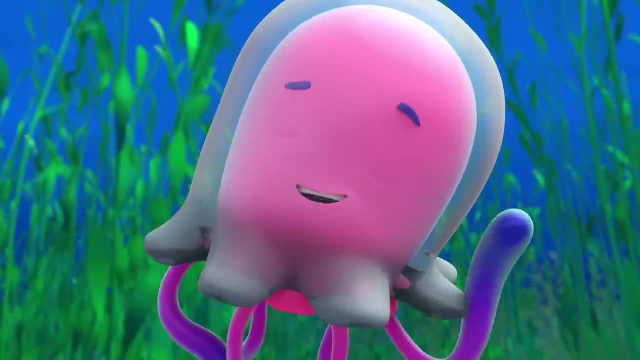 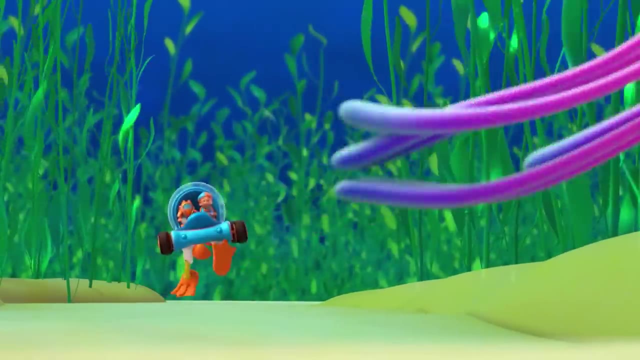 full of surprises. I'll show ya, I'm going to meet my friends and I'll give you a tour along the way. Alright, Thanks, Jerry. First, stop our kelp forest. This kelp can grow up to 150 feet, Wow. 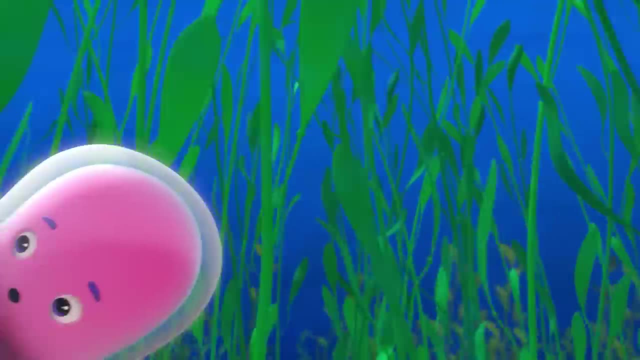 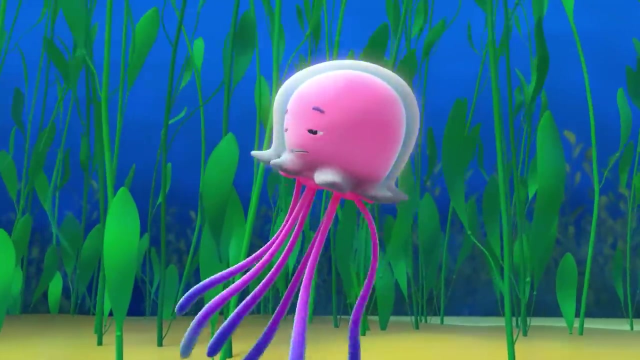 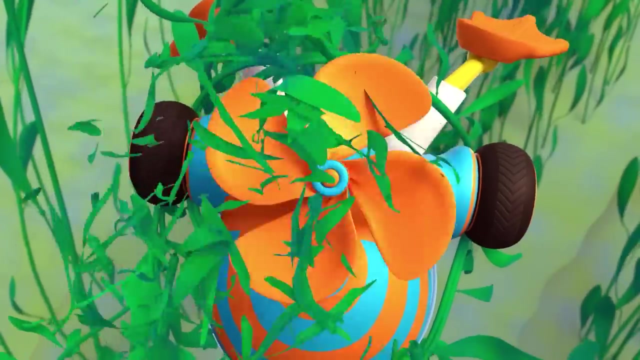 That's so tall, Oh yeah, but sometimes the water current around here blows the kelp around, Kelp, Kelp. Oh no, This never happens. Great idea: Tabs. Let's use the turbo boosters. Oh good, Glad you're okay, Let's move. 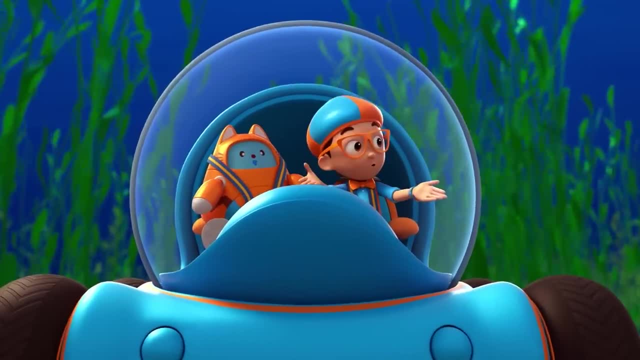 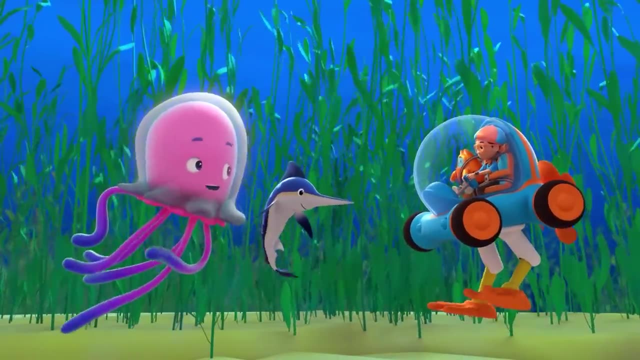 on Whoa. That fish is blue and has a long nose. She's a blue marlin. She used her nose to find and catch food. She's also really fast. Whoa, Whoa, whoa, whoa, Oh no. 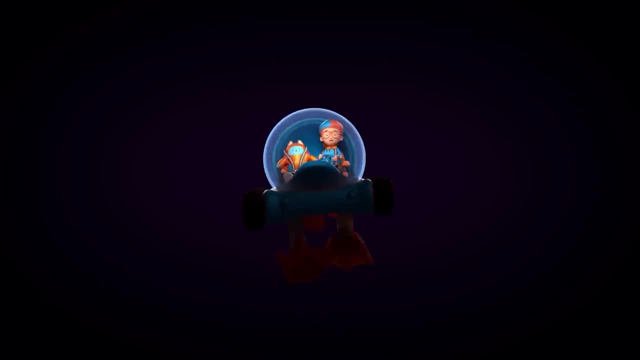 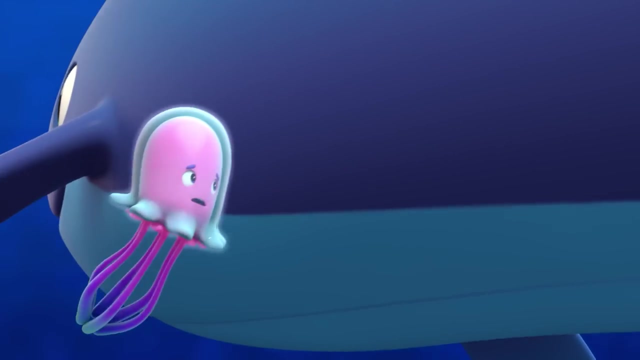 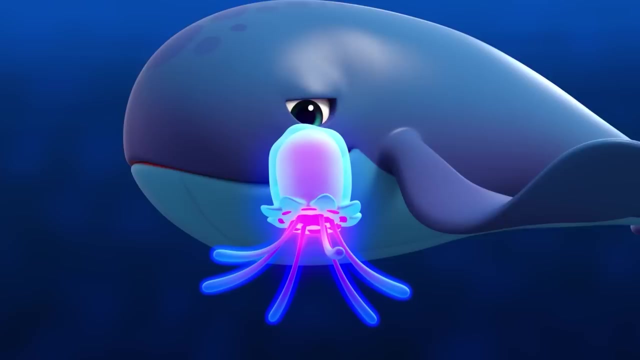 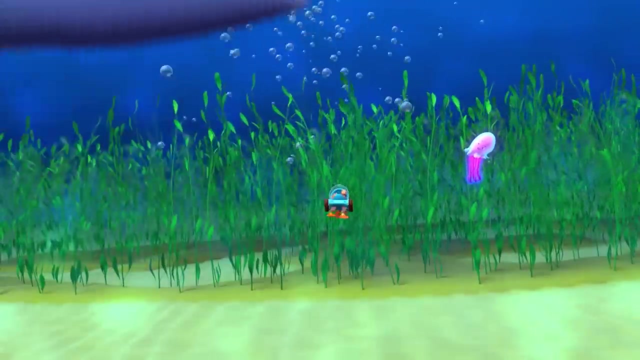 This never happens. Yeah, Tabs, It is dark in here Wherever we are. Jerry, Jerry Blippi, Is that you in there? Oh no, Hold on, Whoa, I scared a gray whale and she blew you. 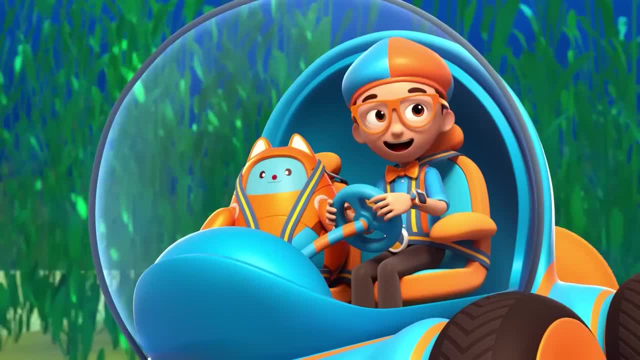 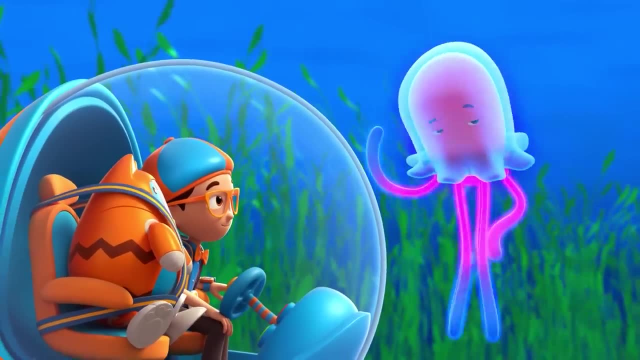 right out of her blowhole. That never happens. Thanks for getting us out of there, Jerry. Oh, you're all lit up. I told you the ocean was full of surprises, didn't I? Hey, look, It's your friends. 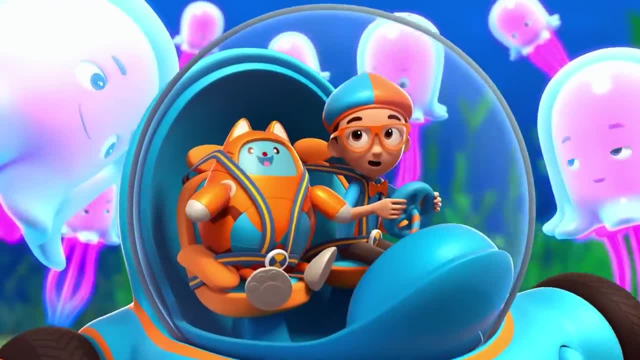 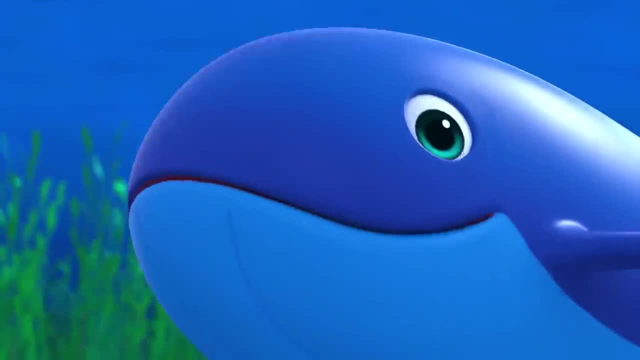 Hiya pals, You guys found me And I found the answer to my question. what's underneath the ocean? There's a kelp forest, blue marlins, huge whales and a jellyfish That lights up. Upload Answer Tabs. 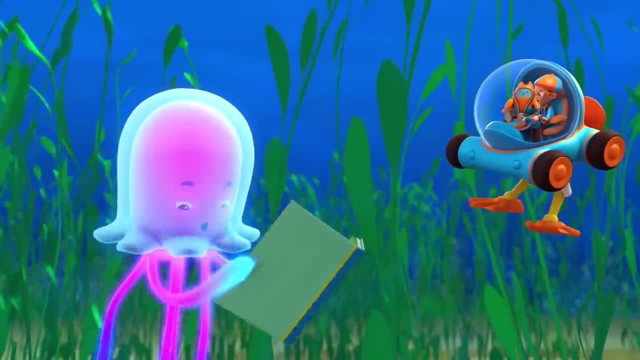 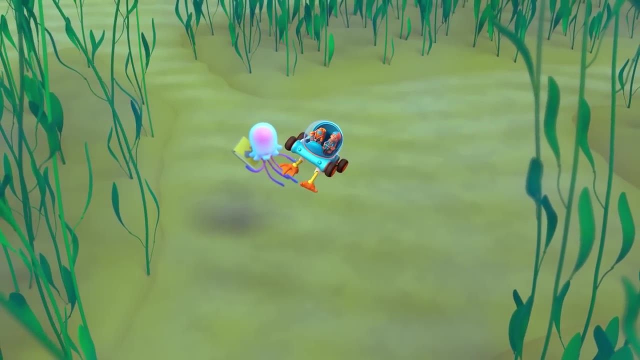 And we're only on chapter one. In chapter two there's an octopus and a shark and a sea turtle and a tuna- Bye, Jerry, Oh. and there's an otter and a seahorse and a. 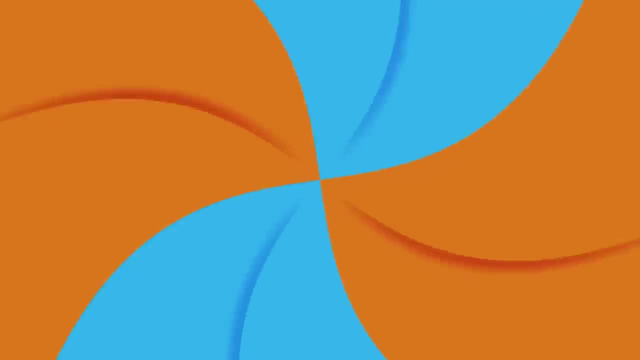 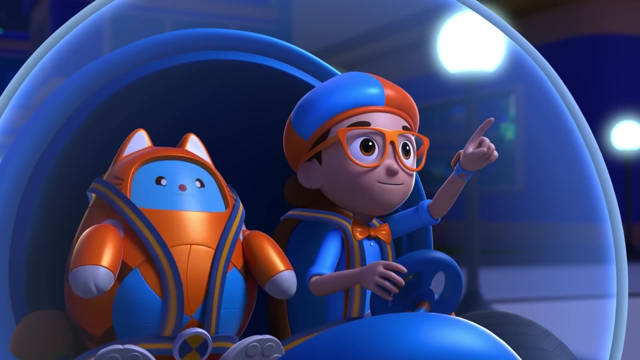 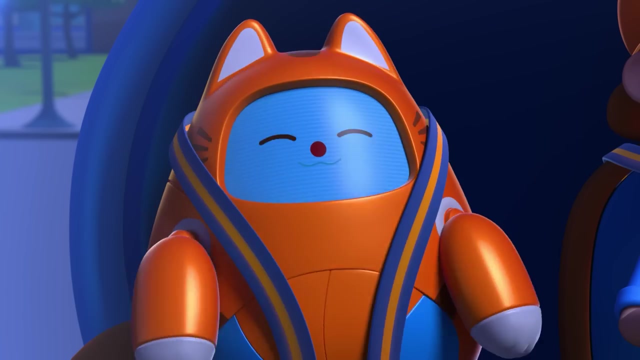 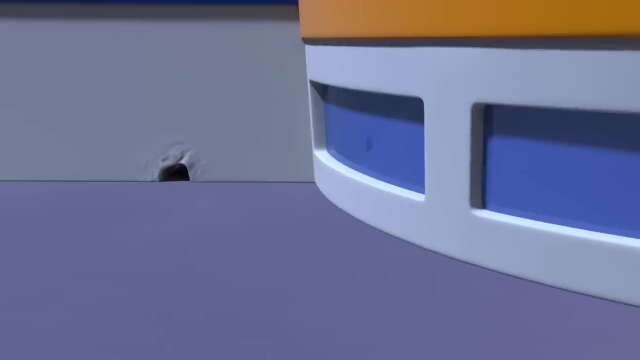 lobster and a stingray. Whoa, Look at that Tabs. It's an adorable kitty cat, Haha. And look at those super long whiskers. Hmm, I wonder, why do cats have whiskers? Great idea, Tabs, Let's follow that kitty. 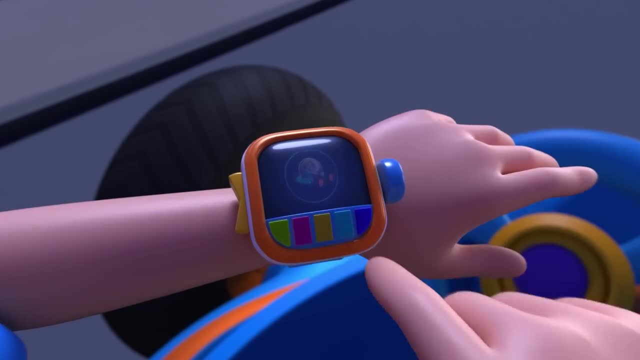 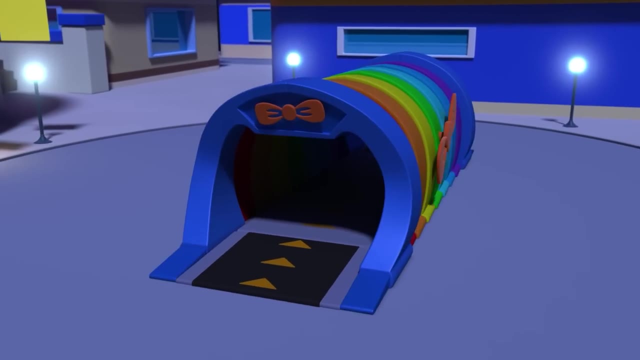 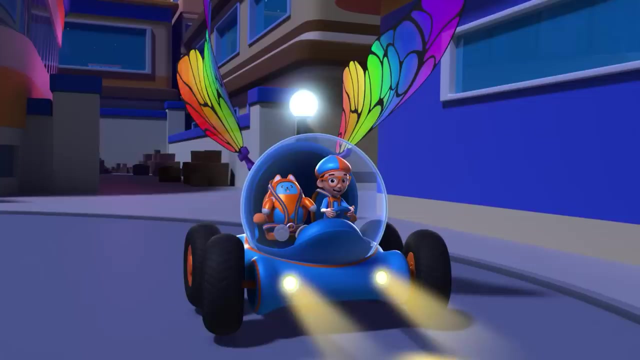 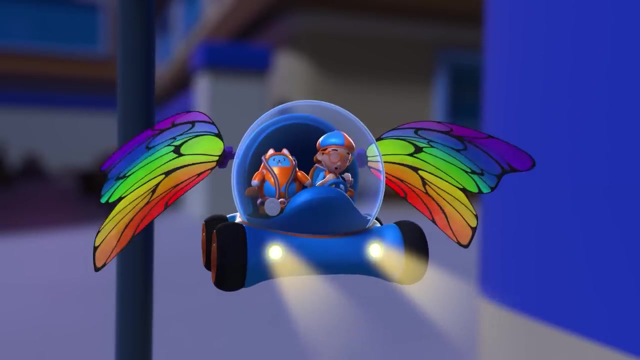 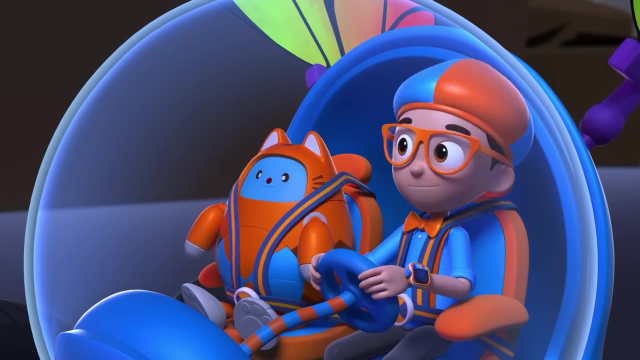 cat and find out. I'm gonna need wings, Wings, confirmed. Activate flippy stations Shrieking down. The flippy mobile is ready for adventure. Do you see any kitties yet? Tabs, Whoa, What was that? Hey, It's me Flippy. 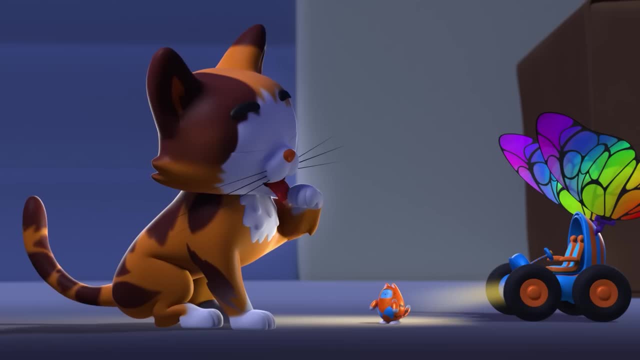 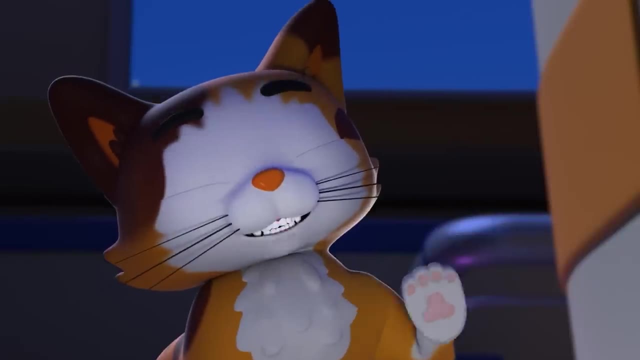 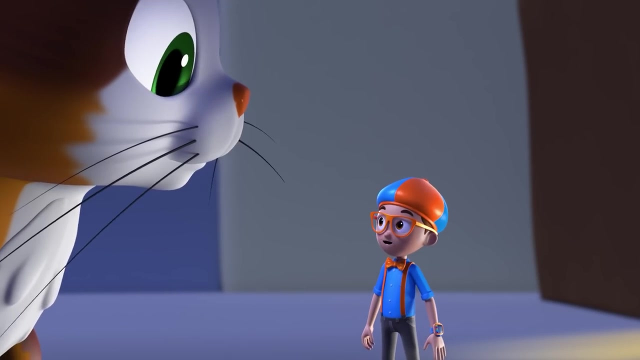 What's your name? Hippley's the name and treats are my game. Say you aren't holding out on me. are you Holding out on what Treats? I can smell them like hot cakes in the morning. They're close. 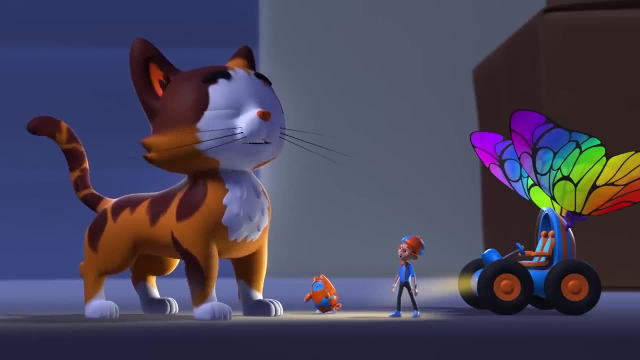 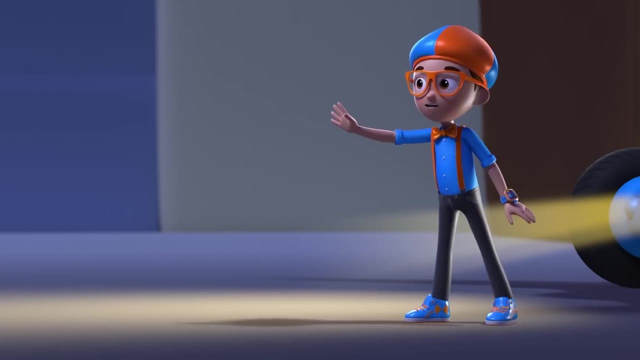 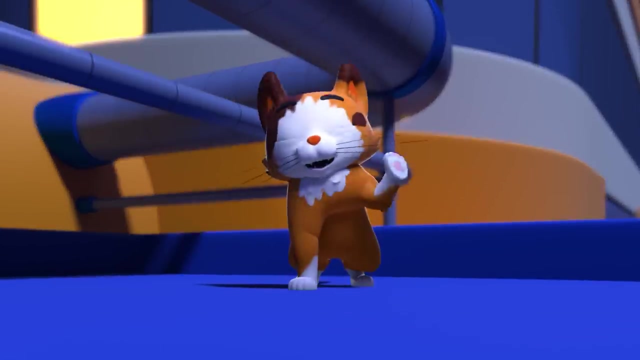 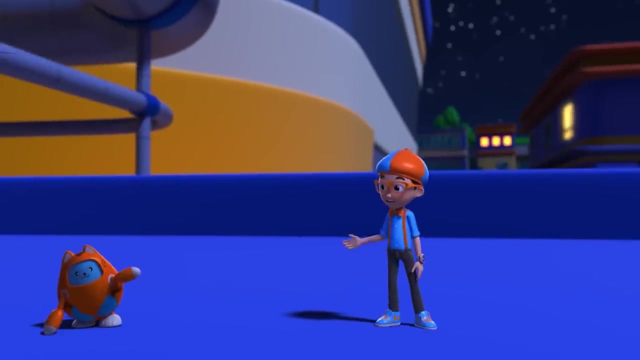 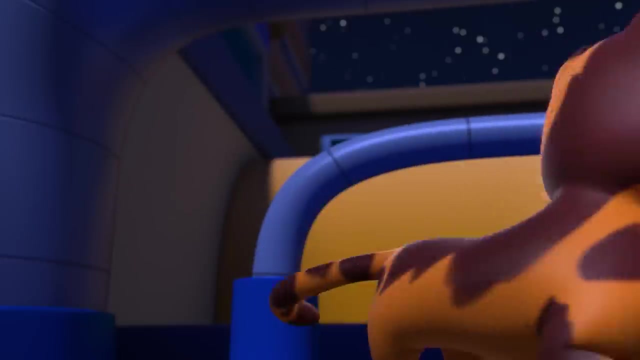 Hurry, Follow me, Oh, Oh, Follow me, Wait for me. Yee-haw, Woo, Flawless. How do you land so perfectly? My whiskers have special sensors that help keep me oriented, so I always land on my feet Like. 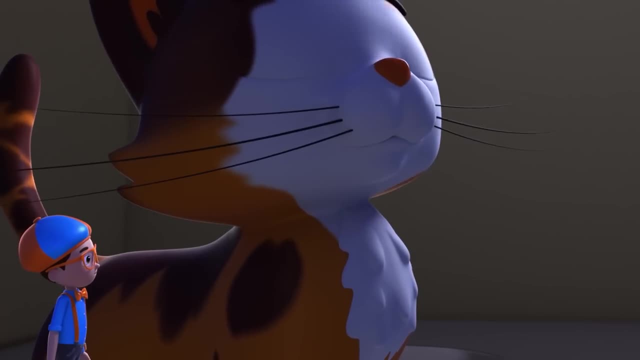 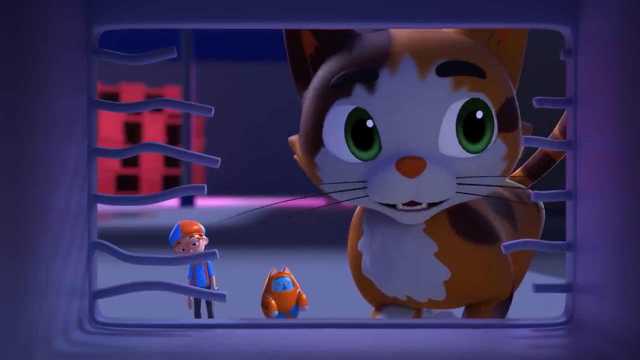 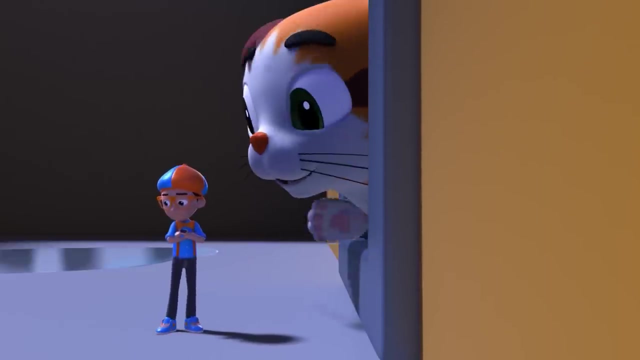 this. Haha. Do you think you can fit My whiskers? help me determine if I can fit through the passage without getting stuck. See, I told ya Come on Blippy. It's so dark, How can you see anything? 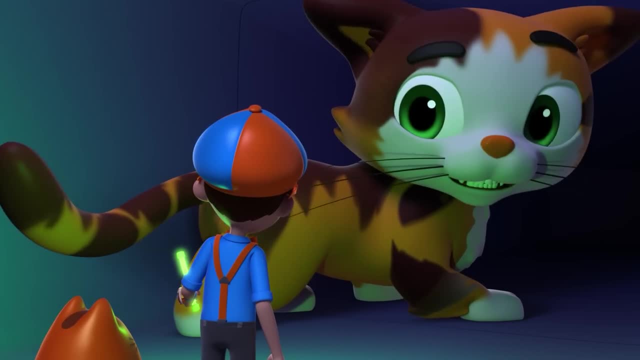 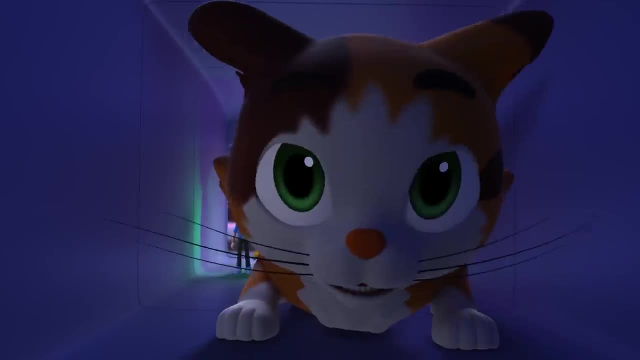 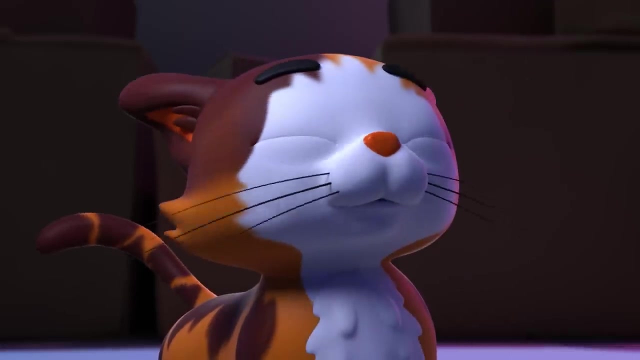 When I can't see what's around me, my whiskers tell me when something's there, Ah rats, No treats in here, But we must be close. Come on y'all. What else can your whiskers do? Even the slightest breeze? 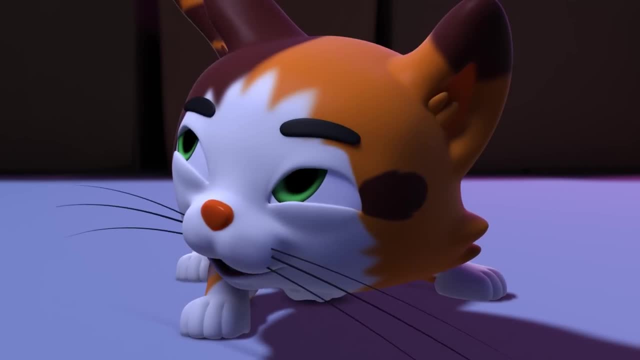 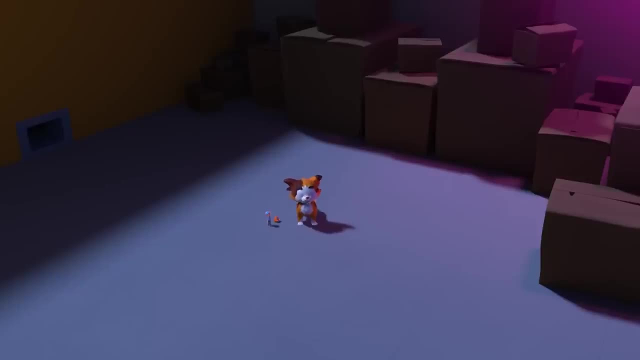 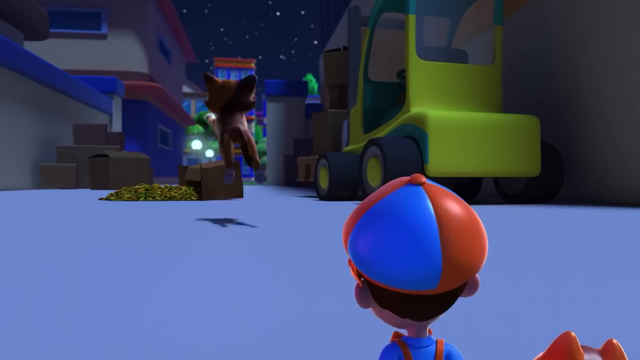 can tell me information about my environment and what direction a smell is coming from. My whiskers are telling me that the treats are Woo There, Woo Snack pod. Would you look at that? Woo-hoo-hoo, I'm happier than a pig. 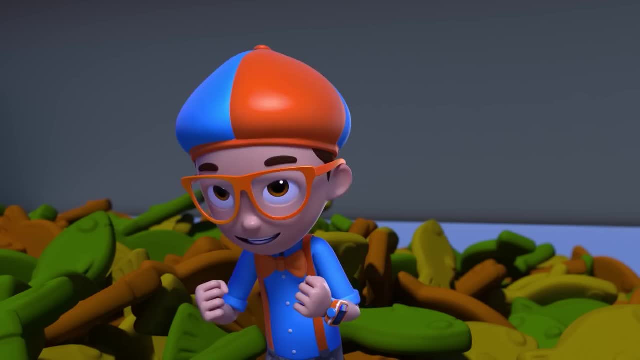 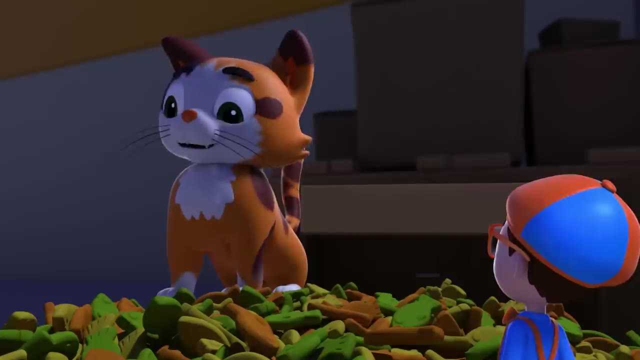 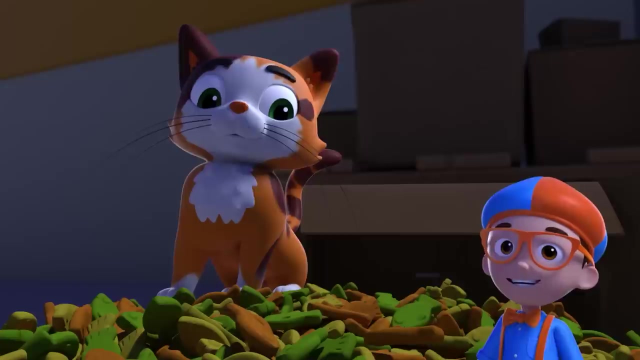 in mud. What a great adventure, Kipli: We found the treats And I got the answer to my question: Why do cats have whiskers? Cats' whiskers help them navigate their environment and help them keep oriented, so they always land on their feet. 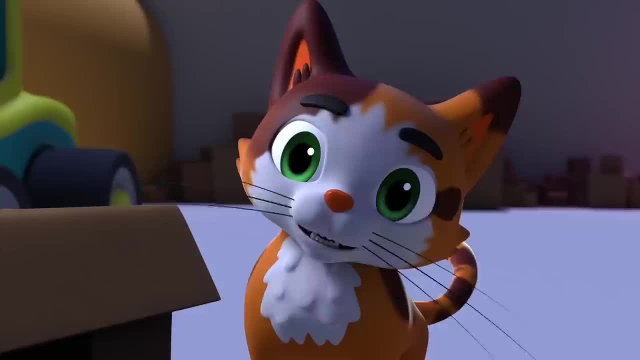 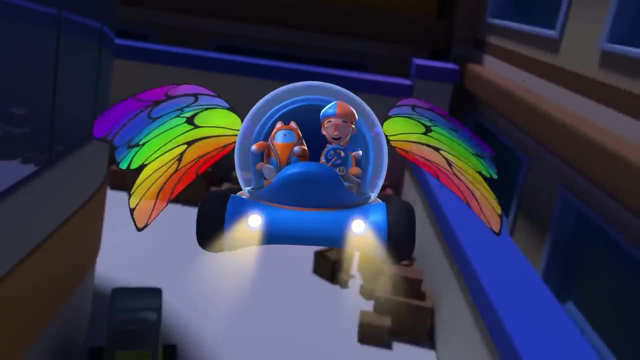 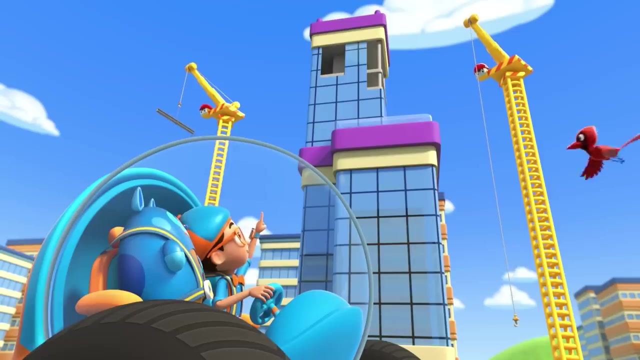 Upload answer tabs. Buh-bye Kipli. Thanks, Blippy. It was great to have you as a sidekick on this adventure. Bye y'all, Whoa. Look at that massive skyscraper with a crane next to it. 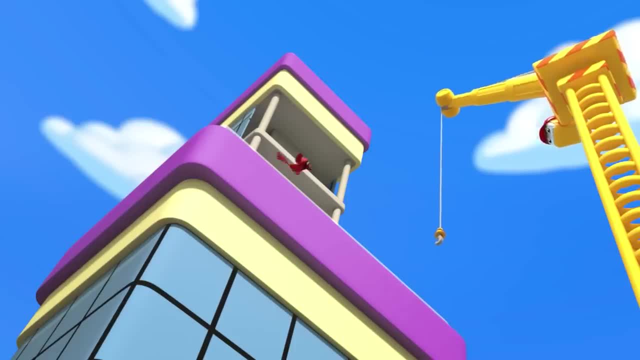 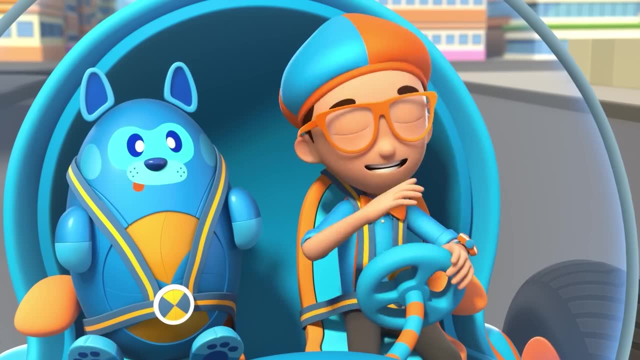 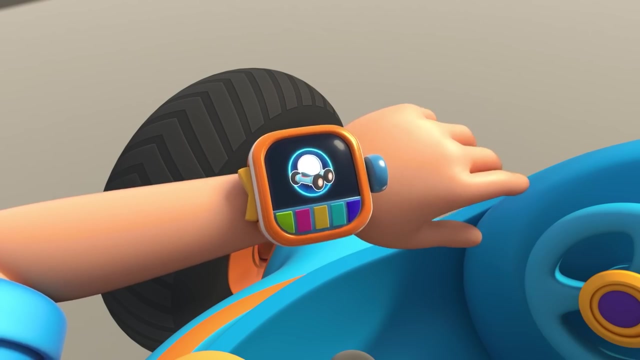 Right, Deebo, I think it is helping build the building. Hmm, I wonder: how does a crane help build a building? Great idea, We'll go talk to the crane. I'm gonna need a grabber arm and extendo legs. 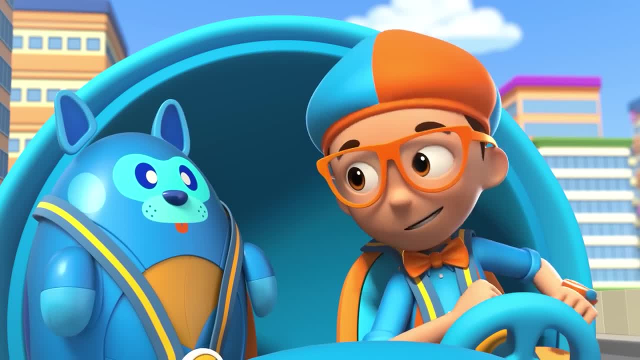 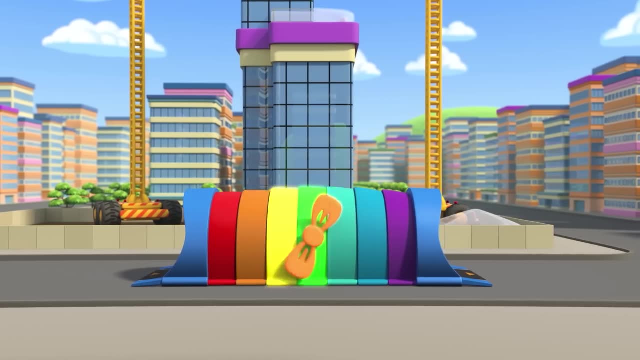 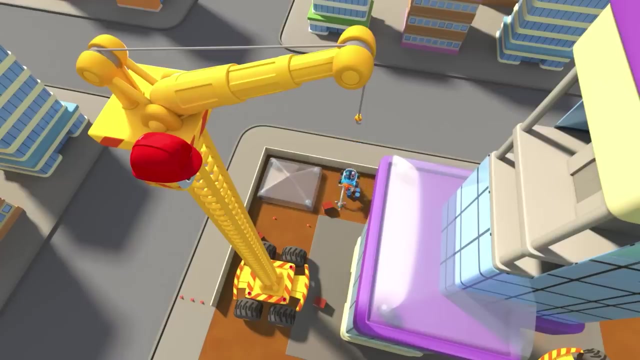 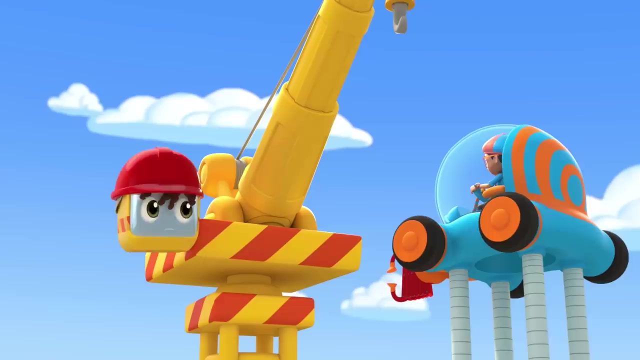 Grabber arm. Extendo legs- Confirmed. Activate Blippy Station. The Blippy Mobile is ready for adventure. Extendo legs up. Whoa Hi, Um, are you here to help me? Hey, It's me Blippy, And this is my. 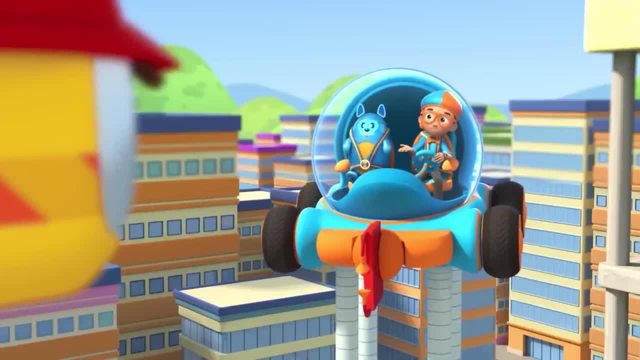 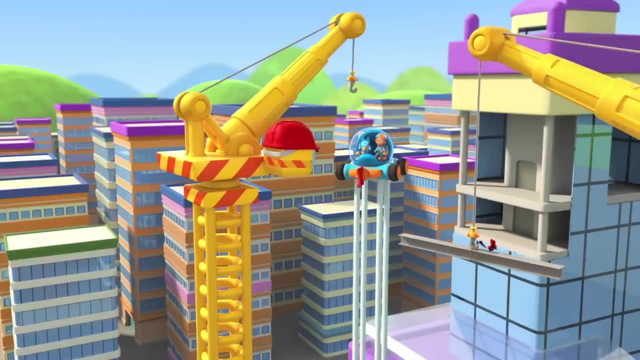 name. This is Deebo. Sure, I'll help. What's your name? It's Kareem. Kareem the crane. It's my first big job today. I'm kinda nervous. I get it. Trying new things makes me nervous sometimes too. 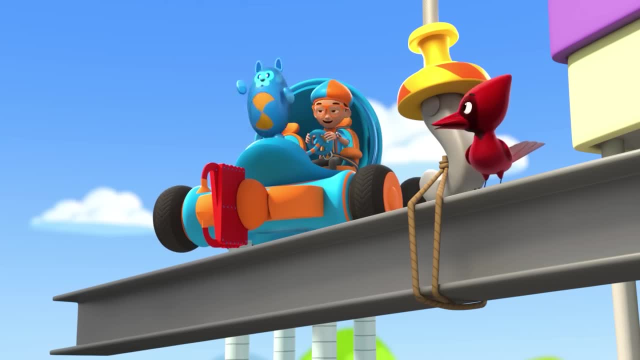 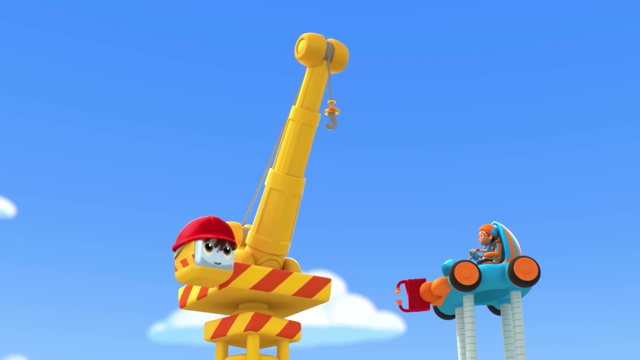 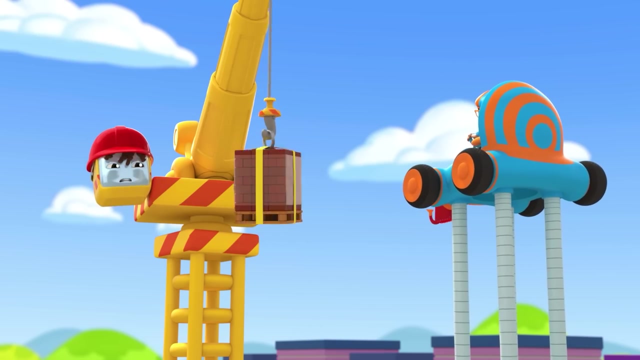 We'll help you any way we can. I spin my mast, my tall body around and then I extend my jib down. The jib is my long arm. Now I can use my hook to pick up these really heavy bricks. Whoa, I can't stop it. 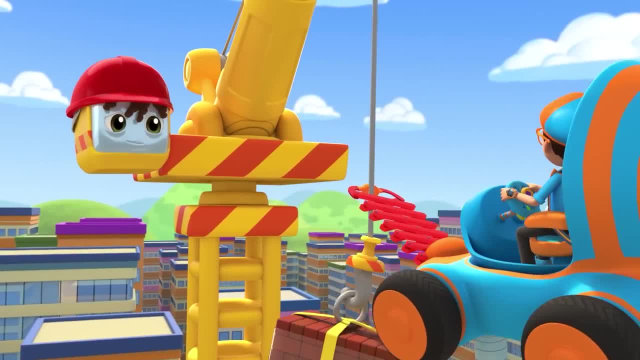 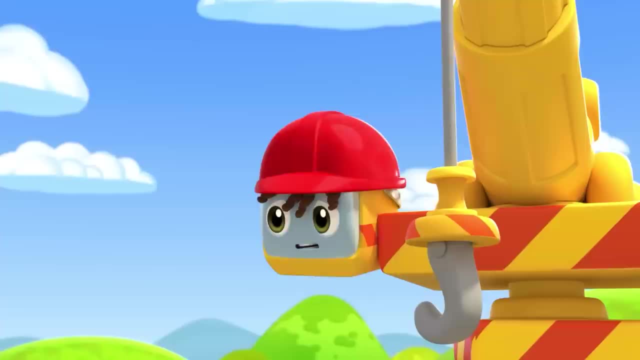 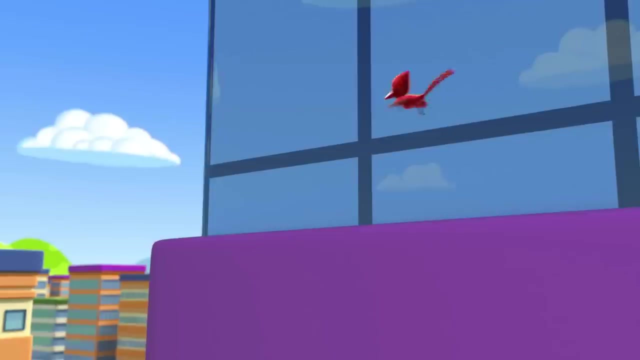 swinging Gotcha. Thanks, Blippy. I'm still learning, but I'll figure this out. Now you can help me with the roof. It's that big glass square down there. Glass is very fragile. You got this, I'm doing it. I'm. 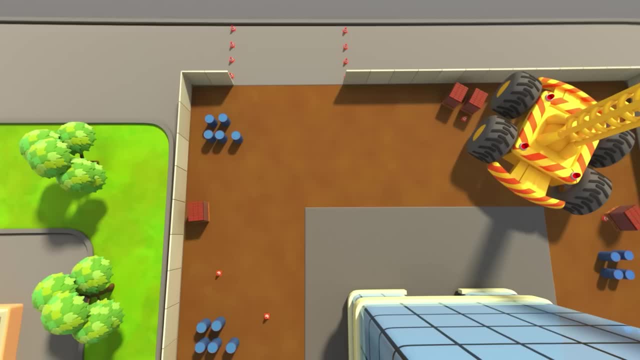 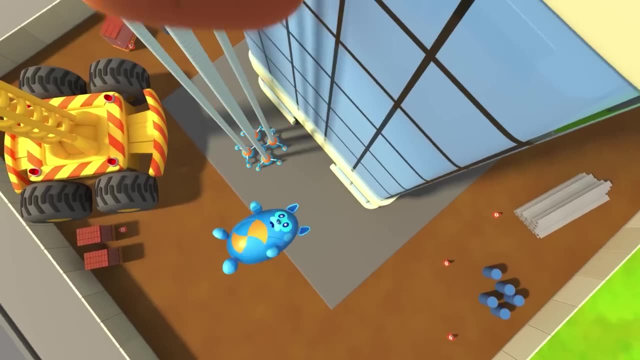 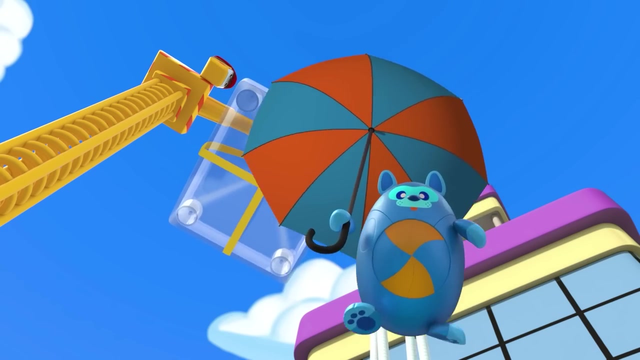 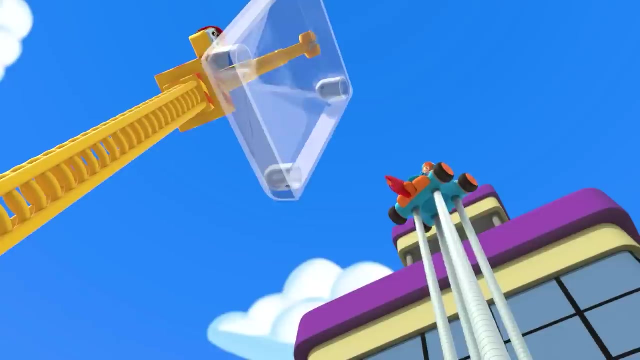 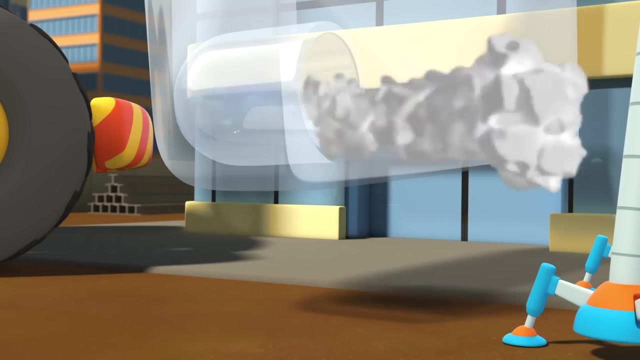 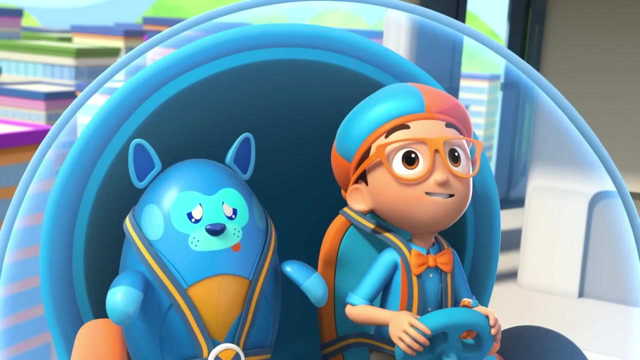 really doing it Now. take it up, Kareem. Oh Goodness, Look out below. Got it Now. let's finish the job. Ha ha ha. Yeah, Isn't helping Kareem so fun. Ha ha ha. Hey, We did it. 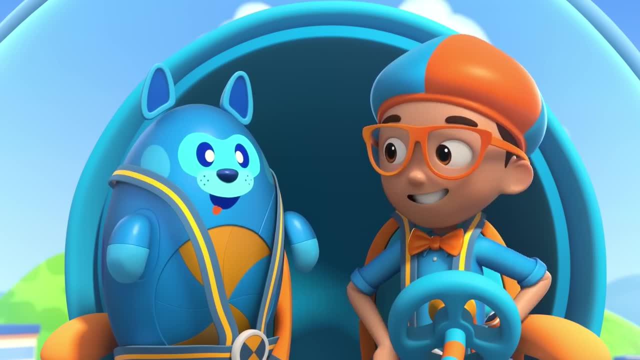 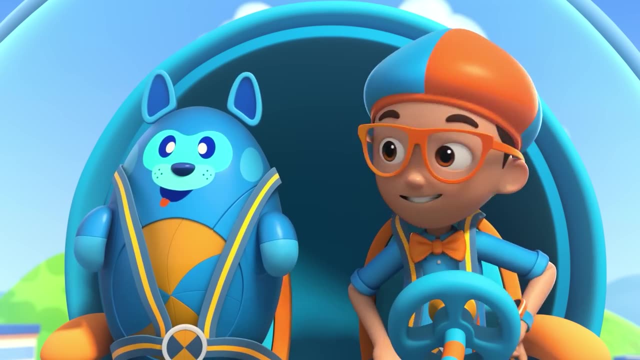 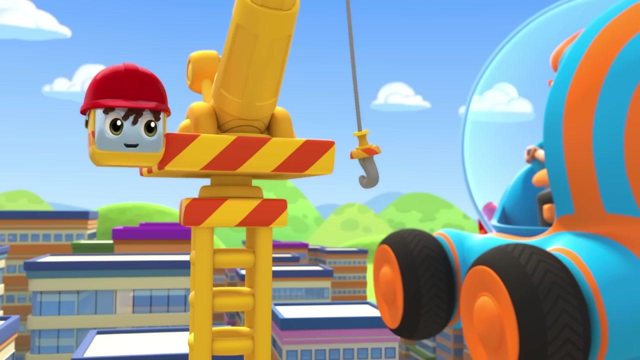 And now I know the answer to my question: How does a crane help build a building? Cranes lift heavy materials so they can be used to construct super tall buildings. Upload answer: Debo: Yes, Thanks for everything. Bye, Bye, Kareem. 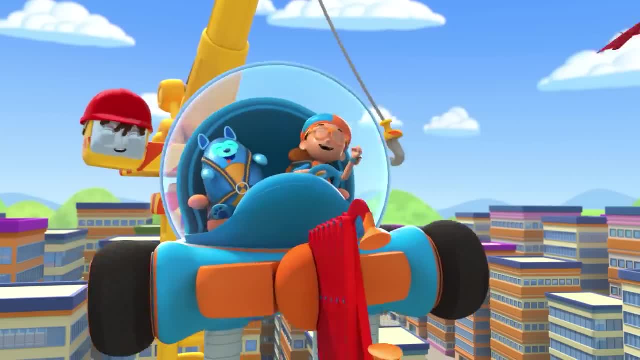 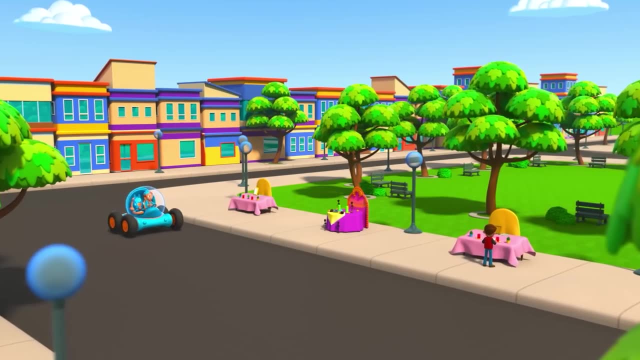 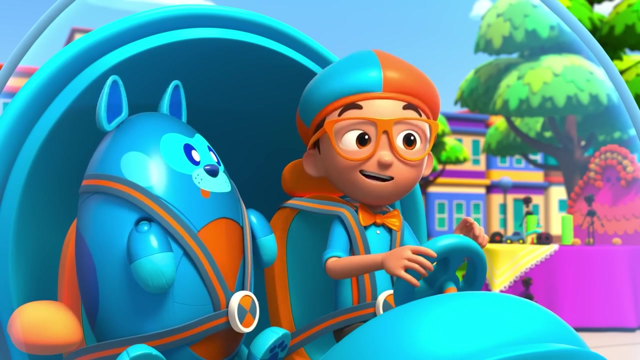 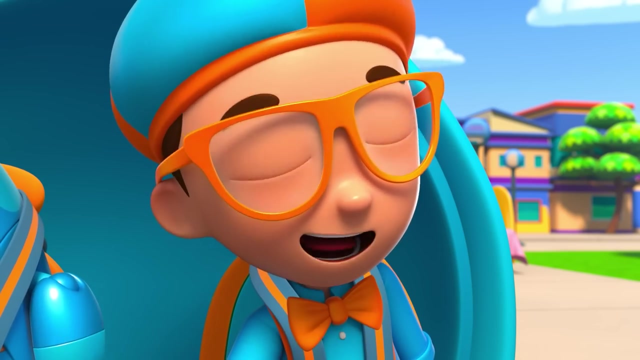 I knew you'd be an amazing crane. Whoa, What is that? You're right, Debo. I think he's setting up for Dia de los Muertos, the Day of the Dead. Hmm, I wonder, why don't you celebrate? 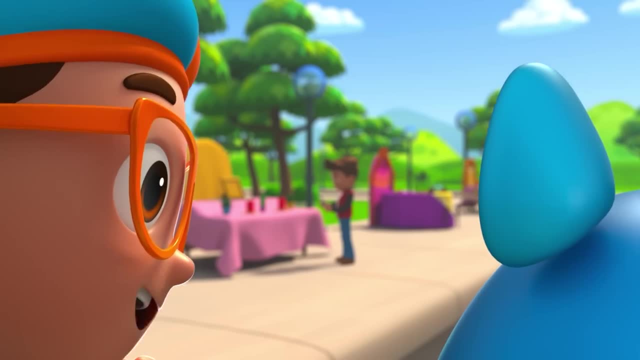 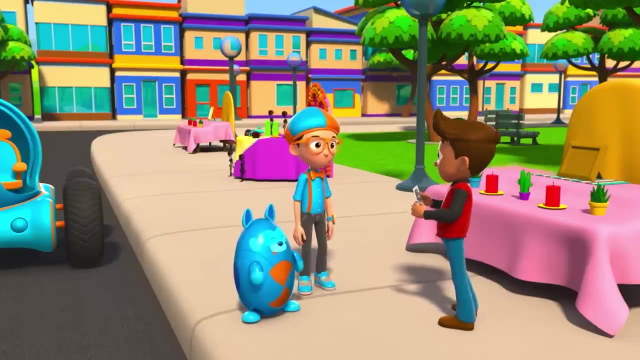 Dia de los Muertos. Great idea, We'll go ask him and find out. Hey, It's me Blippi And this is Debo. Oh hi, I'm Paco. Paco. What are you making here? 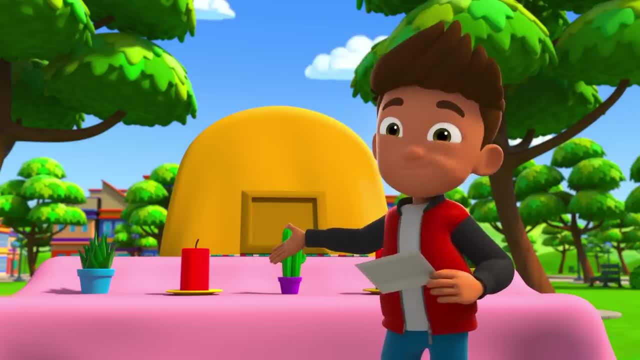 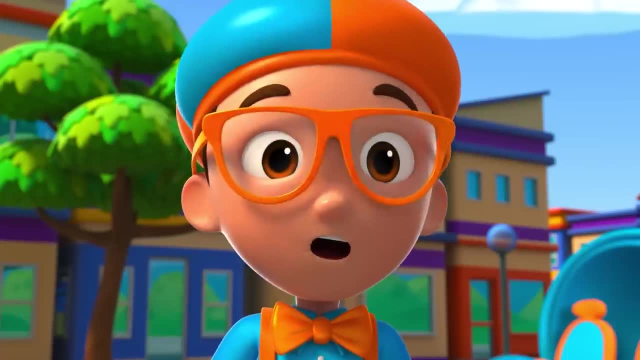 I'm making an ofrenda. It's part of a Mexican celebration where we remember the family members who are no longer with us, But I have a problem. What's wrong? I'm thinking about my great-abuela Rosa. I need to know what things she liked. 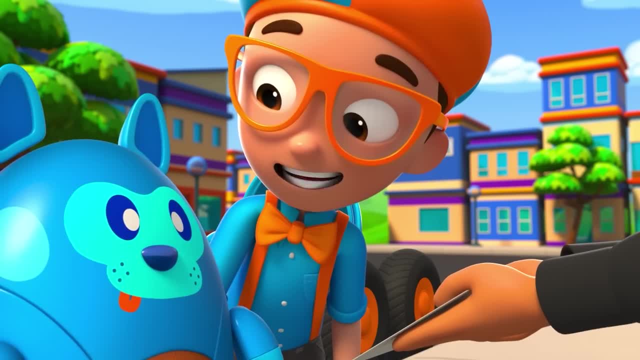 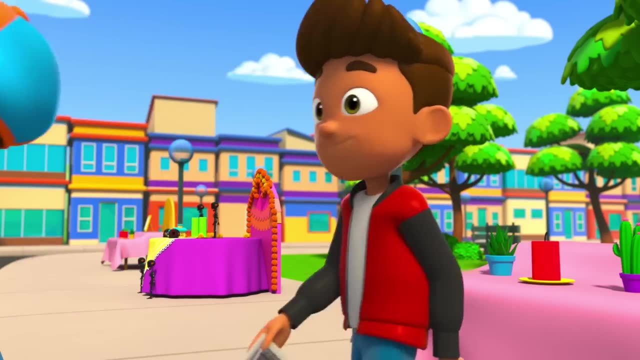 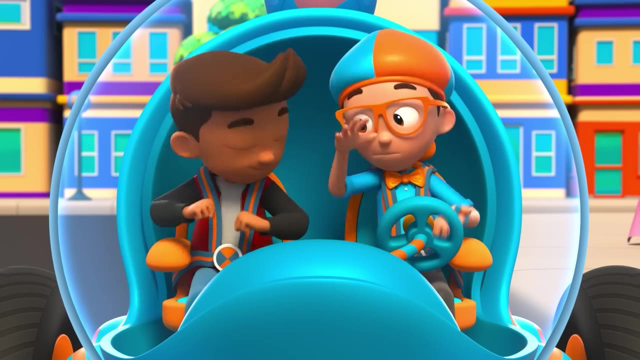 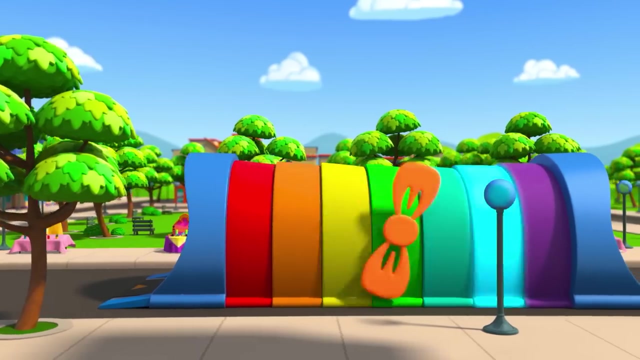 so I can make a proper ofrenda for her Great idea. Debo, We can go back in time and meet your great-abuela Rosa. Just follow us. I'm gonna need wings. Wings confirmed, Activate Blippi Station Going back in time. 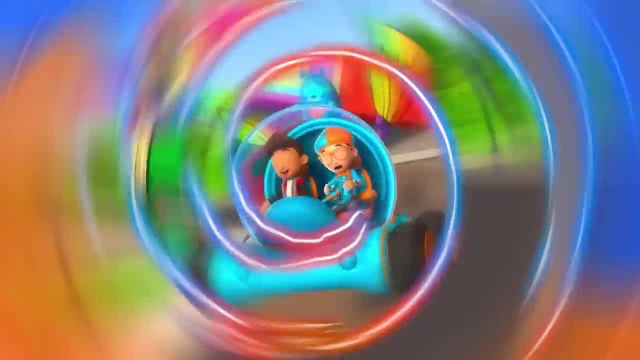 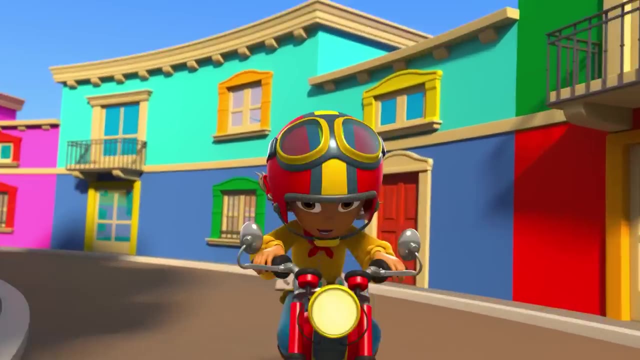 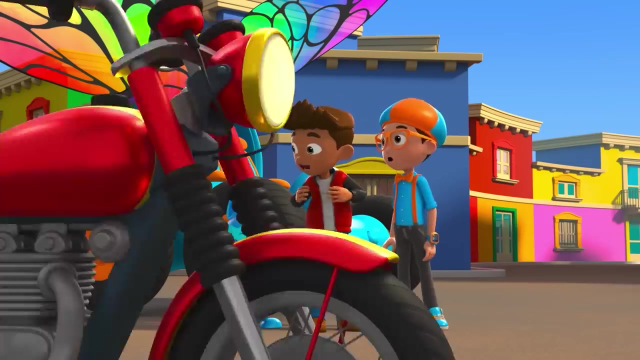 Going back in time. Going back in time. Whoa, where are we? Whoa, where are we? Welcome to Mexico. Whoa Great-abuela Rosa. Yes, Hi, It's me Paco, your great-grandson from the future. 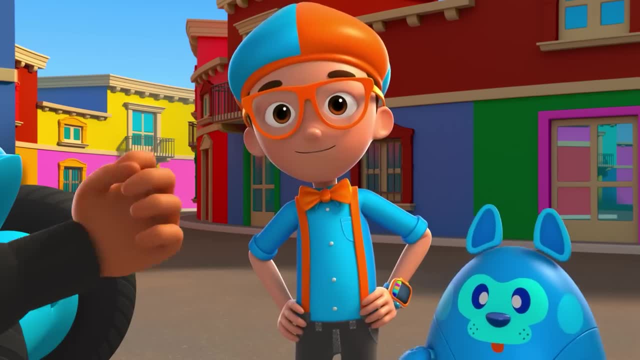 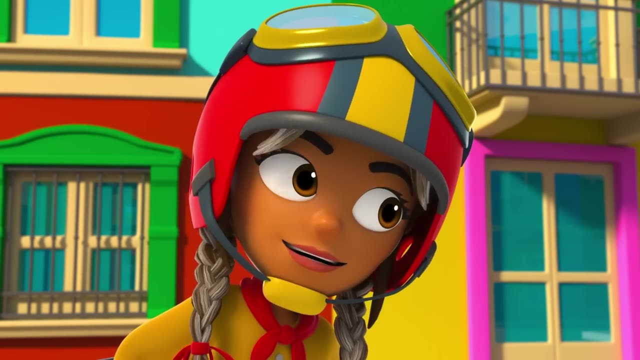 Hola, mijo, And who are your friends? This is Blippi and Debo. Hola, Hola. What are you doing here? Don't tell me you don't know how to make a proper ofrenda for me. 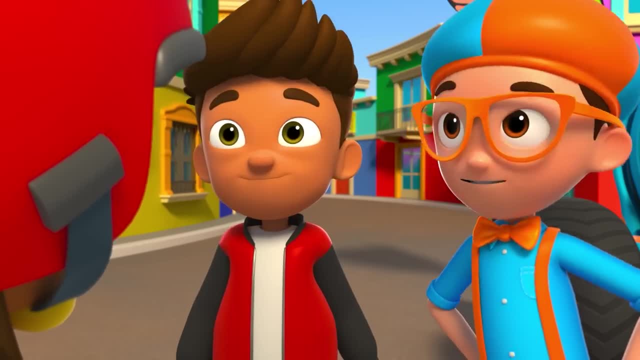 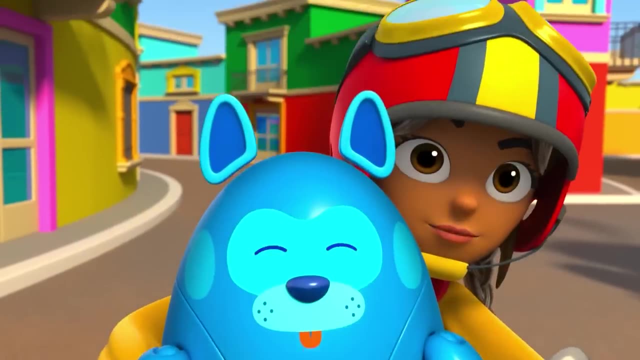 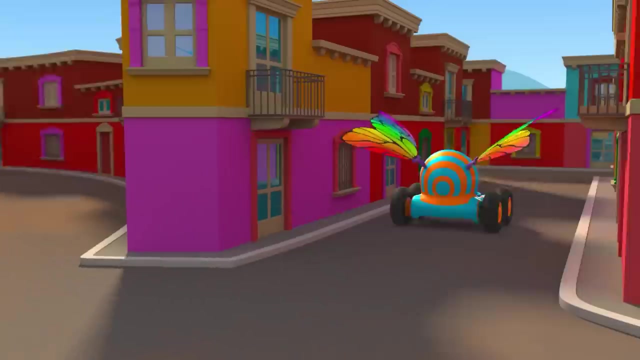 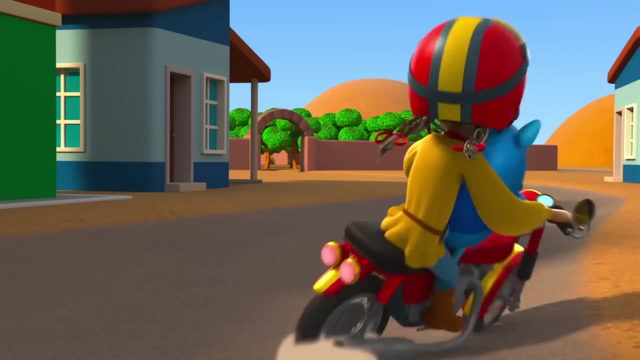 Well, Nope, he doesn't. Bueno, I will show you all my favorite things. Come on. The first thing I love is riding Fast. Whoa, You're really fast. Whoa, You're really fast. My second favorite thing: 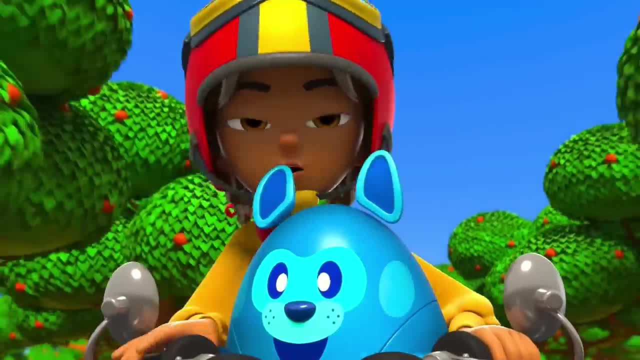 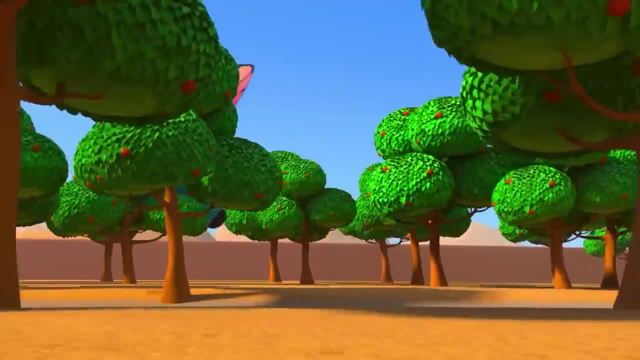 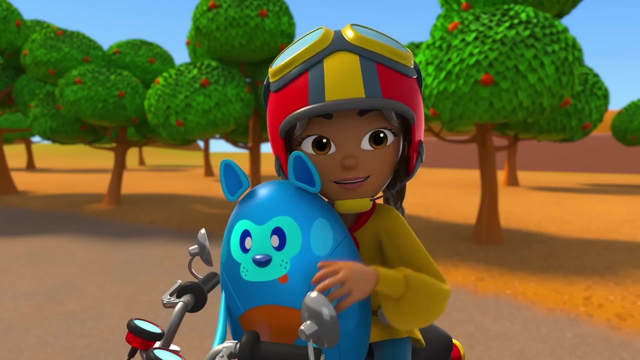 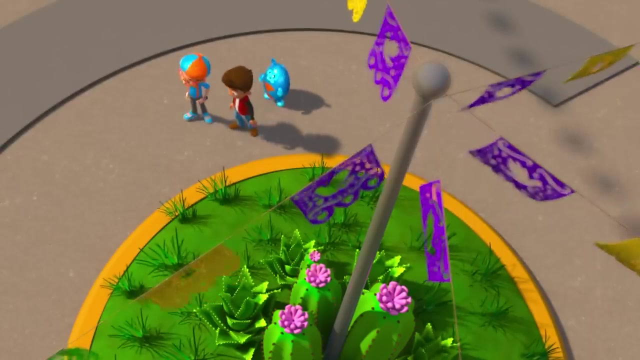 is oranges. They are so juicy and sweet. Mmm Yeah, Oh no, We can make orange juice. Follow me, Follow me, Follow me. Okay, my third favorite thing is musica. I love music. Well then, you must dance. 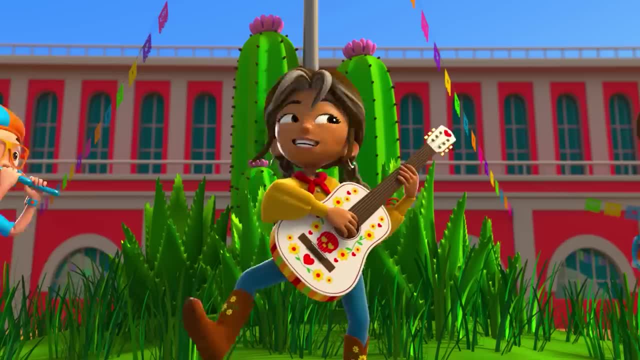 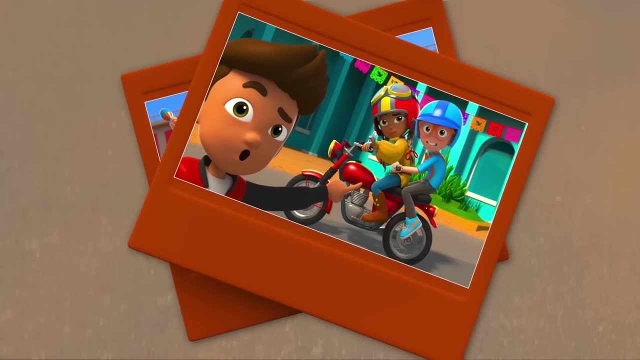 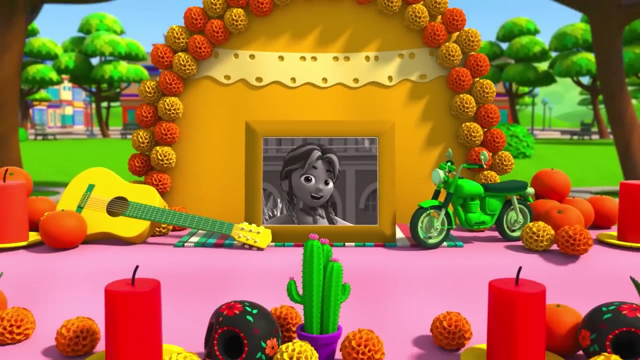 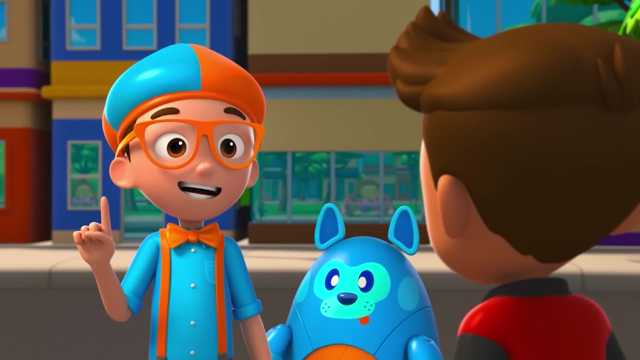 Well then, you must dance: Woo, Yeah, Aha, Woo. Thank you, Blippi, for helping me learn about my great Abuela Rosa. You're welcome, Paco, And I got the answer to my question. To celebrate Dia de los Muertos. 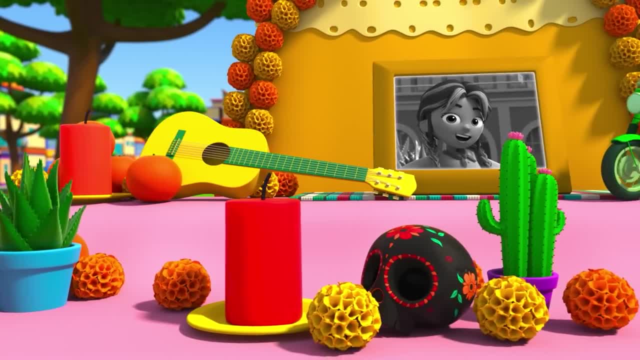 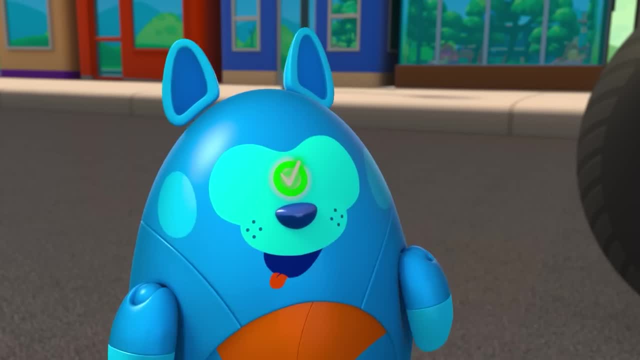 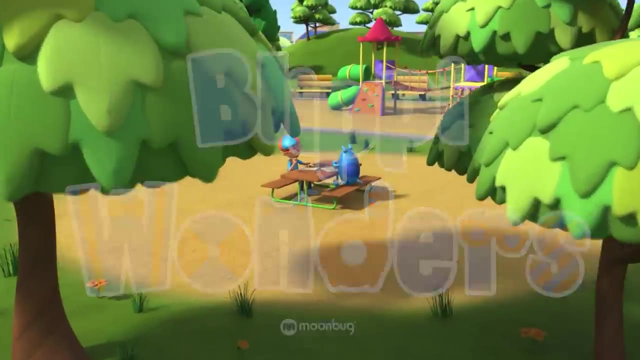 To celebrate Dia de los Muertos, you can make an ofrenda with the things that truly represent the spirit of our loved ones. Upload answer. Deebo Bye, Paco, Bye Blippi, Ready. Deebo Three, two, one. 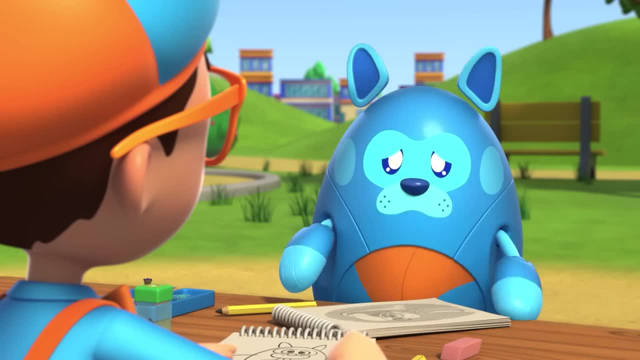 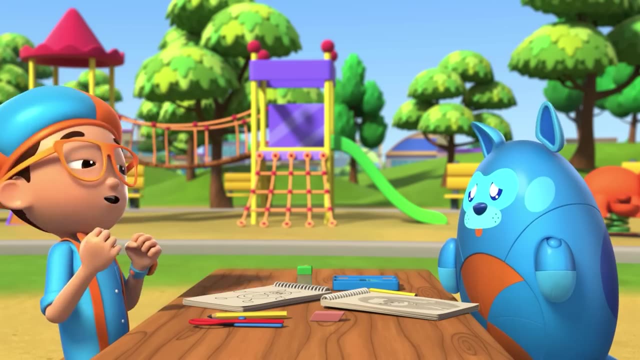 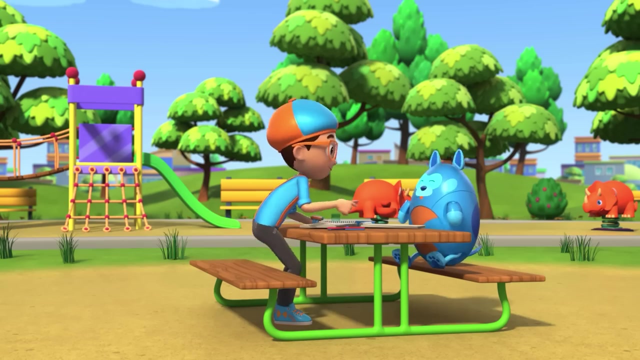 Three, two one, Three, two, one. Yeah, it's not quite what I envisioned. I wish I could make a few changes. Oh yeah, I can use an eraser. Hmm, I wonder how does an eraser work? 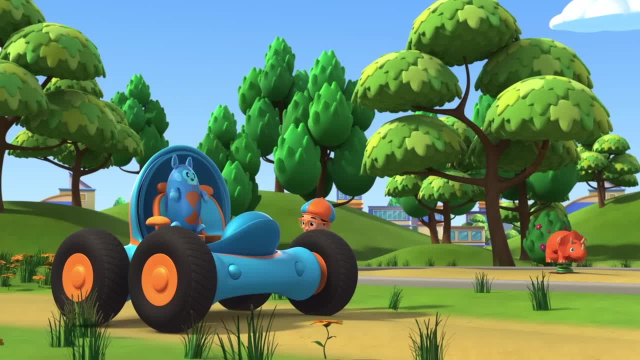 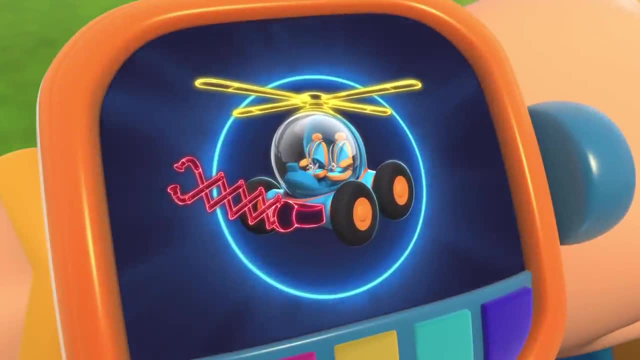 Great idea, Deebo. We'll shrink down and get a closer look. We'll shrink down and get a closer look. I'm gonna need a grabber arm and helicopter blades. Grabber arm- helicopter blades- confirmed Activate Blippi Station. 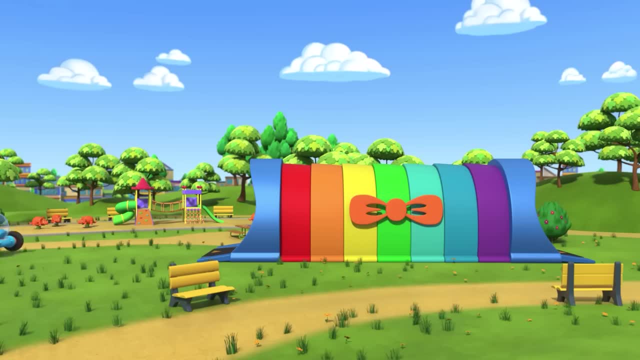 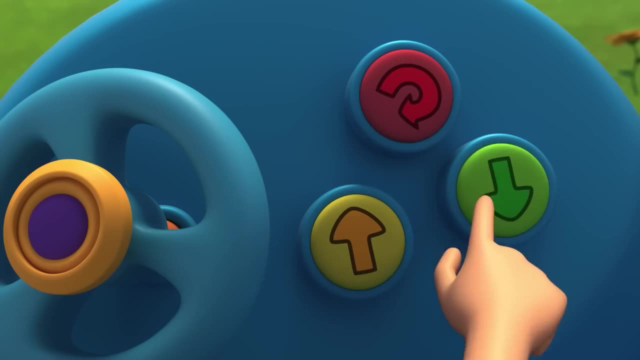 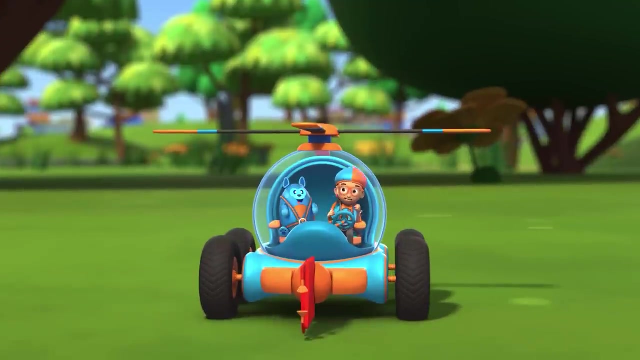 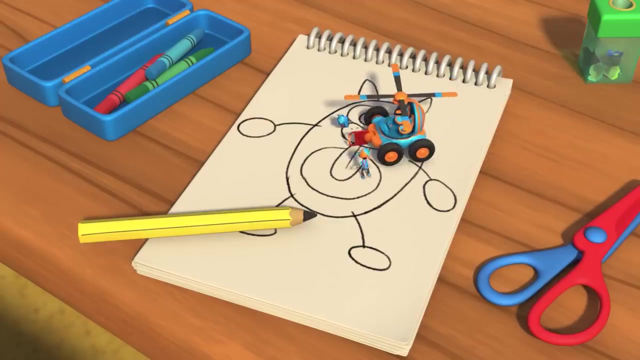 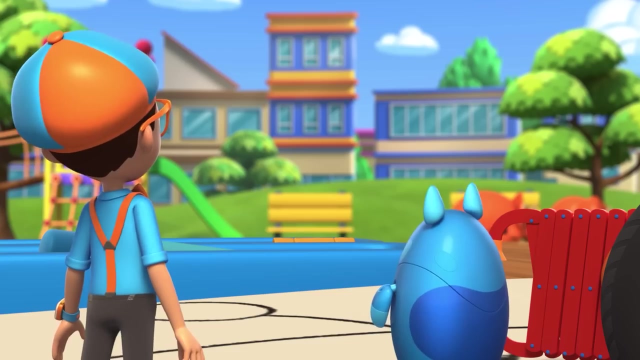 Activate Blippi Station. Shrinking down, Shrinking down. The Blippi-mobile is ready for adventure. Hmm, even up close, It sure does need some changes. Maybe I can help. I am the amazing Ernie. Hey, it's me Blippi. 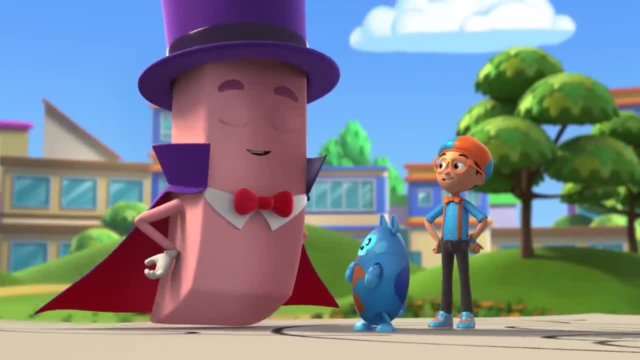 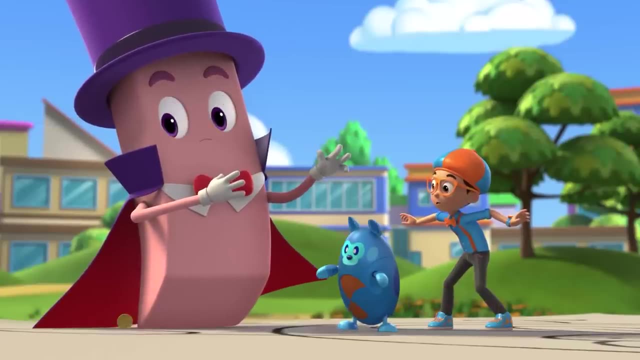 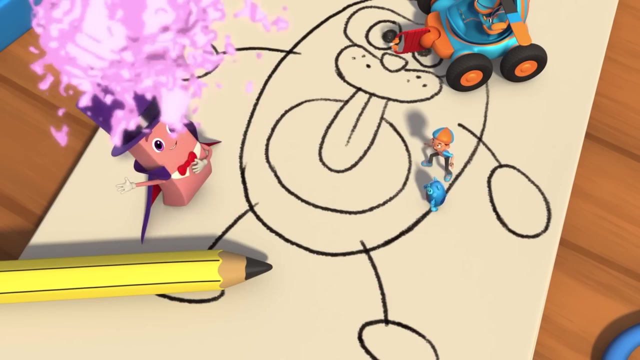 And this is Deebo. We're here to learn how an eraser works. Well, you came to the right eraser, because I can make anything disappear, Even pencil markings. That's amazing. Come see, it's the best show in town. 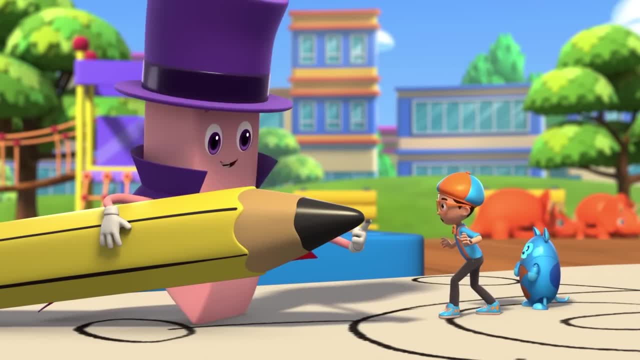 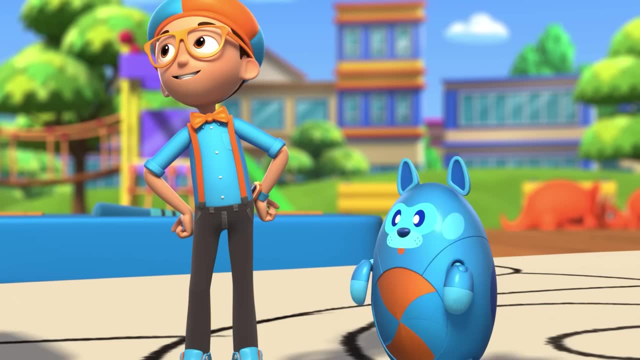 The tip of the pencil is made of graphite And when you rub it on paper it leaves a mark. Cool, Let's take a closer look through a magnifying glass. Graphite gets left behind on the paper because it actually sticks to the paper. 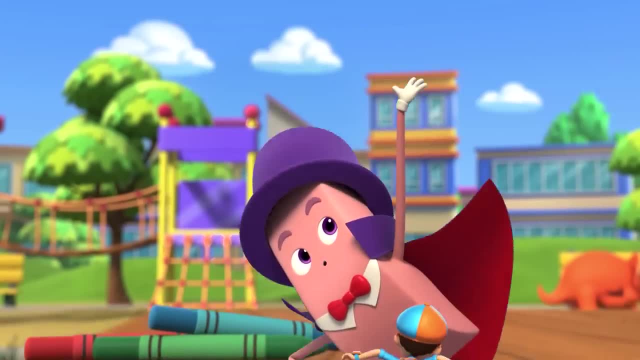 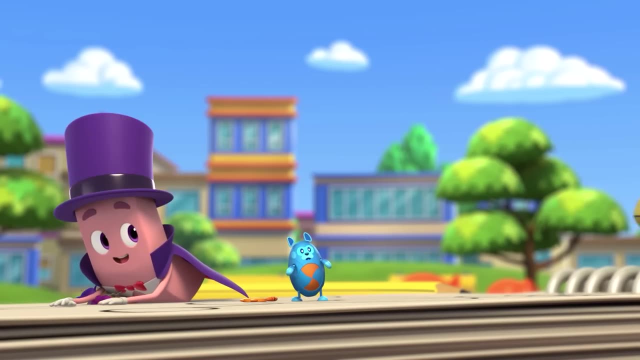 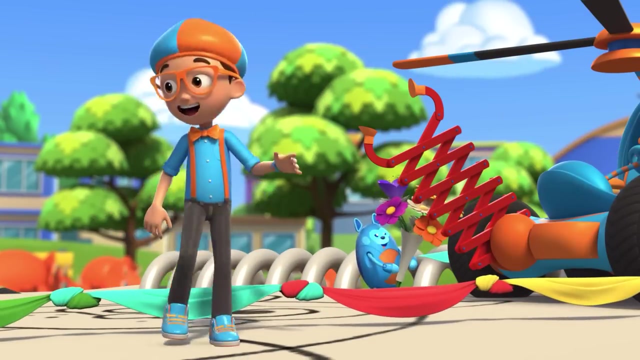 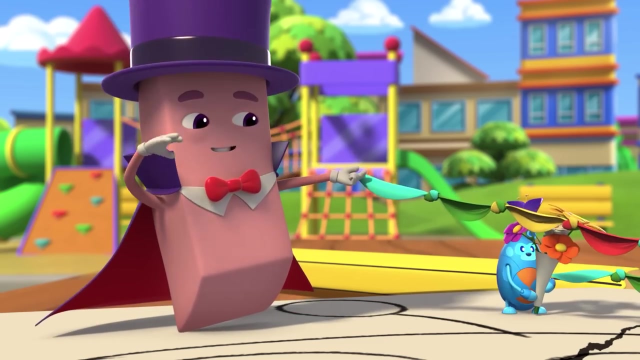 Whoa, Whoa. Oh no, I got it. Phew, That was close, Sorry about that. Whoa, Hey, Ernie, can you erase this graphite mark? Oh, what a great idea. I will make that mark disappear by erasing it. 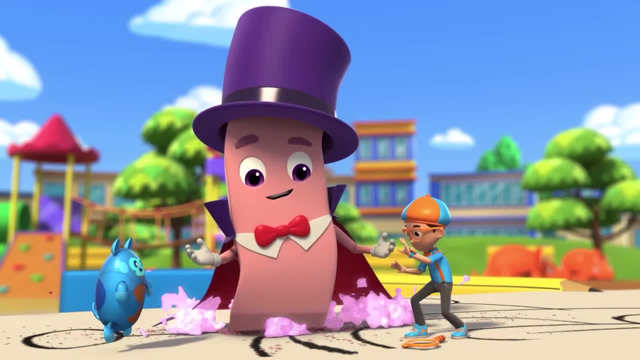 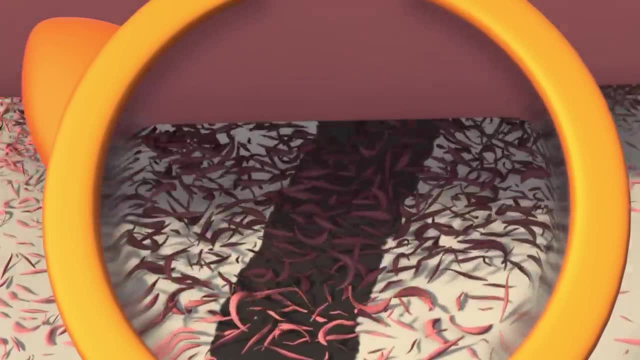 When an eraser like me rubs against the paper, it creates friction and heat. Awesome, The heat makes the eraser move. The eraser is stickier than the paper, So the graphite comes loose from the paper and sticks to the eraser instead. 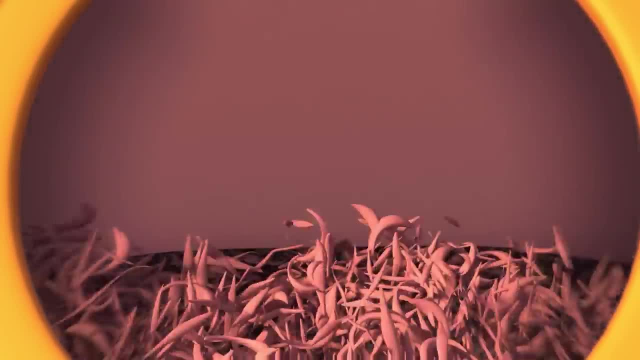 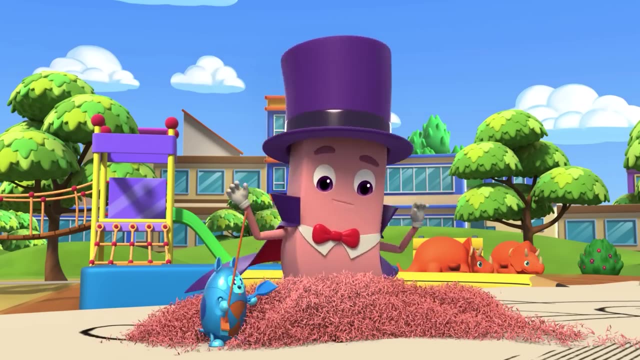 Friction also causes the eraser to disintegrate or fall apart. See the small bits coming off. You've got a few on you, Oh, they're cute. Rub the eraser on the paper and up, And boy oh boy, the graphite comes off. 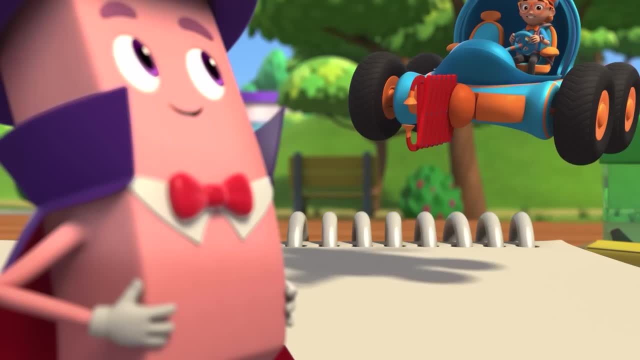 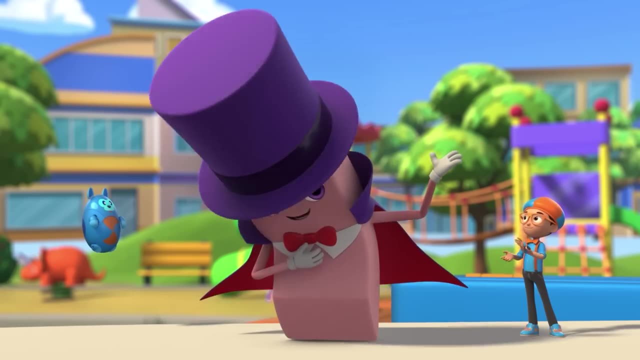 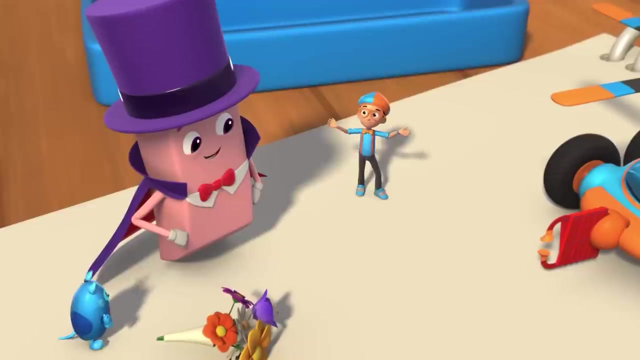 Ta-da, My disappearing act. Oh, that's amazing. Was it magic? No, it's science. Cool, And I got the answer to my question: How does an eraser work? Erasers work by using friction to make them stickier than paper. 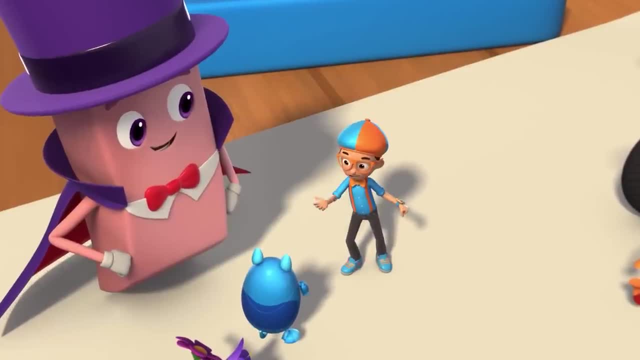 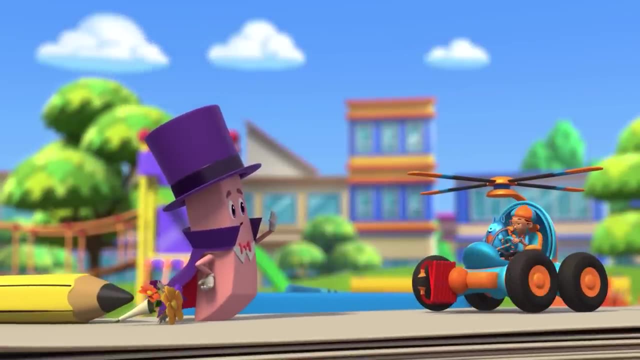 So the graphite on the paper clings to the eraser. Upload answer, Deebo. Thanks for the magic show, Ernie. Now it's time for us to disappear. Goodbye, Blippi. It was magic to meet you. 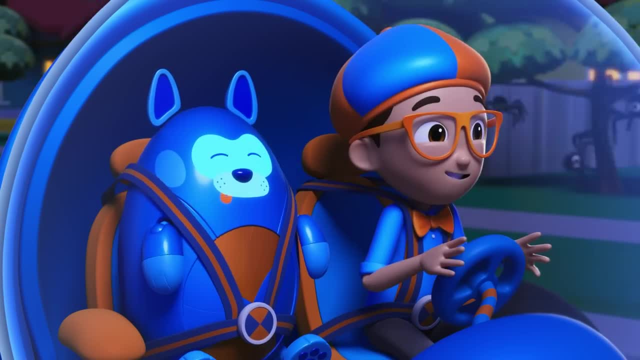 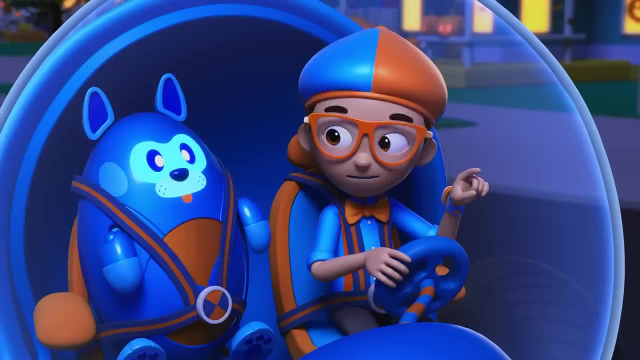 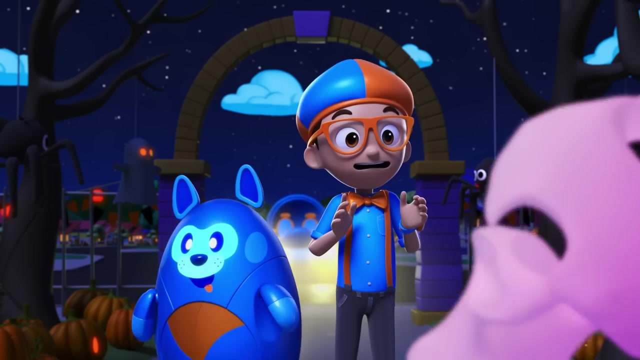 Me too. I love looking at spooky houses decorated for Halloween. Wow, look at all the jack-o'-lanterns. Let's go check it out. Hi, Blippi, Yikes, Oh, Hello, Mr Pops. 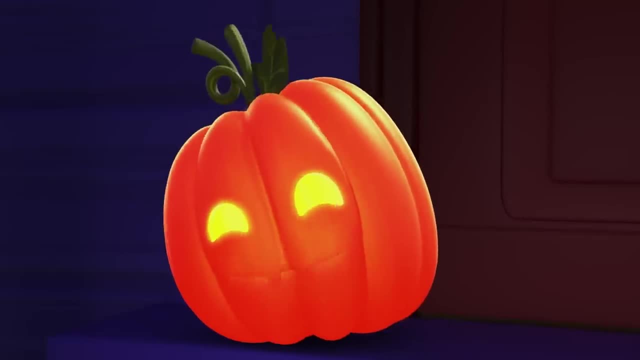 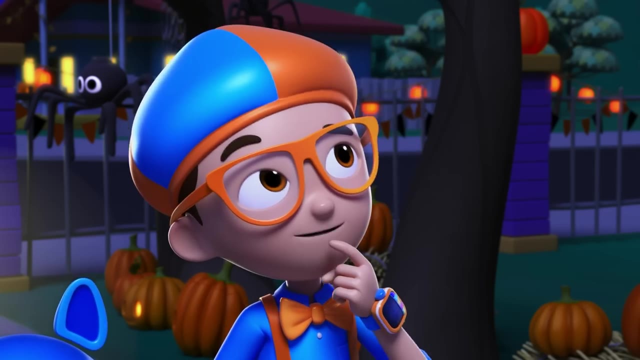 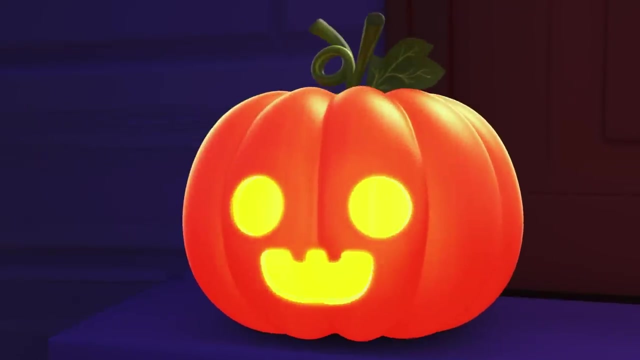 Mr Pumpkin, you scared me. You're welcome, Blippi. I love to be scared. It's fun, It is. Hmm, I wonder: is it really fun to be scared? Only one way to find out: Let's have a scare contest. 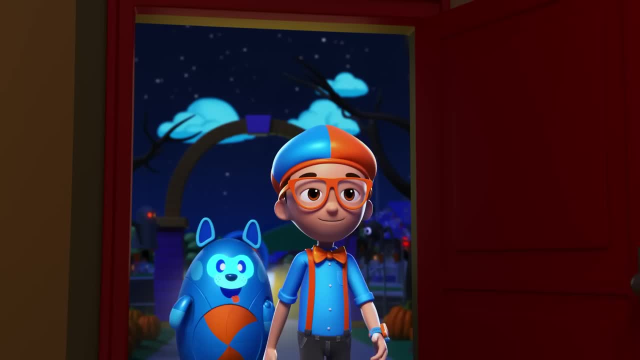 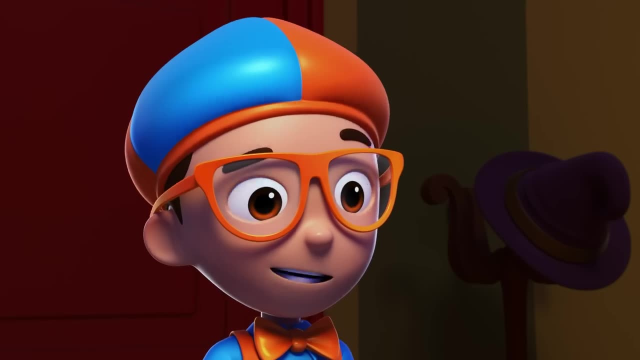 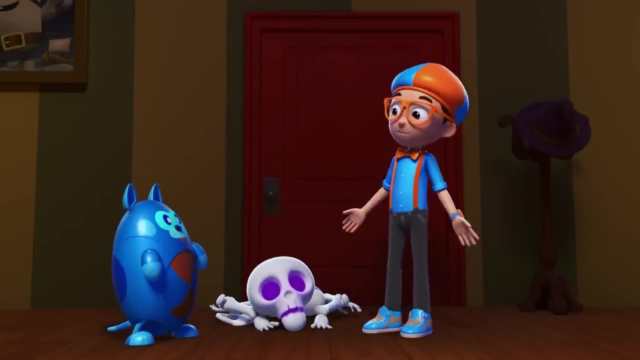 Hmm, okay, Let's do it. Yikes, Score one for Team Pumpkin Team. I don't see anyone else. Uh, yikes, Oh, hi, again Bones. That's two points for Team Pumpkin. Come on, Bones. 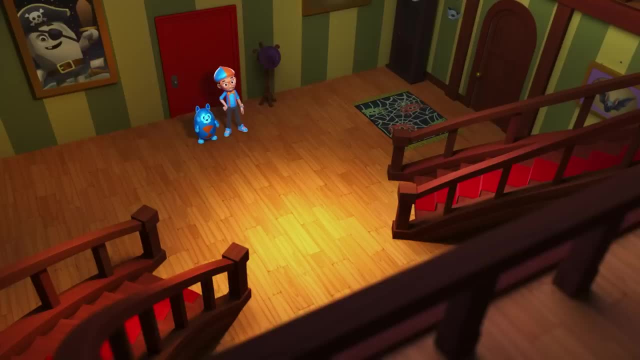 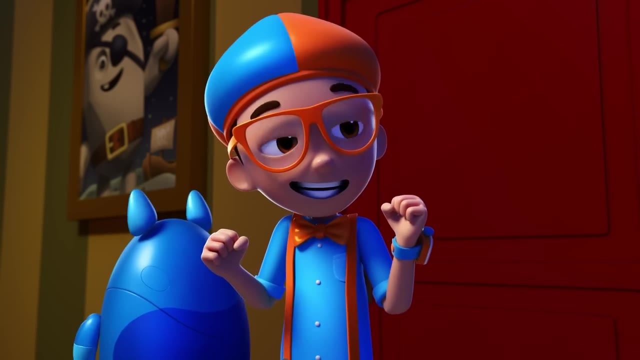 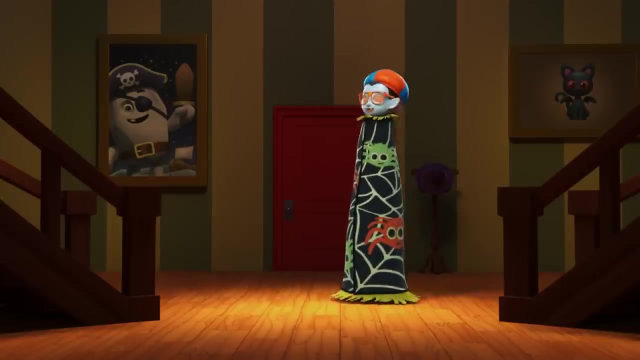 Let's plan our next scare. Hmm, we have to come up with a good scare. Deebo, What can we do? I have an idea: I'll wear this mask and stand on your shoulders while you Howl. Let's go. 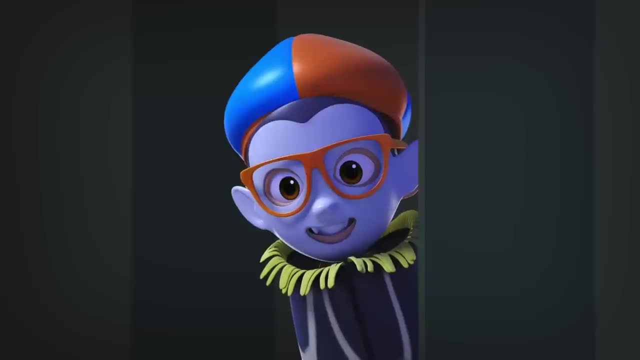 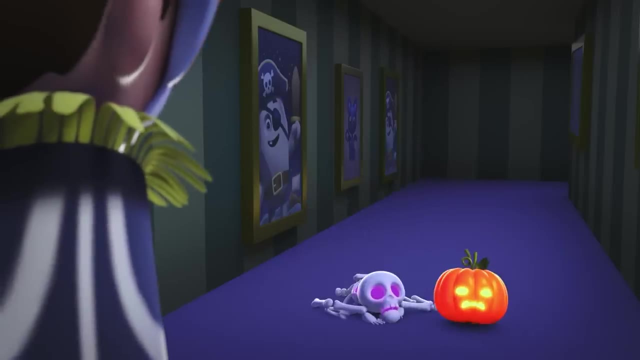 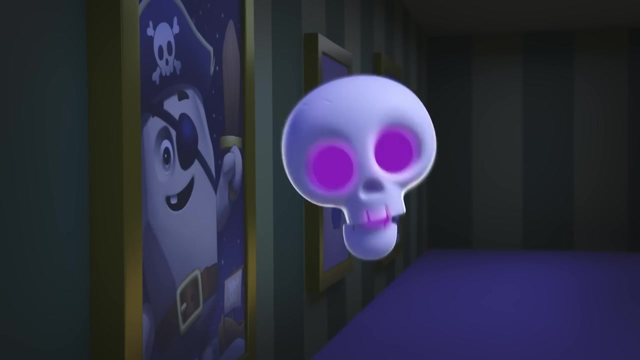 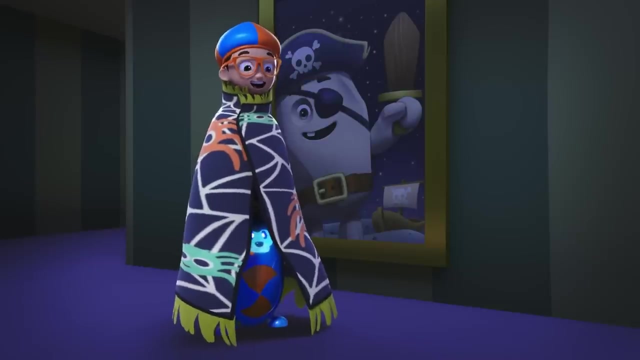 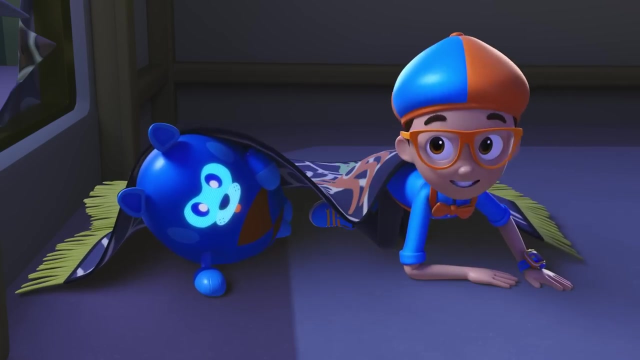 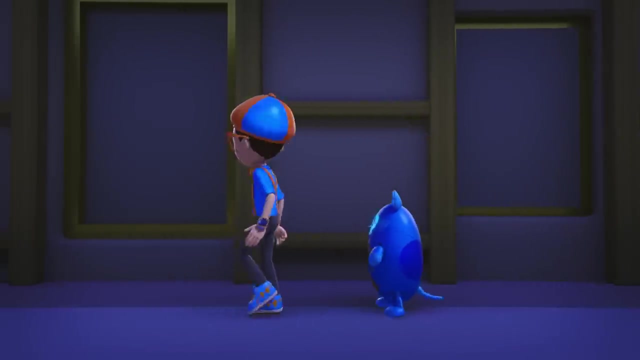 This is gonna be good. Ooh Ah, Score one for Team Blippi. You got us good, Blippi, Yeah, Nice work. Deebo, Whoa, Whoa Cool. A secret hallway, Hmm, Oh boy, this is really going to scare them. 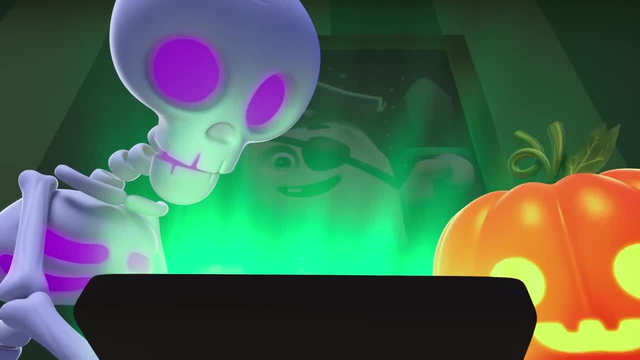 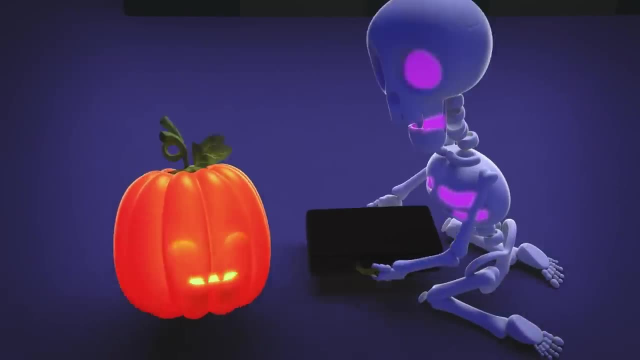 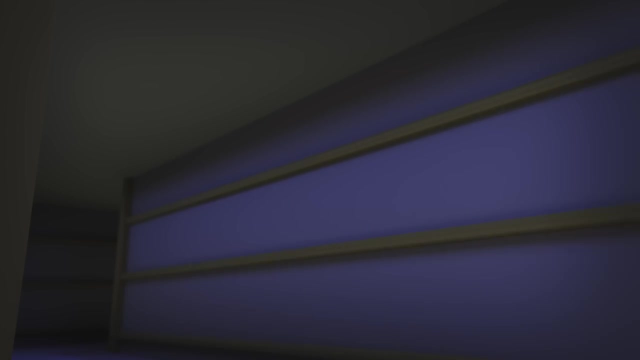 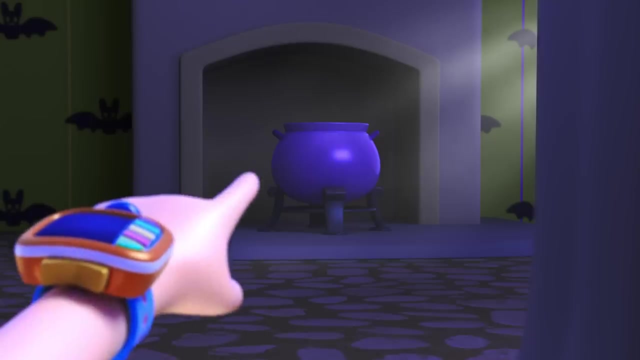 Hee, hee, hee, Shhh, Boo, Whoa. Oh, That's two points for Team Blippi. The next team to score a point is the winner. Yeah, Hold on, Deebo. I have an idea. Let's hide in that cauldron and jump out and scare Mr Pumpkin and Bones. 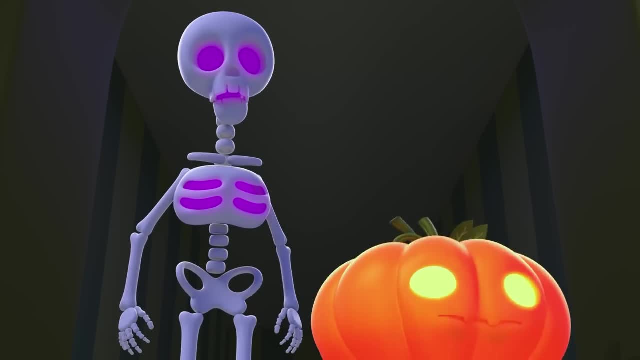 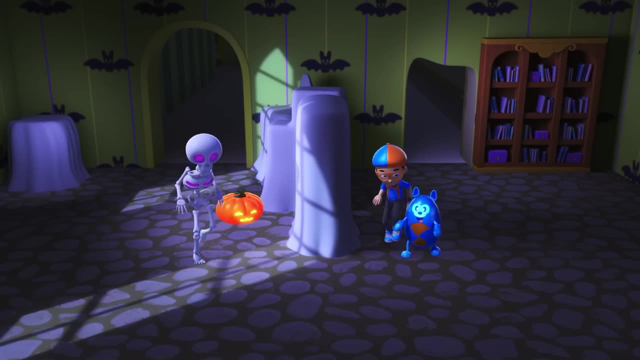 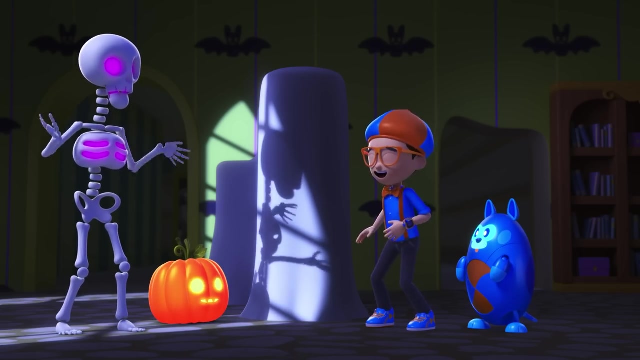 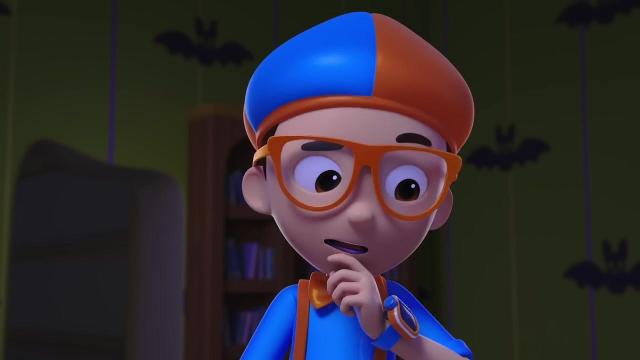 Hey, Bones, Let's hide in that cauldron and jump out to scare Blippi and Deebo. Ha ha ha ha. Mmm, I guess it's a tie. Ha ha ha. All right, Halloween is the best, But I still don't know the answer to my question. 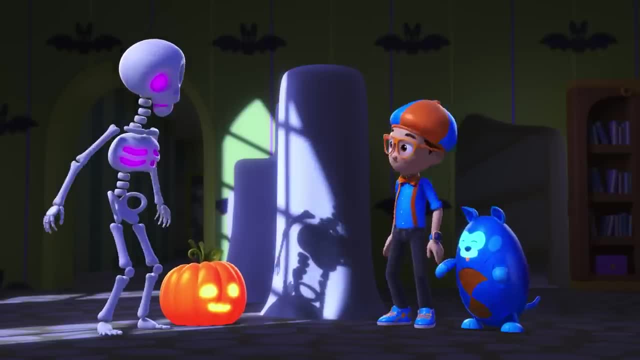 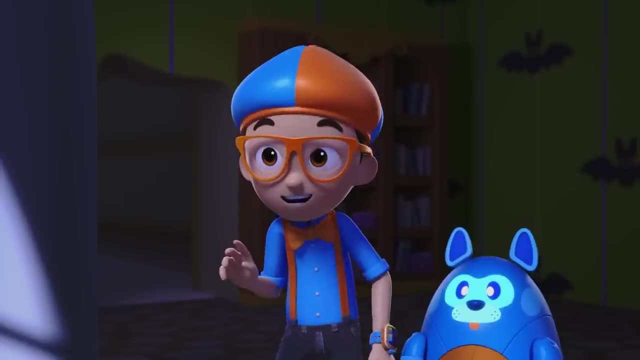 Is it really fun to be scared? Ha ha ha, Yeah, All right, Upload answer, Deebo. Ha ha ha. Thanks for an awesome scared contest, Mr Blippi. Ha ha ha, Yeah. Yay, Mr Pumpkin, I had a lot of fun. 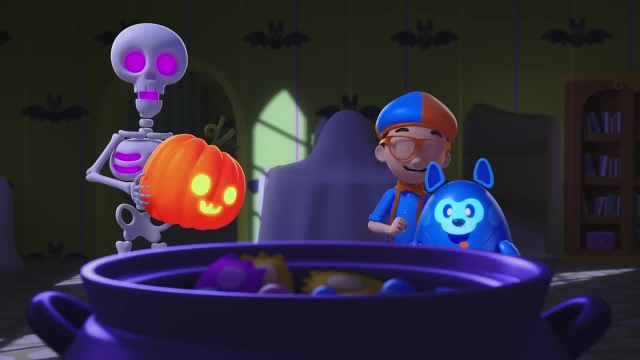 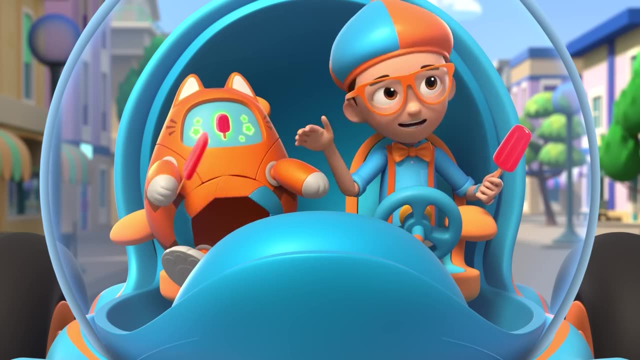 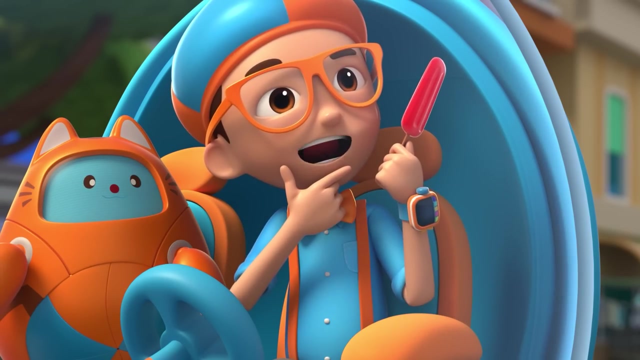 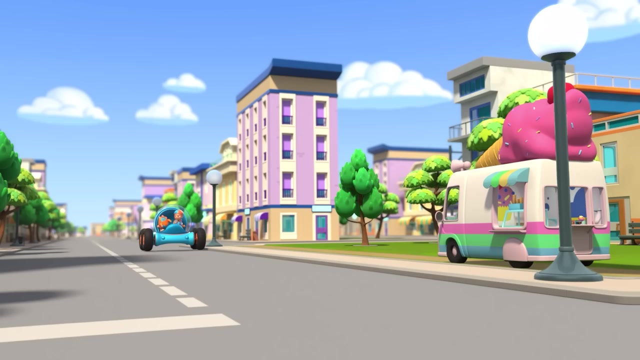 No problem, Blippi, I had a lot of fun too. It's so hot out today, but my popsicle is melting down my hand. Hmm, I wonder, why do popsicles melt down my hand? What's that Tabs? Go into that ice cream truck and ask an expert. 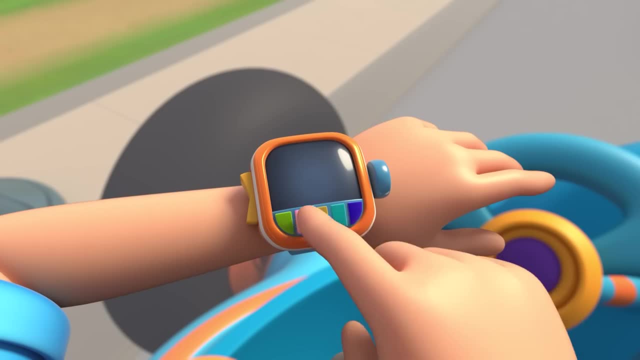 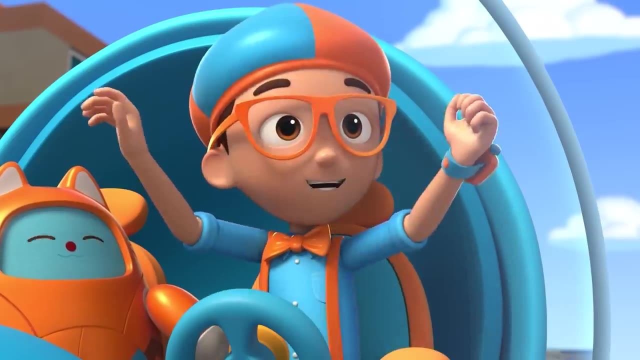 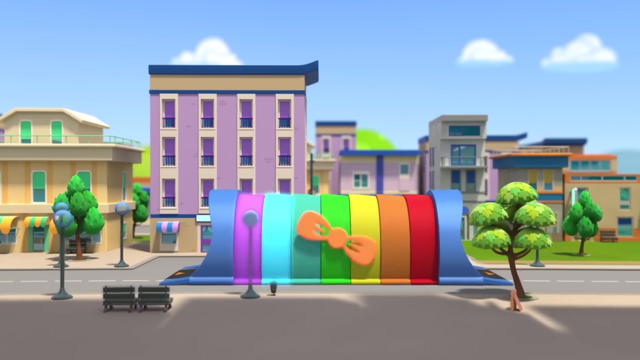 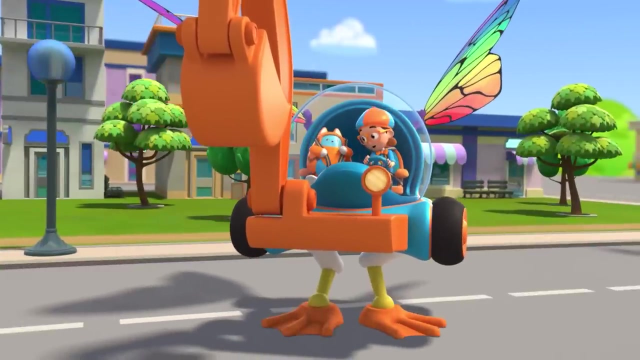 That's a great idea. I'm gonna need wings, the excavator arm and duck feet. Wings, excavator arm, duck feet- confirmed. Activate Blippi Station. The Blippi-mobile is ready for adventure. Let's go find out why my popsicle always melts down my hand. 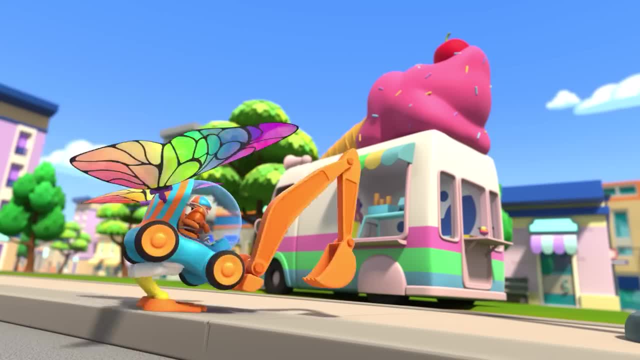 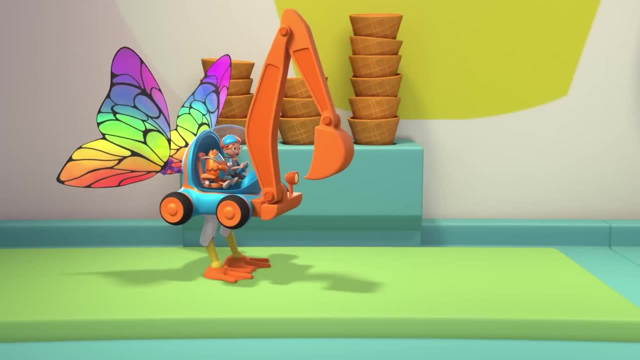 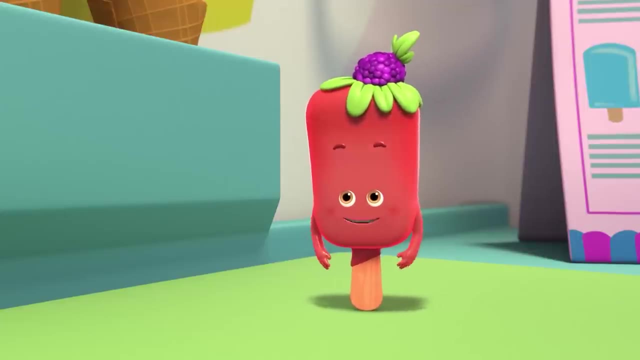 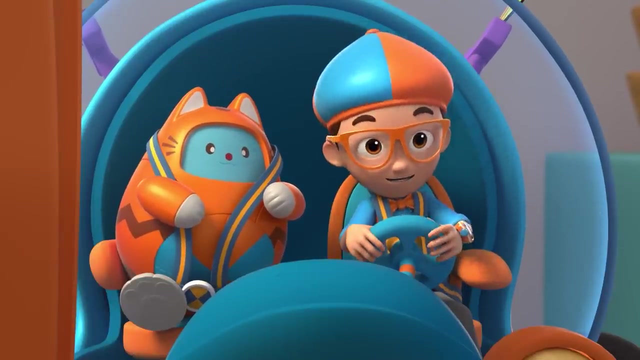 Shrinking down. Woohoo, I'm in the ice cream truck. Hi, Welcome to my neighborhood. I'm Sherry Pop. Glad you popped in. Hi, Sherry, It's me Blippi. I was wondering why my popsicle always melts down my hand. 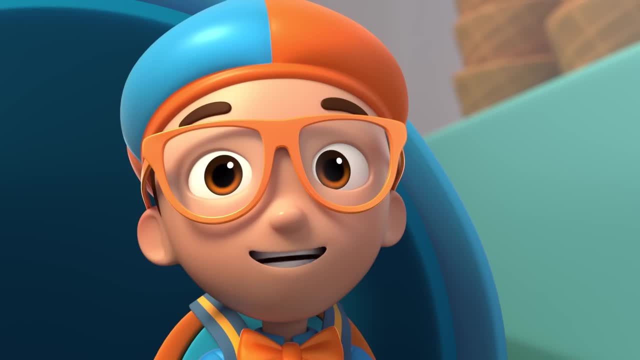 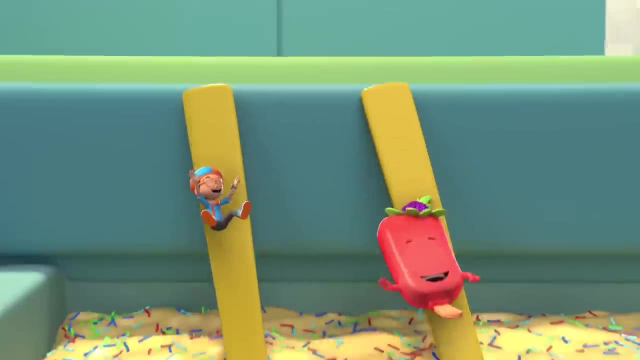 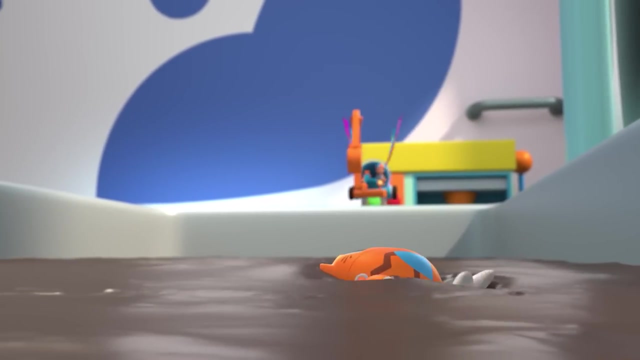 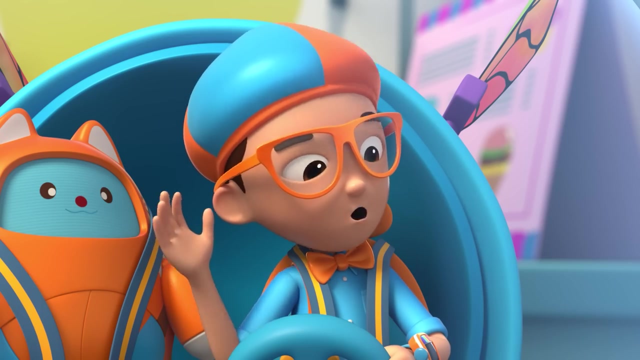 Oh, I know that one. But first let's have some frozen fun. Alright, Woohoo, We're ice cream boarding. Woohoo, We're sprinkle sliding. I'm chocolate fudge snorkeling. Sherry, are you melting? 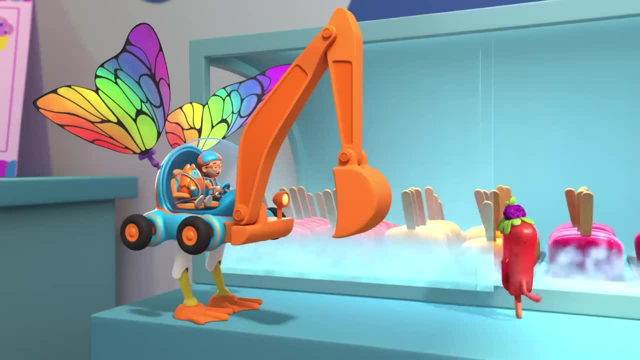 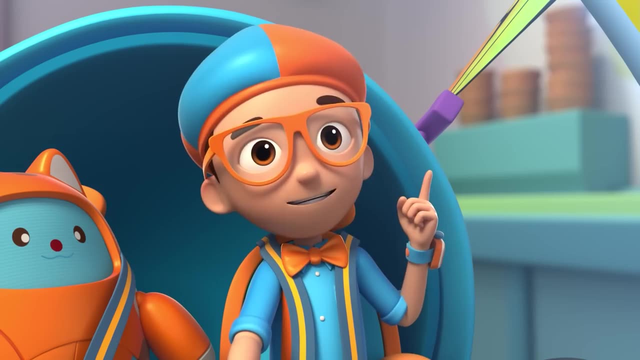 Yes, I'm melting because I'm very warm, But I'll go cool off in the freezer and I'll be fine in a sec. Mmm ice cold. How's it going in there, Sherry? It's freezy breezy. Now I'm all set. 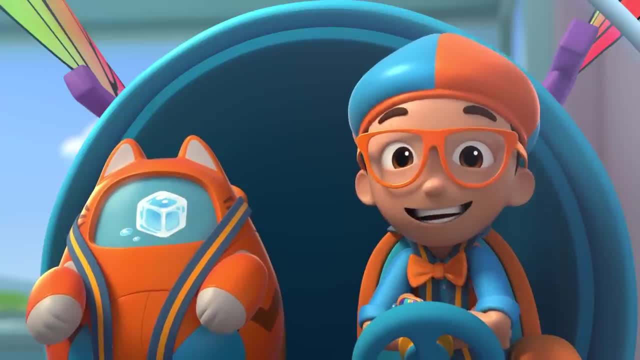 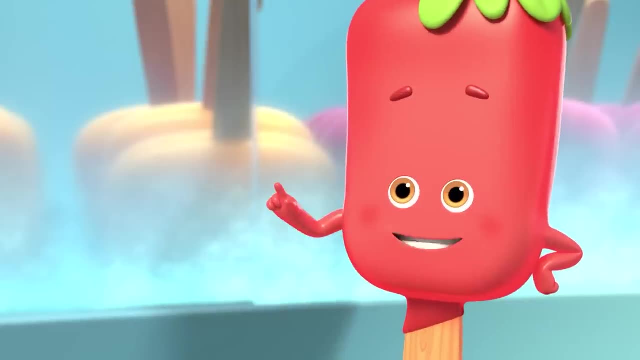 Whoa, It looks super freezing in there. Yup, It's cool to be cold when you're a frozen dessert like me. My ideal temperature is 32 degrees Fahrenheit, 0 degrees Celsius. If I keep cool like that then I won't melt. 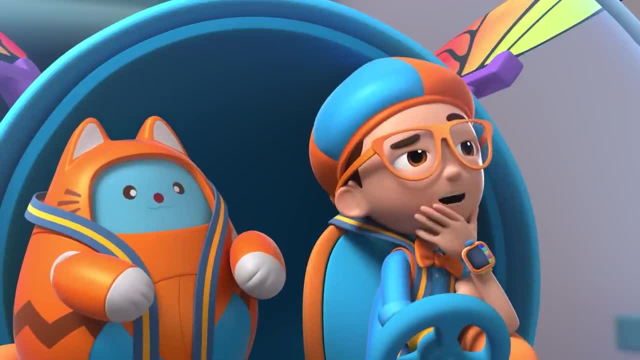 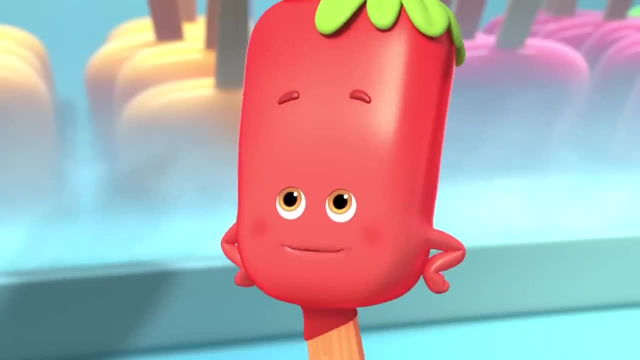 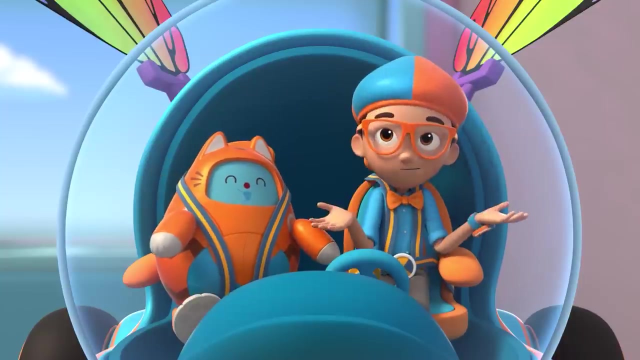 Good to know. I see you're like my popsicle from earlier, When it was out of the freezer and in the heat of the Blippi-mobile it melted off. Sounds like your popsicle should've come for a visit, You're right, Which means we have the answer to my question why my popsicle melts down in my hand. 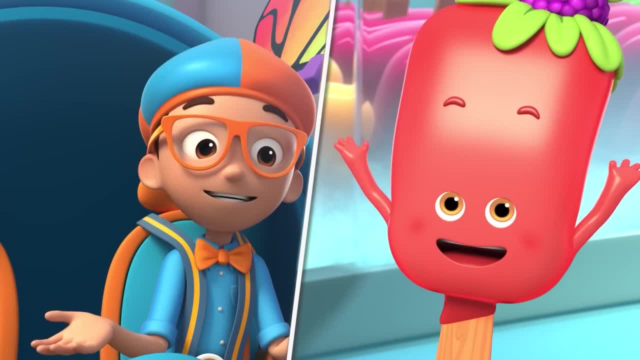 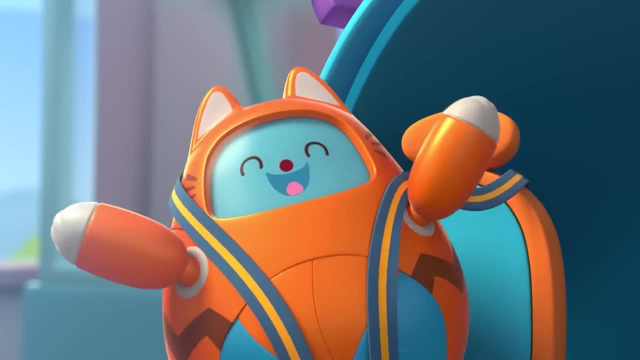 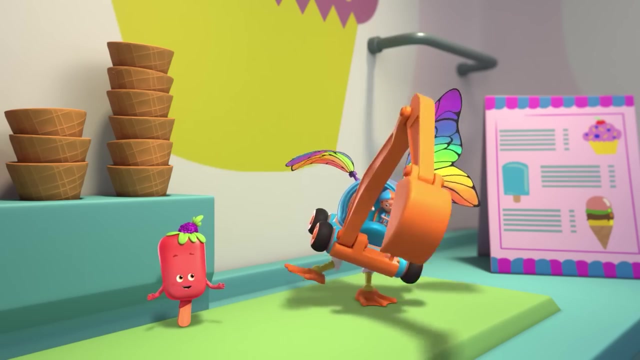 It's because popsicles will melt if they get too warm. That's why we keep them in the freezer. Upload answer tabs. Sherry, thank you for a totally tasty adventure. It was so cool. Stay cool, Blippi Buh-bye. 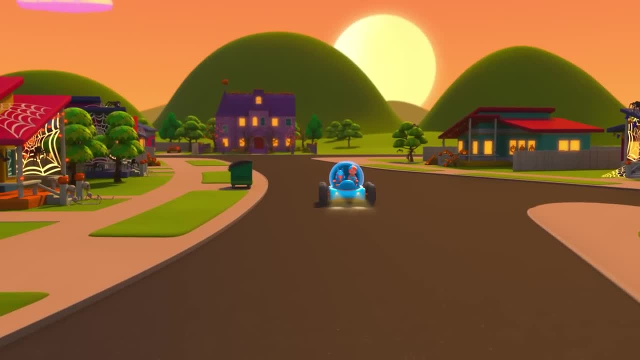 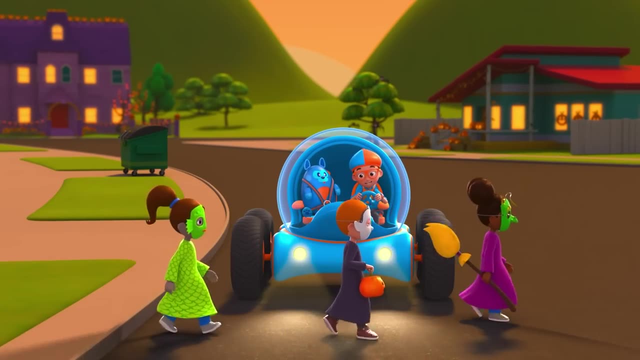 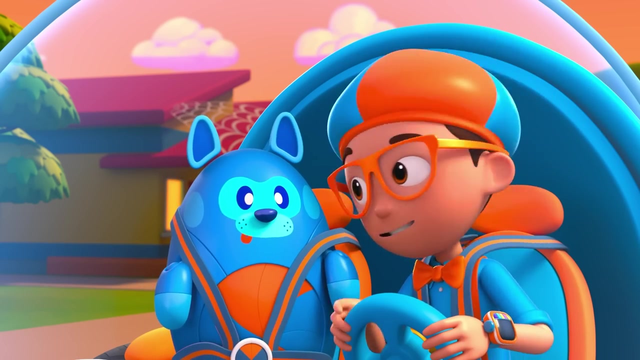 Clearly an ice cold, ice проб. How nice weren't they. But don't worry, Deebo, Those aren't real monsters – they're trick-or-treaters. Because it's Halloween. Of course, Deebo, I can teach you how to trick-or-treat. 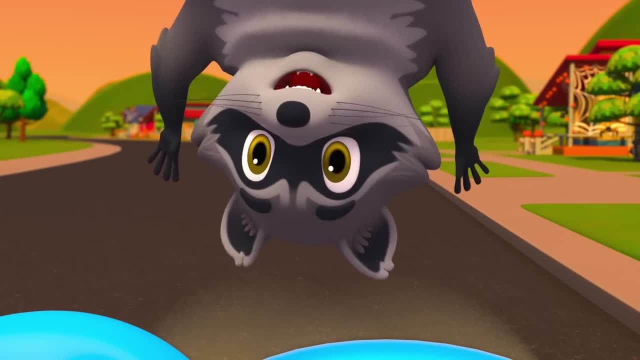 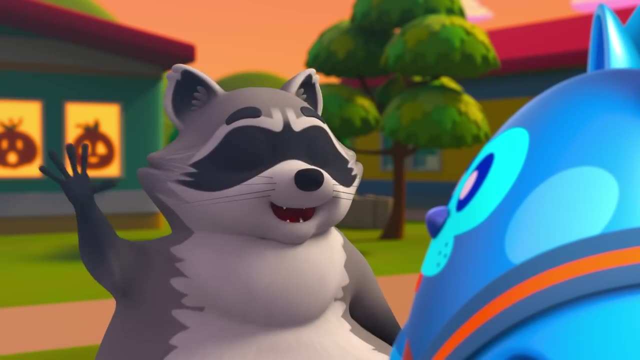 Did somebody say trick-or-treat Yours, Dax? Really, Holla Hi Rita. This is my friend Deebo Hi Deebo. I'm Rita the Raccoon, and Halloween is my favorite holiday Because of all the costumes. 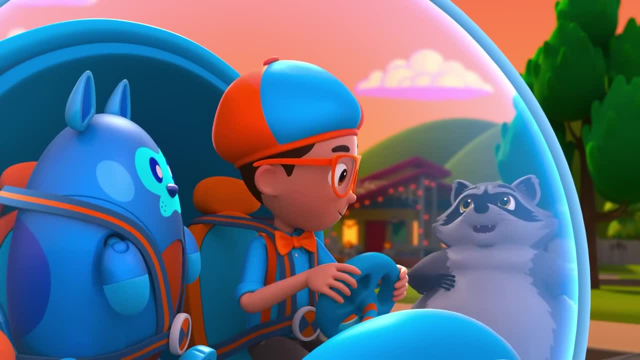 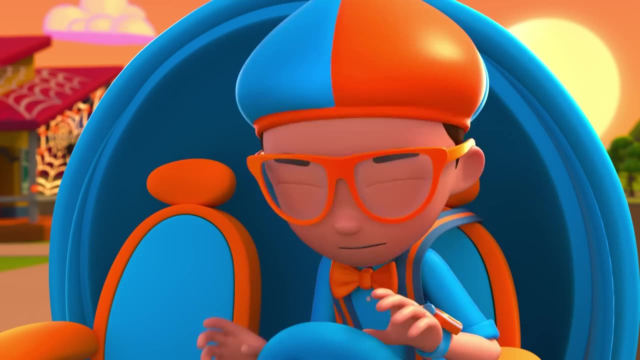 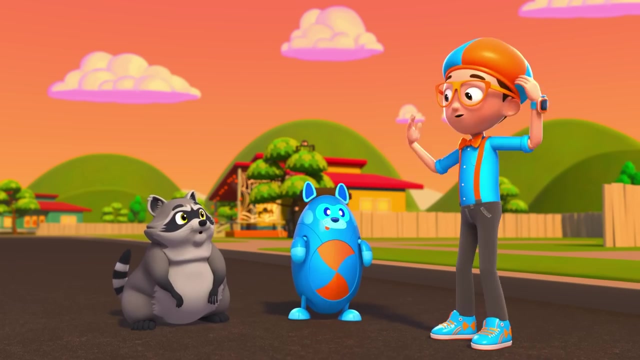 No silly, All the free food. Ha Well, you're just in time, because Deebo and I are about to go trick-or-treating. Wait, Deebo, We still need a few things before we go. The first thing we'll need are costumes. 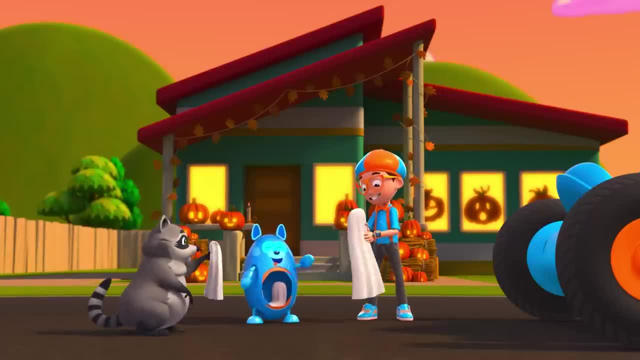 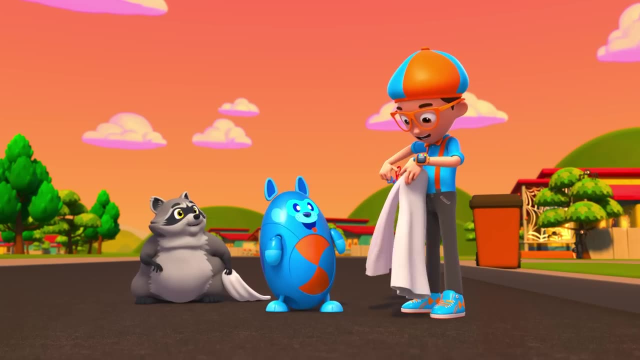 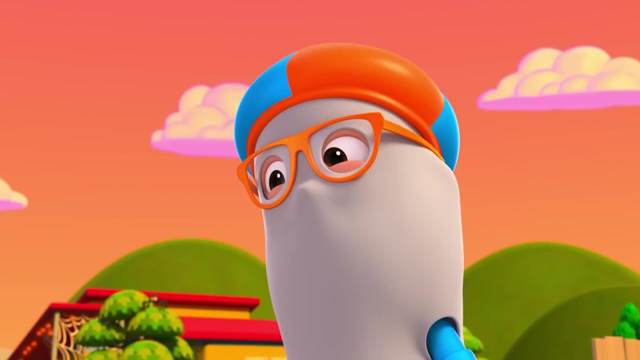 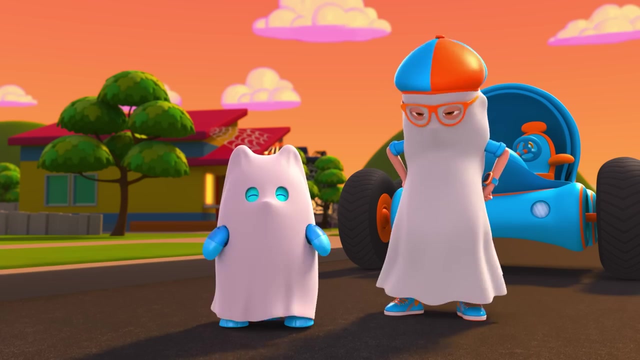 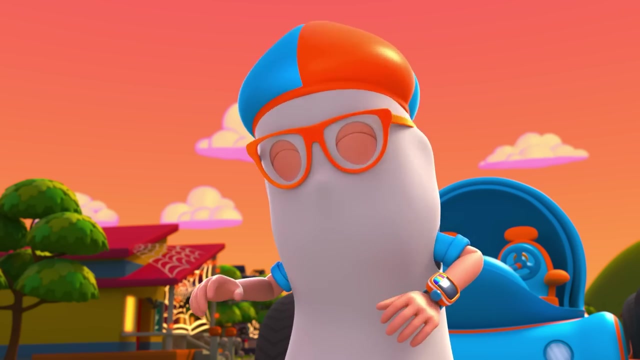 Great idea. We'll be ghosts- So fun. Even ghosts need to be able to see. There we go. I'm a Blippi Ghost, Whoa. We've got a Karate Master trick-or-treating with us Enough, And now a chef- So cool. 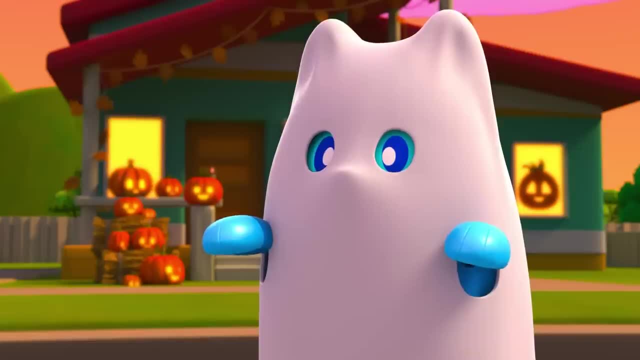 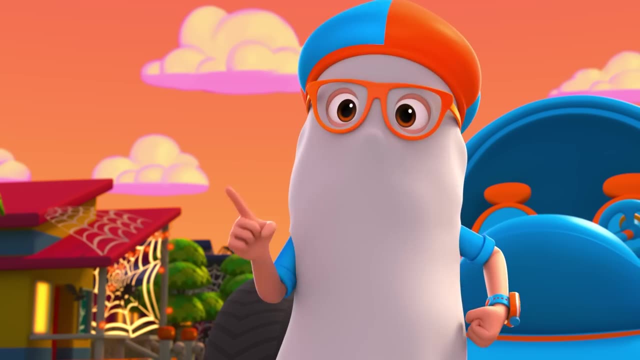 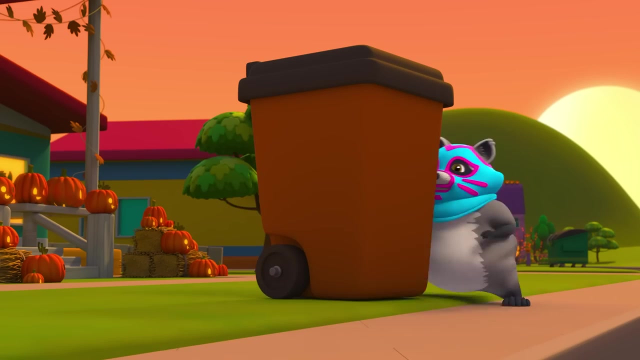 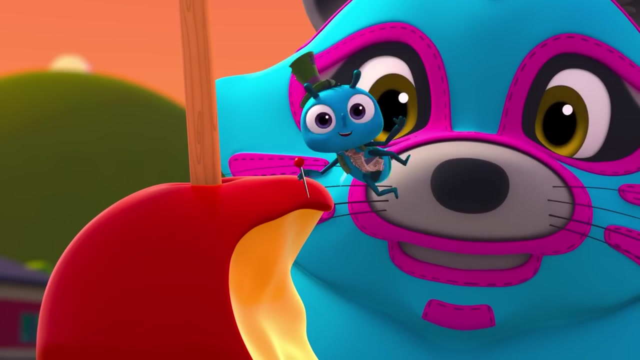 Boo, I'll just stick with the mask. Our costumes are ready. Time for the next step: Containers to hold our treats. Cool Jack-o'-lantern pails, Yeah. Trash bag, Ooh, My first treat. Now it's time to hit the streets. 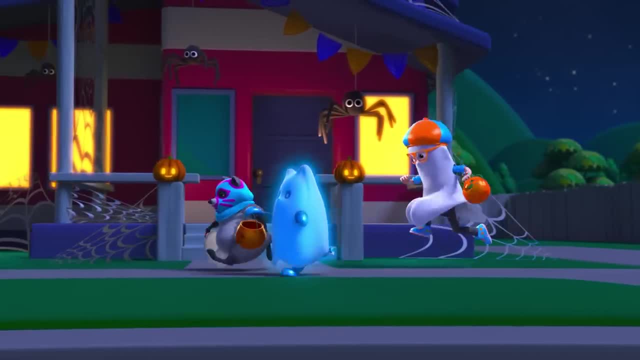 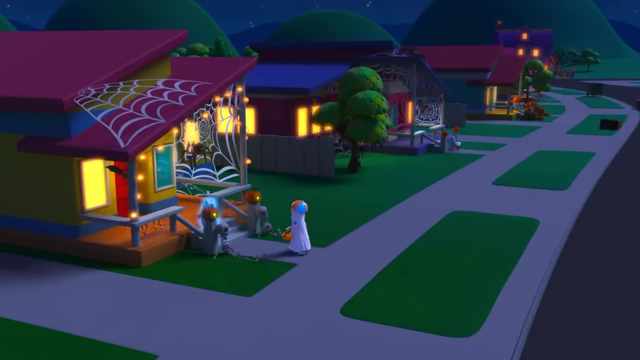 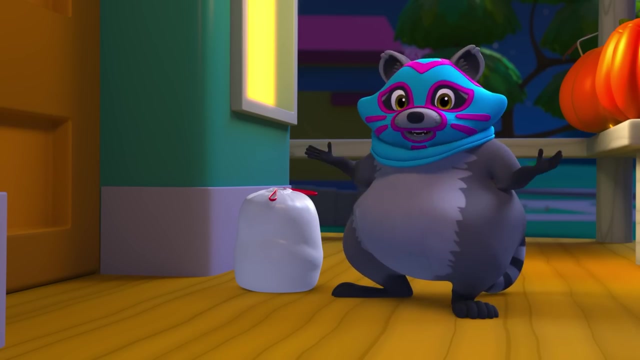 It's getting dark, A glowing ghost Fun. Okay, Be sure to pick a house that is decorated and lit up for Halloween. Then knock on the door and say: Trick-or-treat. Come on, What are you waiting for, Trick-or-treat. 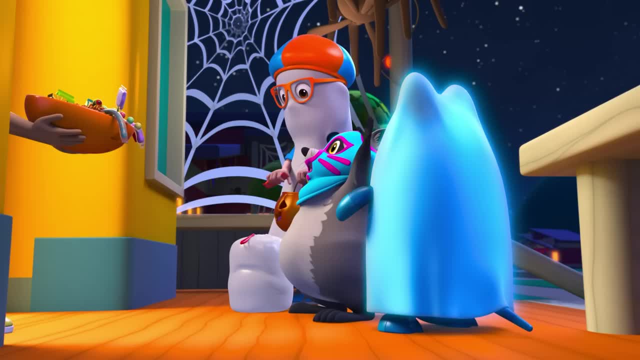 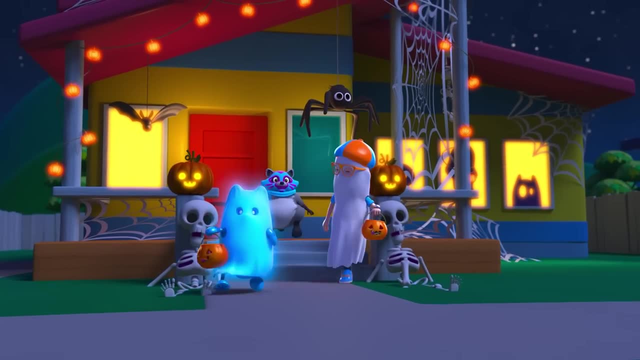 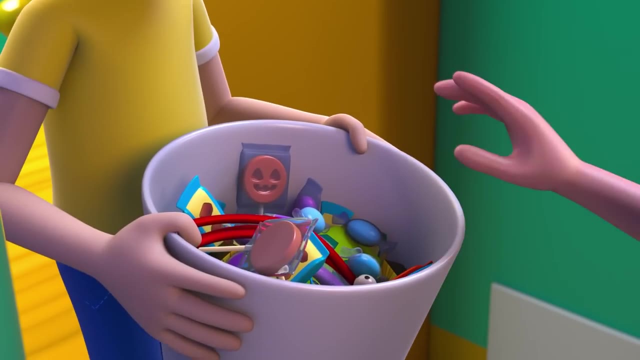 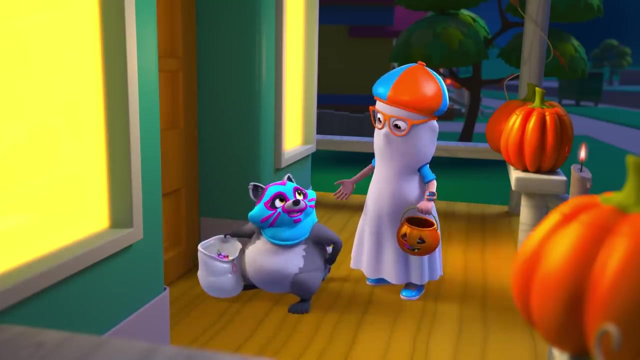 Trick-or-treat. Thank you, Happy Halloween. What Shoot, Remember. you can only go to each house one time and just take one piece of candy. Trick-or-treat, Ha-ha Jackpot, That'll last you till next Halloween.